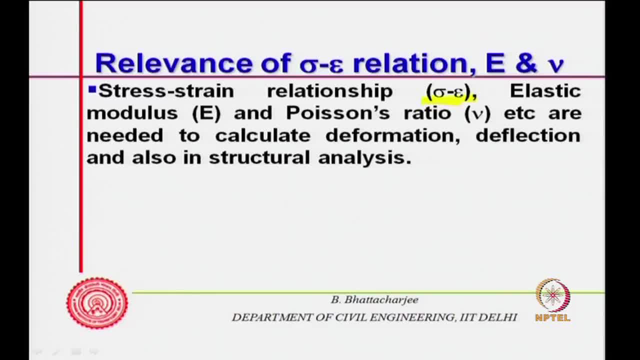 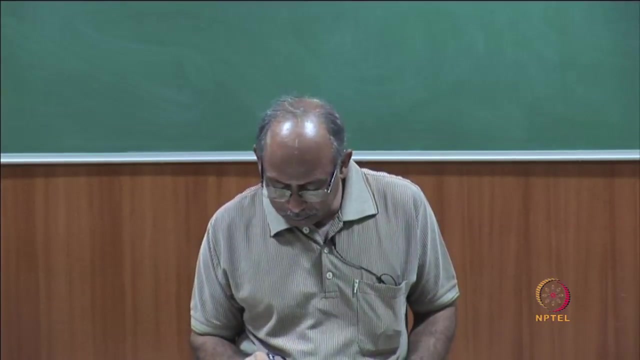 Stress strain relationship. you know, sigma i is how we denote stress and epsilon. Elastic modulus and Poisson's ratio are needed to calculate deformation, deflection and, you know, necessary to determine also forces sometime in indeterminate structures. So structural analysis would need this modulus of elasticity particularly, and deflection etcetera are dependent. 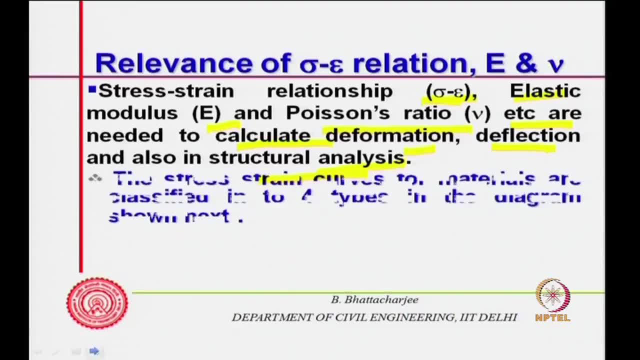 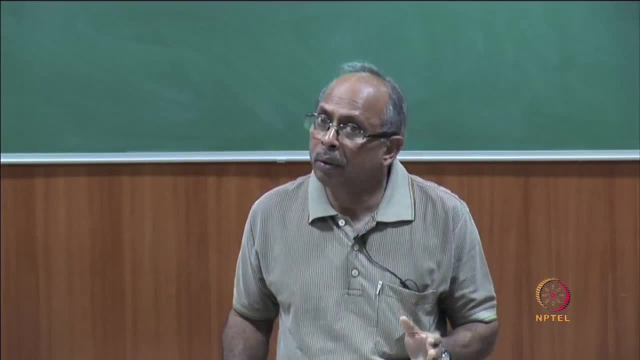 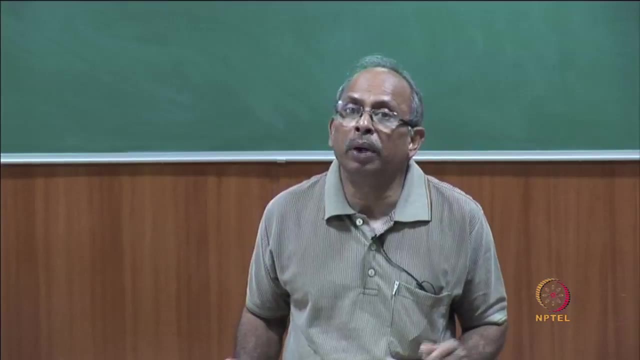 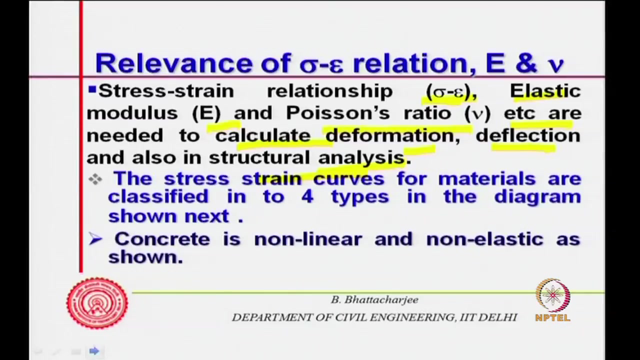 on all this. So these properties are relevant and the stress strain curves for materials is important because in structural design you know they have their relevance. Now, stress strain curves of materials: we can classify into four types for all materials in general. Of course we have left out elastomers, but typically these are the four, So we will. 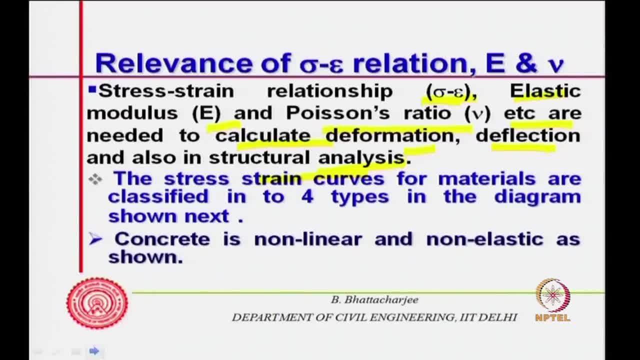 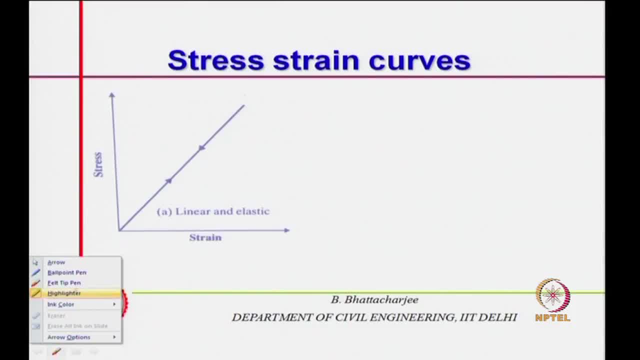 see that concrete is, of course, non-linear and inelastic or non-elastic material. So simple: linear and elastic material. linear and elastic material, strain versus stress. So it will follow this stress strain curve during loading and when you unload it. it. 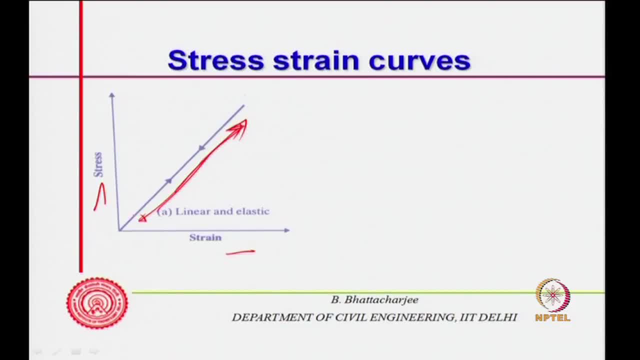 comes back just back to the original, with no residual strain remaining. This is non-linear and elastic. So an elastic material will come back to its original state, So this state when load is withdrawn. but this is not linear, It is non-linear. And if we follow, 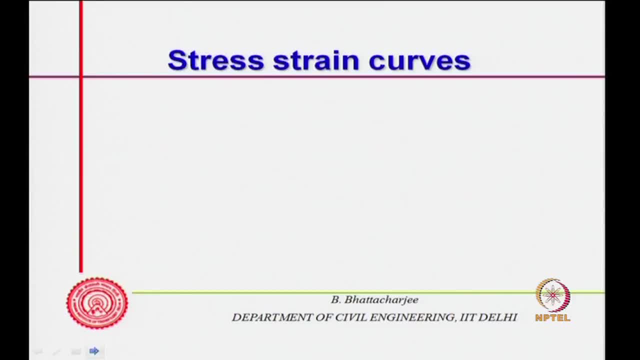 it up further. this of course linear, but inelastic or non-elastic, You know it does not comeback. So there is a residual permanent strain And this is non-linear and non-elastic. So there is permanent strain. it goes like this: at some level of stress you go, and when? 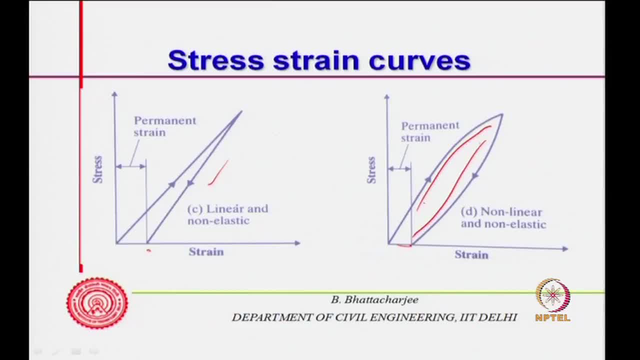 you come back, It does not come back And this is non-linear and non-elastic. So here it does not close in. So there is some kind of a hysteresis and it is non-linear, non-elastic. 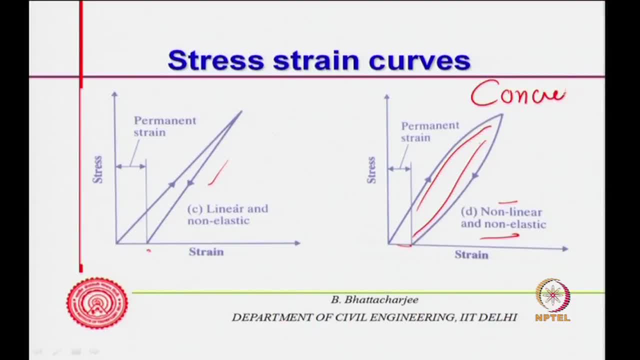 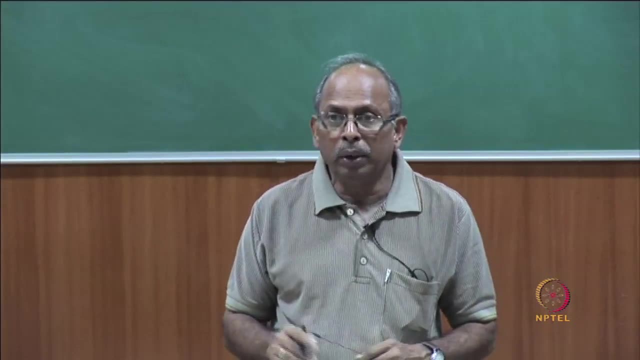 and concrete belongs to this. So concrete belongs to this material. Concrete, cement paste or similar material, they belong to this. So it is actually non-linear as well as inelastic. So when you release load beyond of course, certain point, not right. 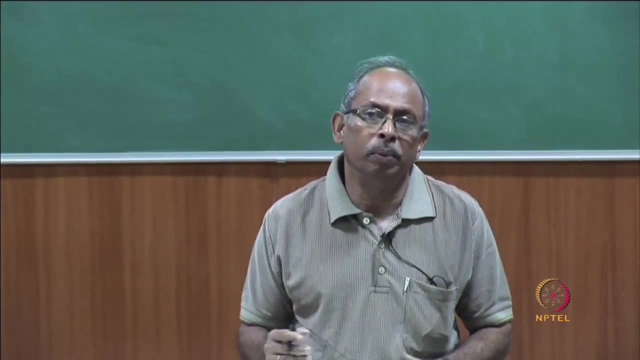 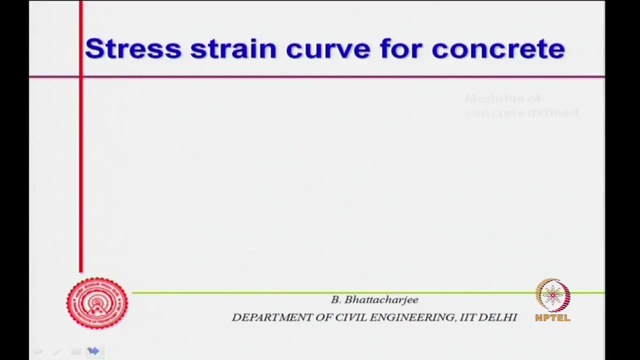 in the beginning, at least one-third load. if you go on beyond that, there will be some permanent strain when you release the load. Well, since it is non-linear, we have to define the modulus of concrete since non-linear. So its behavior is something like this and: 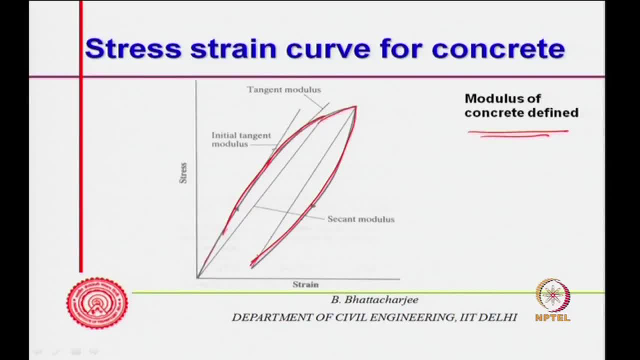 then it follows something like this: So what you do, You define something called initial tangent modulus, initial tangent modulus. you know this is what it is. So the tangent if you draw here that is we call it, We call as initial tangent modulus. but I can draw tangent anywhere that is called tangent. 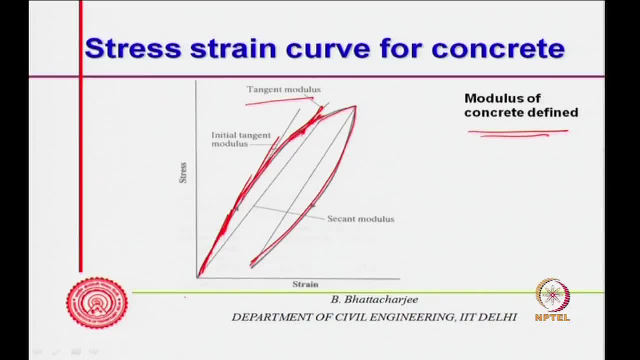 modulus at that particular load. but I can join the origin with this point and I get another modulus, the slope of this line, and that we call as second modulus. and while returning I can also calculate out the same second modulus from this point, the slope of this line. So 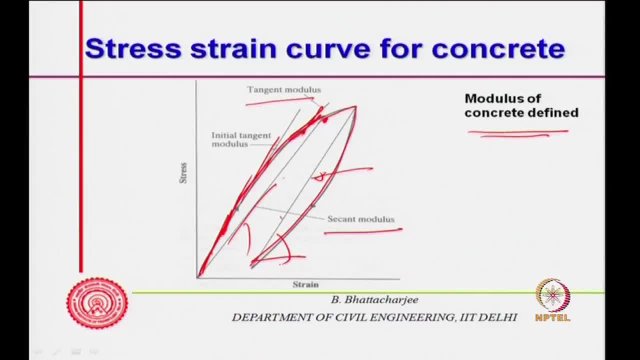 for concrete modulus can be defined in different way: Initial tangent modulus, tangent modulus at any stress or strain level, and second modulus, again at any stress or strain level. In fact, we can have a chord modulus joining between two points. You can have a chord modulus, So chord modulus, So joining between two. 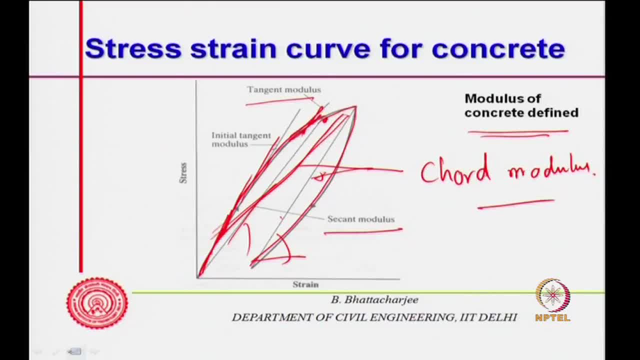 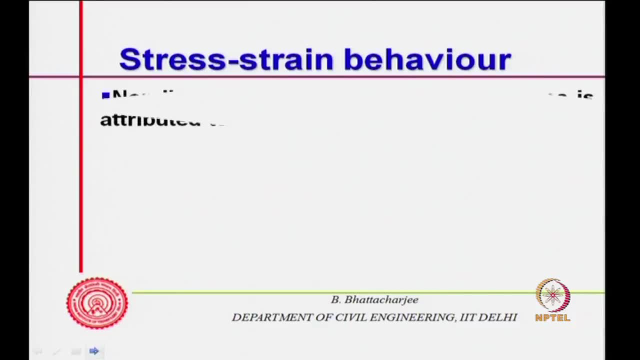 points is also called chord modulus. So here we define the elastic modulus. for concrete, Now, if you look at stress-strain behavior, it is non-linear. That is what we have shown, and this is attributed to something called creep, that is, the deformation under sustained 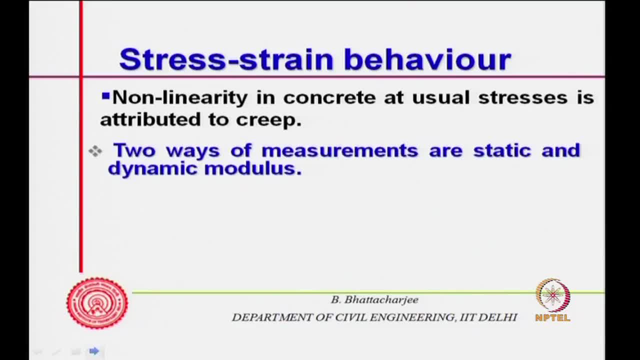 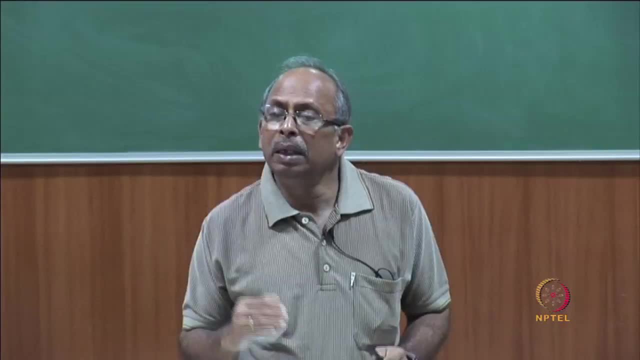 loading. We will come to that sometime. This one way of looking at it, but there is something more we will look into. So we can measure this under static condition. another is under dynamic condition. that means static condition means you apply the load monotonically, in steps, and then see how the deformation or strain changes. So stress. 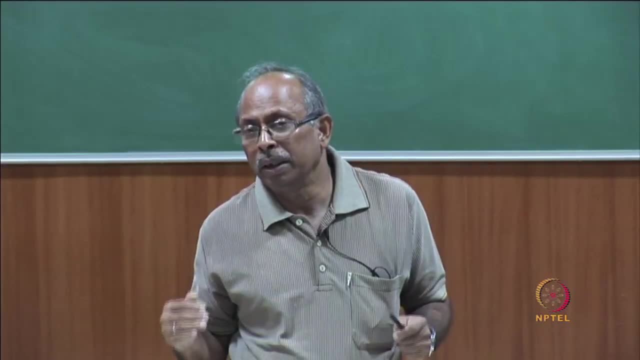 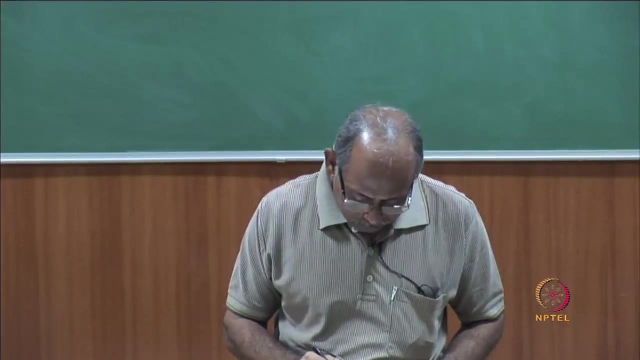 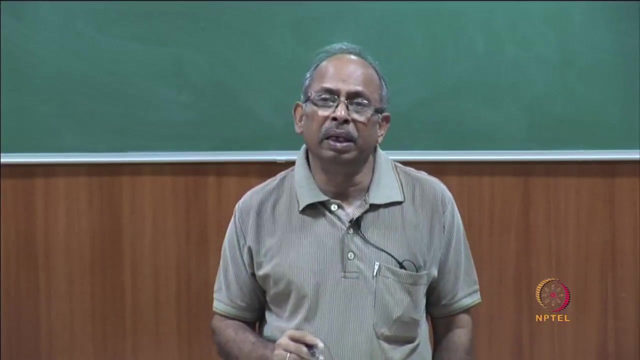 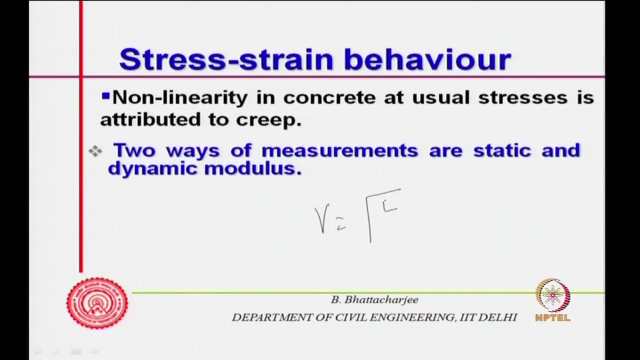 at steps and strain at measure, corresponding stress, and from stress strain curve you can find out the modulus of elasticity. But you see, from, you know concepts of mechanical wave travelling in solid media. we know the velocity in the media is a function of. velocity in the media is function of e. you know it is a function of e root e over rho. 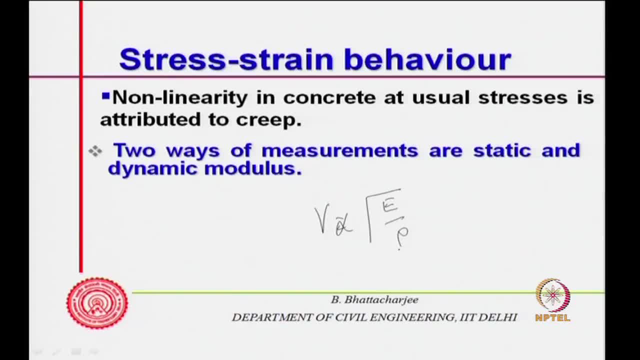 actually, you know So, for velocity is proportional to e over rho. So therefore, modulus of elasticity has something to do with this velocity, something to do with the mechanical wave or sonic velocities, pulse velocities. So when wave is travelling through the solid, you know, there is a compression and rarefaction longitudinal. 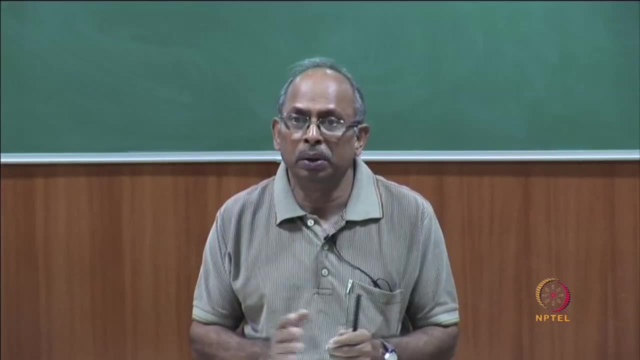 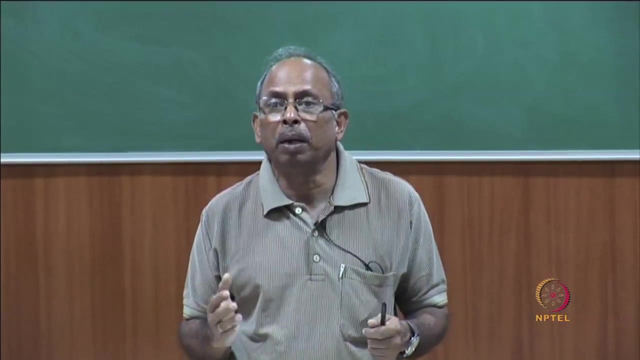 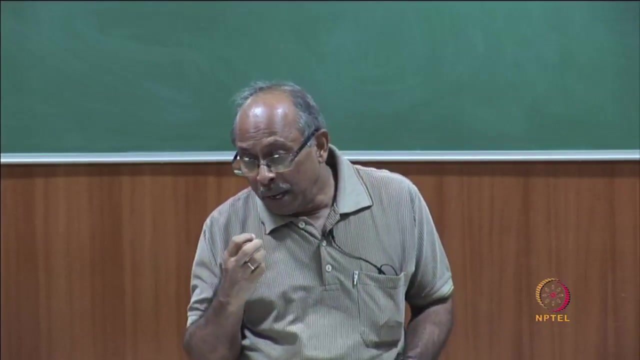 wave travelling through it, or any wave travelling through it, there are deformation and therefore the modulus of elasticity plays a role. But what kind of modulus of elasticity? that would be bulk modulus. So you can relate these two anyway this: can you relate this to velocity? So if you have actually obtained velocity of wave travelling through, 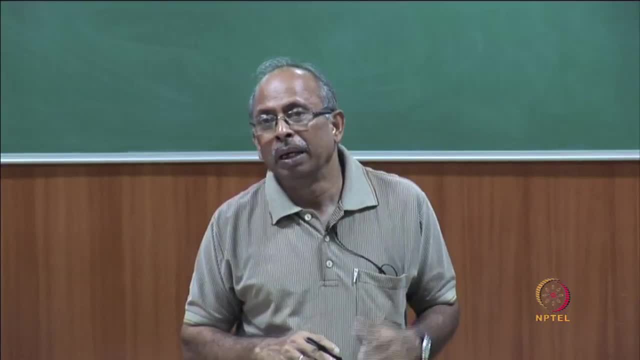 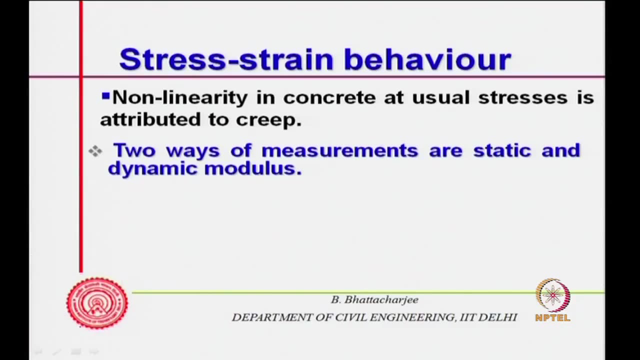 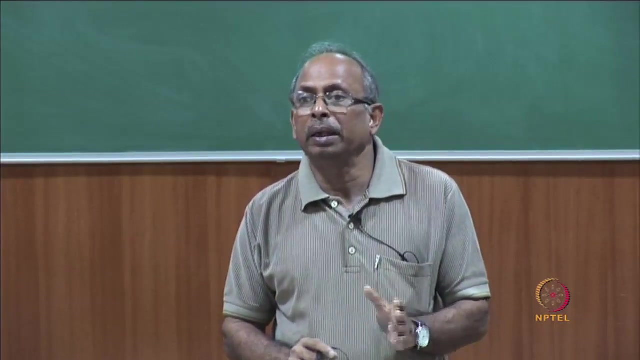 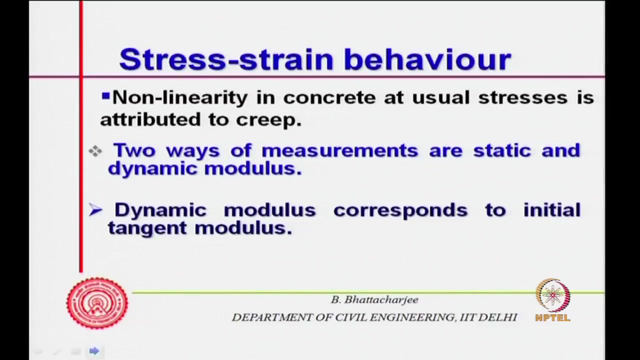 this medium you can actually estimate modulus of elasticity. Now that is called dynamic modulus. So dynamic modulus is related to wave propagation within the material itself, Because velocity of wave propagation or characteristics, you know, wave propagation is related to elastic modulus and one can determine that way. Dynamic modulus because there is no load applied, as 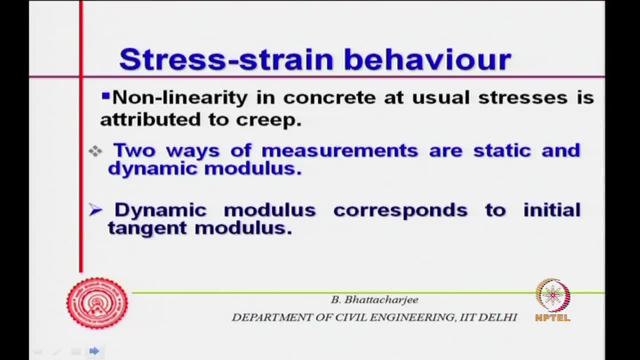 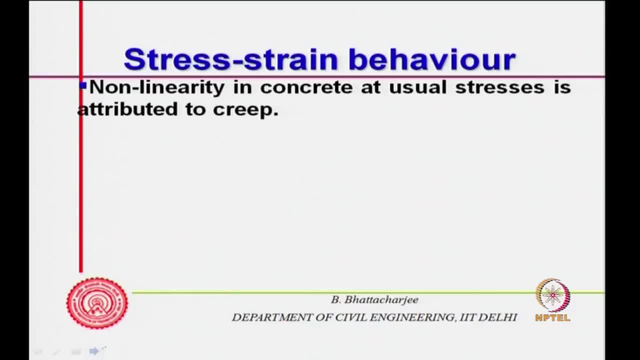 such in a big way and it actually corresponds to initial tangent modulus. So obviously this value will be higher than any other modulus because it is non-linear. Now, physically, of course, micro cracking of concrete at usual load results in apparently permanent deformation. 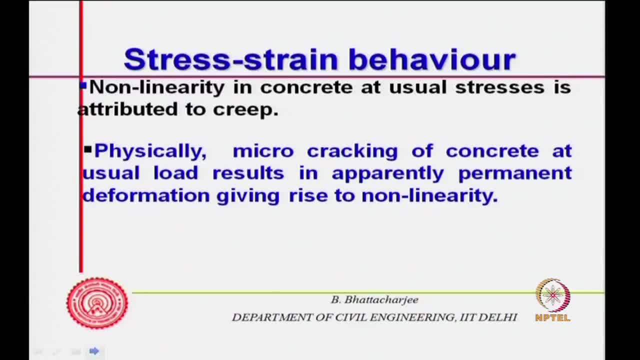 and that is why it gives rise to non-linearity. I mean, creep is one issue, but why finally So? micro cracking of concrete at usual load results in apparently permanent deformation, giving rise to non-linearity. That means you know whenever you are actually, for example, 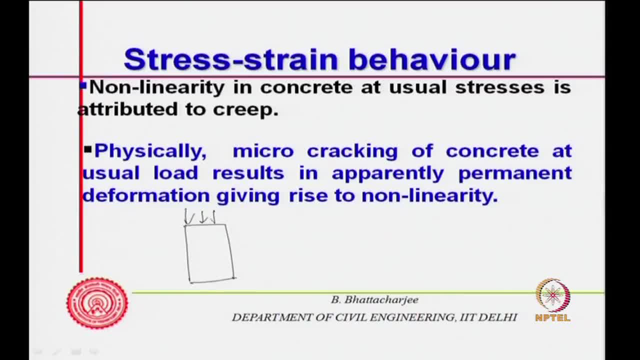 if I have a compressive specimen Applied load like this: Now, if it is sufficient, l by d is sufficiently large. let us say l by d is sufficiently large. l by d is equals to 2 or something of that kind. So whenever, 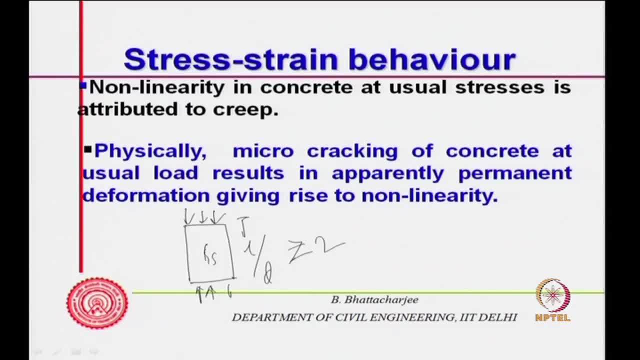 I am applying load. remember that we said the cracks will form here. There will be cracking, micro cracks will develop because of the tension along this direction. You know, you recall we discussed there will be tension along this direction and therefore micro cracks will develop. Now, after certain period of time, supposing, 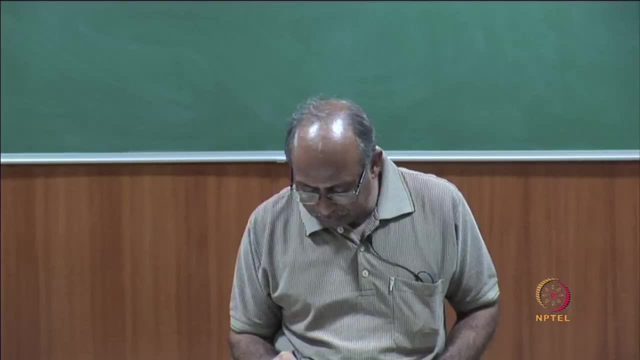 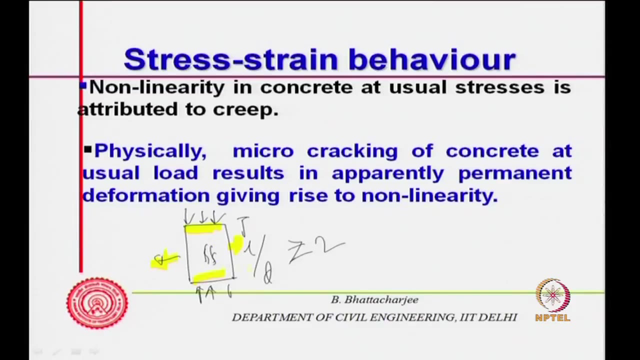 you withdraw the load. this you know, and this results in deformation along this direction too. So reduction in the length micro crack will form and there will be reduction in the length. Now, when you release this load, this micro cracks are not going to fill up. They 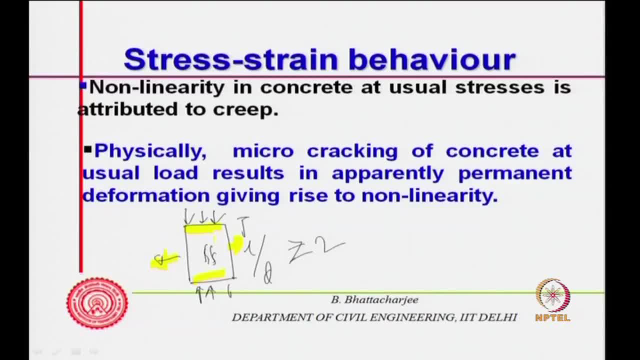 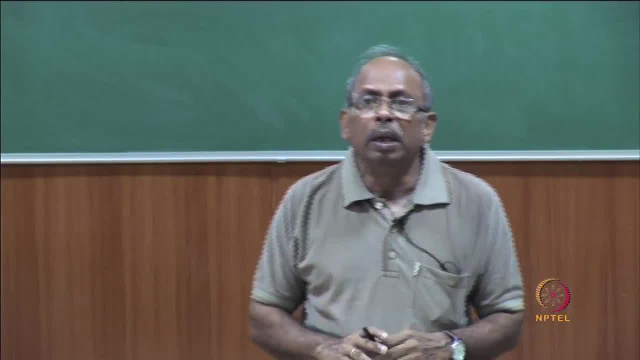 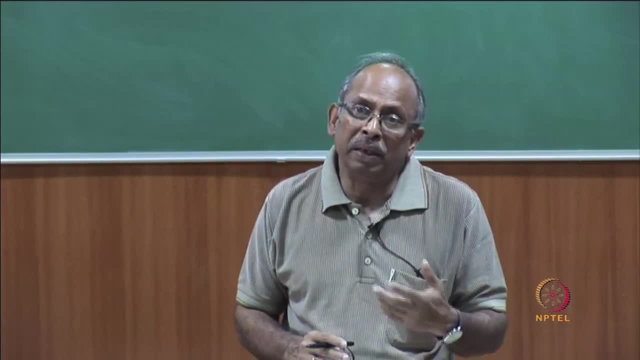 will remain as permanent features in the material and therefore the it will not go back to its original state. So once the micro cracks have formed, it will not go to its original state. So there is some kind of this- will actually, you know, manifest themselves. this: 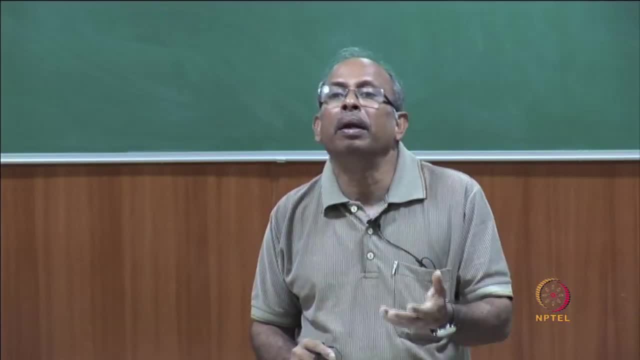 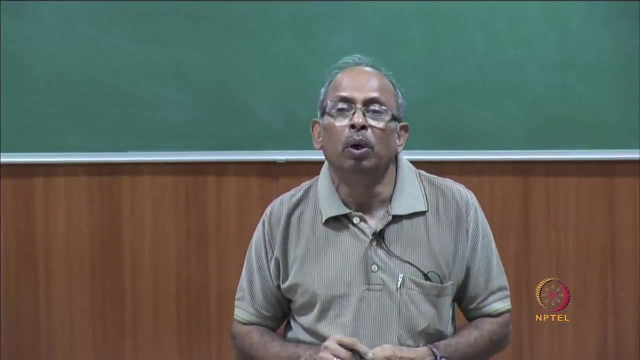 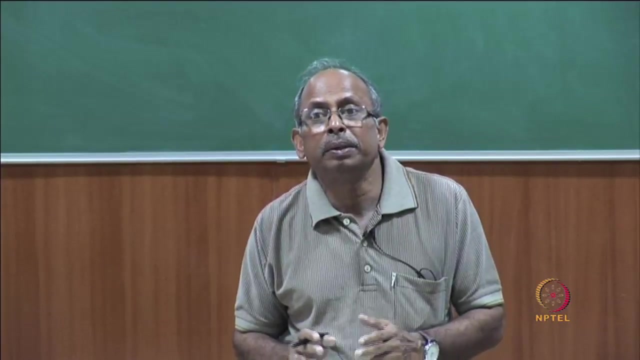 cracks manifest in terms of the deformation, permanent deformation, So therefore permanent deformation, this permanent deformation, and also this gives rise to non-linearity. So permanent deformation and non-linearity both comes to this, because suddenly there is a non-linearity. 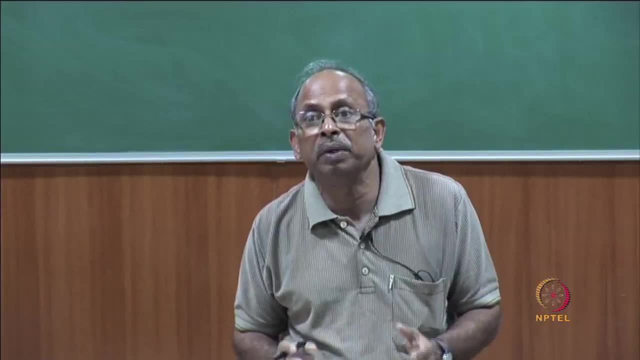 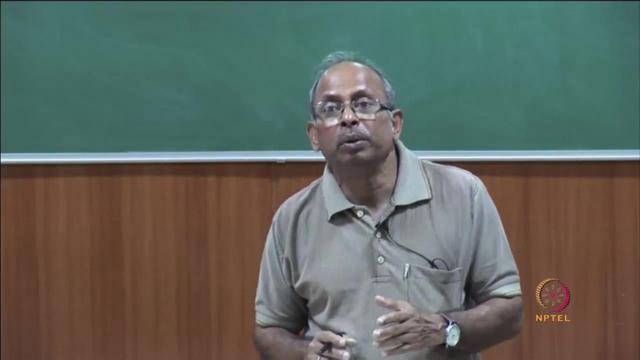 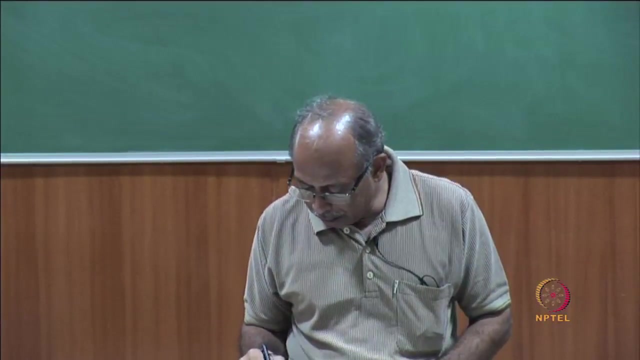 The given stress. suddenly there is an increase. the modulus of velocity, stiffness reduces because the cracks has occurred. So stiffness would reduce and therefore the material would tend to show lower modulus of elasticity or lower slope. So material shows a kind of non-linear behavior. to start with it is like this. to start with it is like this: you: 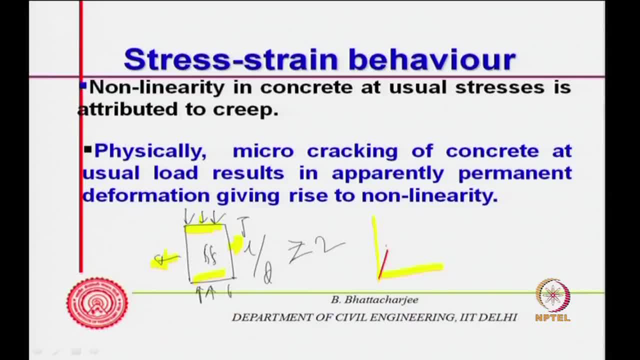 know it goes like this. but then there is suddenly there are lot of crack formation, So modulus changes and this, if this continuous, if this modulus is changing, then it will be show a kind of non-linear behavior. And if this cracks do not close, then it will show. 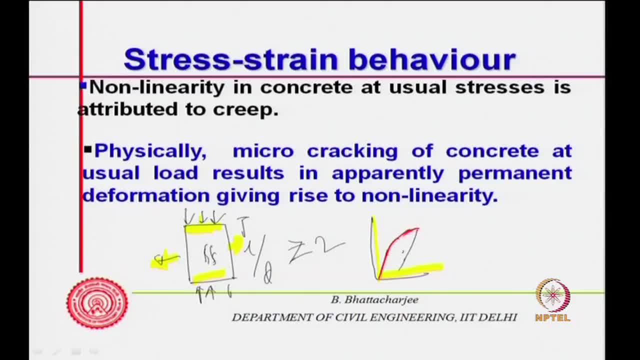 permanent deformation when it is coming back. when it is coming back, it will show permanent deformation. So that is the idea. that is the basic, you know explanation to why it shows non-linear behavior. Now this has been confirmed by test such as acoustic emission and ultrasonic. 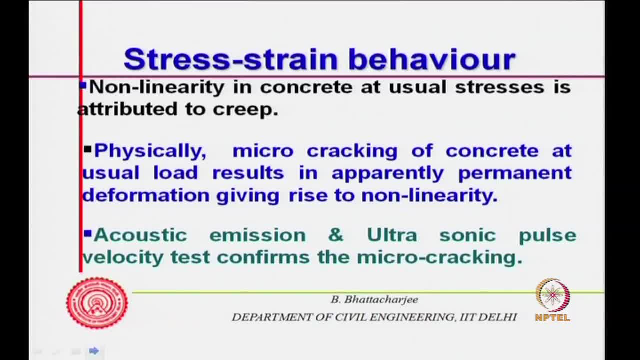 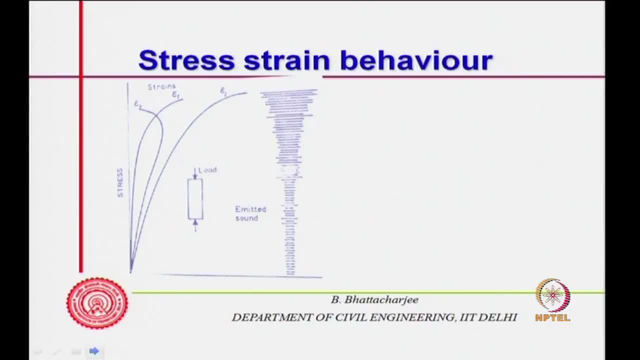 pulse velocity test right. So micro cracking is generally confirmed by this. Now let us see. let us look at this. So you see, if I look at, if I apply load like this, if I apply load like this, you know if I apply load like this on- a specimen is here- if I apply load. 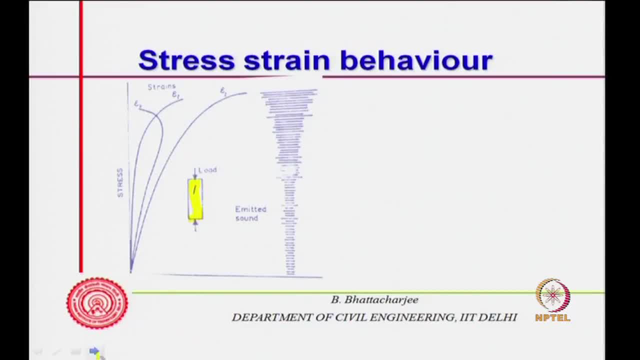 like this specimen is here: if I apply load like this, Now this is longitudinal strain, that means strain along this direction. strain along this direction, dimension change, So strain along this direction, that is longitudinal strain. Now this is transverse strain. that means, if I measure the strain along this direction, 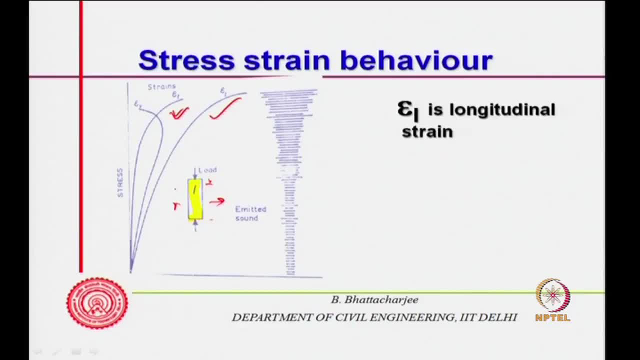 that is, transverse strain and volumetric strain, because volume changes, original volume change in volume divided by the original volume. Now volume actually can be a reduction in the volume change because this is reduction, this side- there is an expansion and net effect. initially there is an expansion, then there can be a reduction in the volume as such. 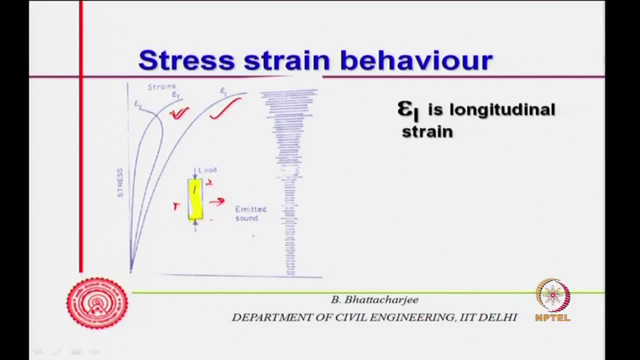 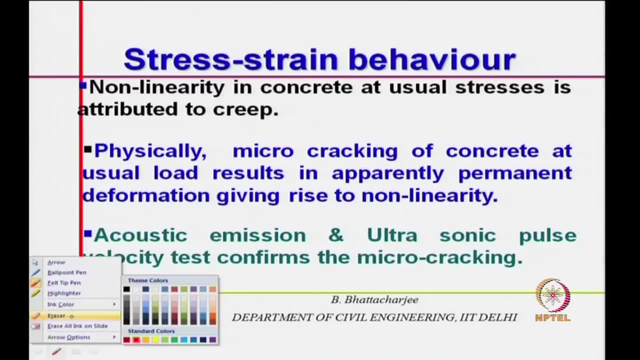 Now, what is acoustic emission? So this is acoustic emission. Acoustic emission: we just mentioned about acoustic emission a minute before. we mentioned that. you know you can when you do acoustic emission. acoustic emission- an ultrasonic pulse velocity confirms micro cracking. So what is acoustic emission? We will just quickly. 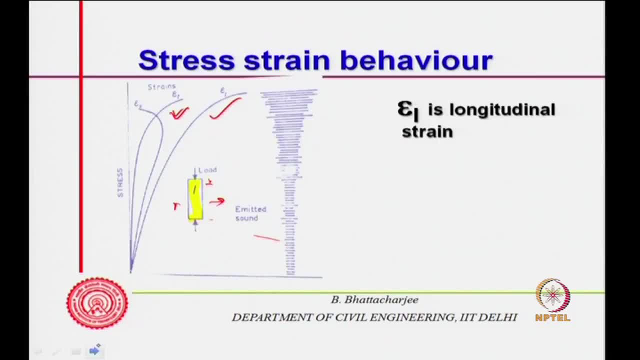 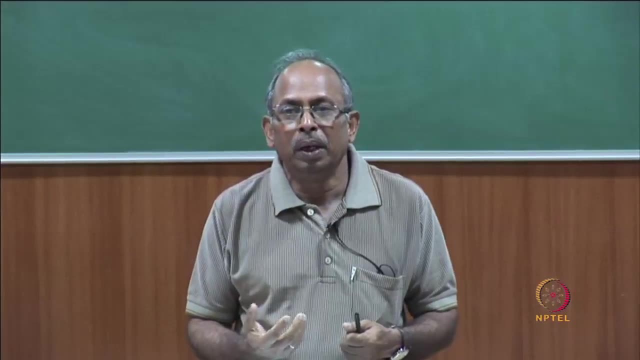 look into this for our purpose as much as is required for our purpose. So what is acoustic emission? You see, if you take, let us say, piece of timber or bamboo, simply right and try to break it, you will find that the sound comes out once it starts cracking, once it starts. 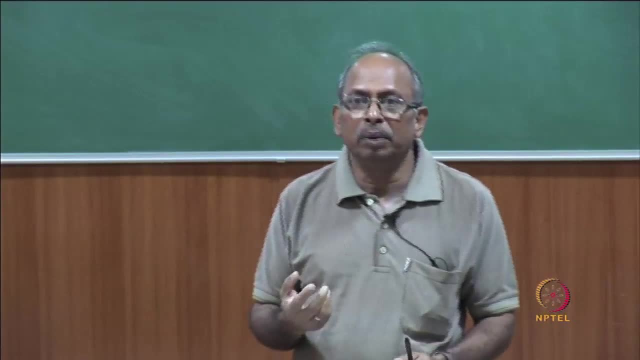 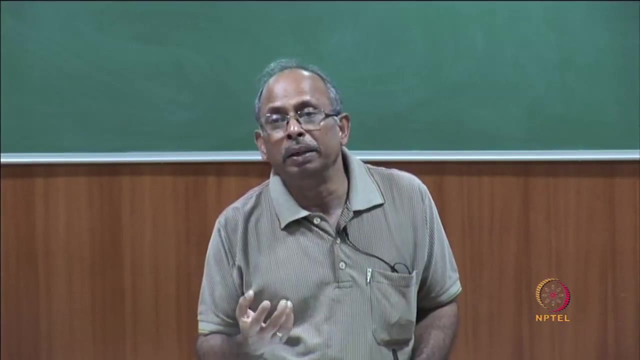 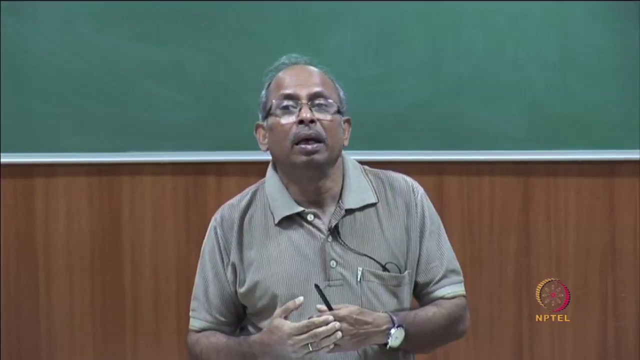 breaking. Now this sound is. you know some of the strain energy is converted into acoustic or sound energy. you know some of the strain energy is converted. So when you apply strain energy, part of the strain energy is converted into surface energy for creating crack. but 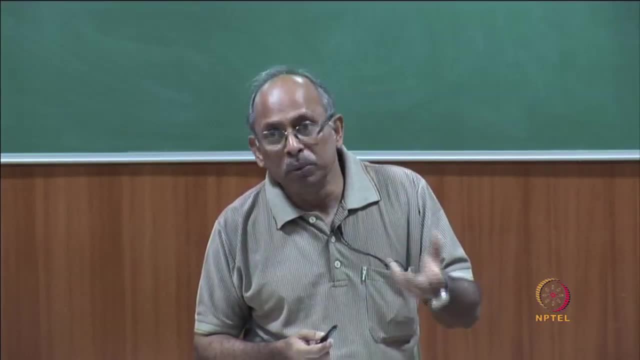 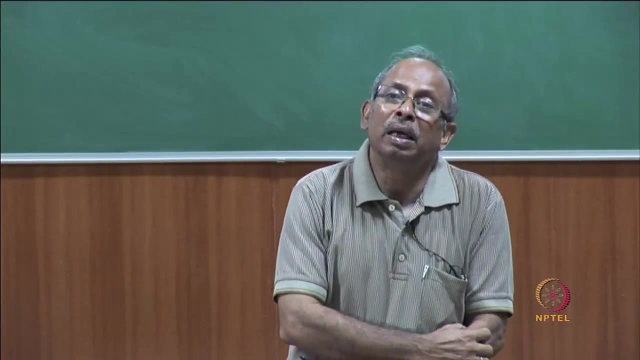 part might go as some sort of acoustic energy. So what is topographic positivo? because be hear sound. when you break a timber piece, you hear sound. So similarly a bamboo piece, you here sound. that is basically a kind of when it crack. So this crack, at the time of cracking there some sound emission. So 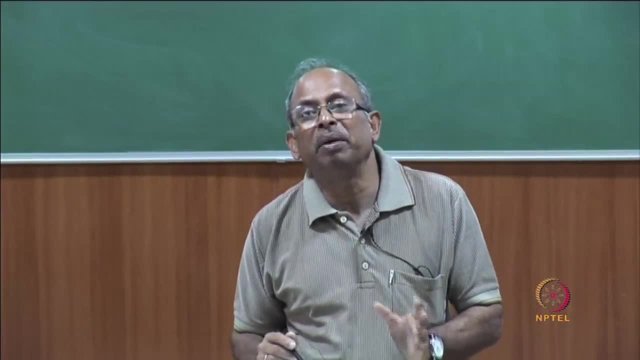 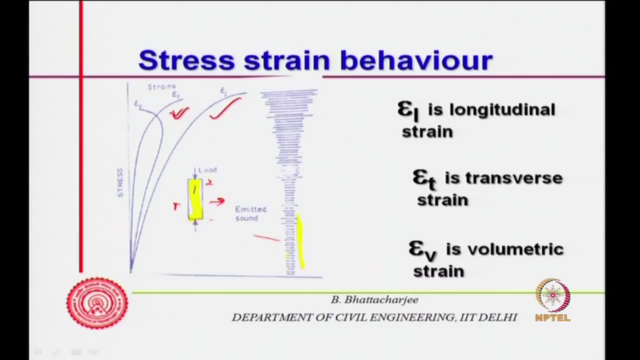 what has been observed in a, So that actually acoustic emission in a systemic manner one can actually trace this, find it out. So emitted sound as a apply the load as an increase. the load initially emitted sound is very less and then go on increasing and the sound starts. more sound emitted. sound becomes more 's. Derek, the next slide toma. 我們今天 番上ichts même ada很多聲音變了聽な音呢. destruction, starting from acoustic emissionぞ. 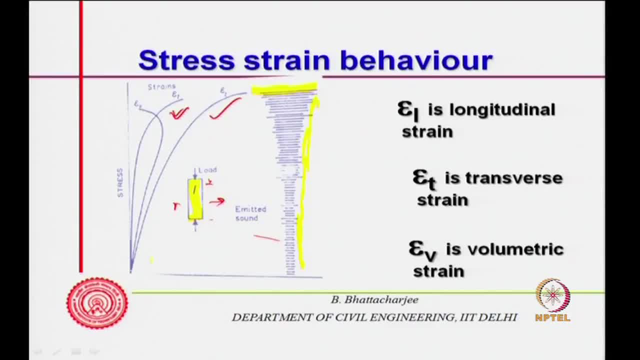 as the, you know, loading progresses, In other words, permanent deformations or non-linearity, is related to all. these are related to somewhere: x, lot of cracking, lot of cracking, And this is confirmed by ultrasonic pulse velocity also. pulse velocity also, you know, sonic. 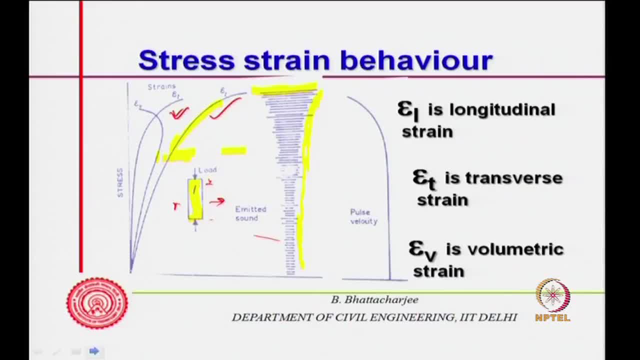 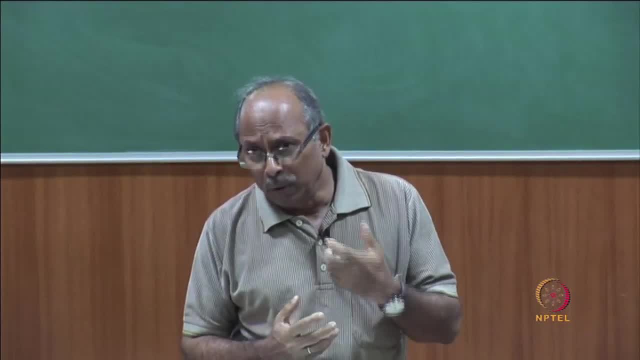 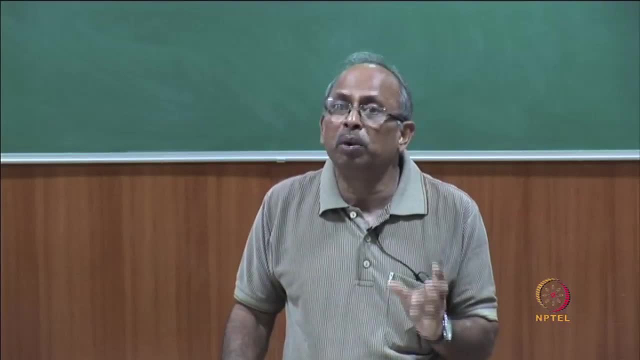 pulse velocity. Now, what is pulse velocity in a solid material is more compared to crack material, because velocity of sonic or mechanical waves in solid concrete, very solid concrete, could be of the order of around 4.5 kilometer per second. So they it could be of the order. 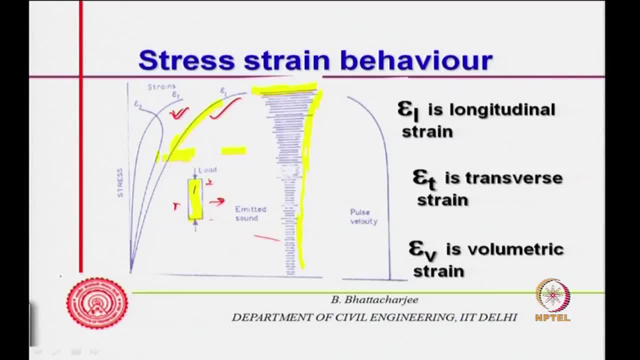 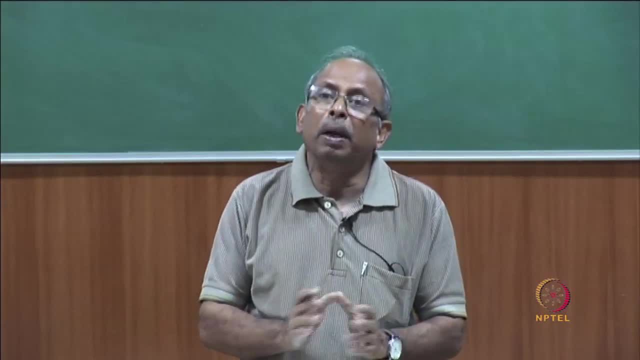 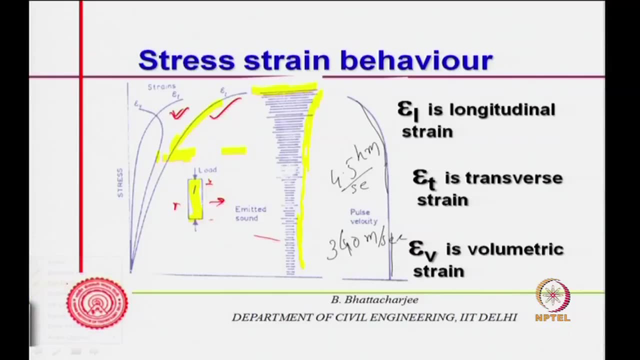 of cracking occurring. cracks have occurred, then pulse velocity will reduce. So pulse velocity starts reducing. Initial reduction is relatively slow. Initial reduction is relatively slow, but then it starts reducing as soon as lot of cracks starts appearing. So therefore, 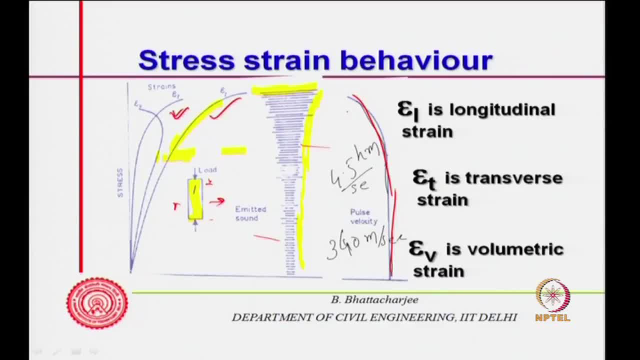 the cracking of concrete is confirmed by this kind of testing And therefore, if I am trying to plot the stress strain curve, you know stress as stress increases, longitudinal strain they. it shows that the nonlinearity, linearity of the stress-strain curve is largely related to micro cracking of concrete And 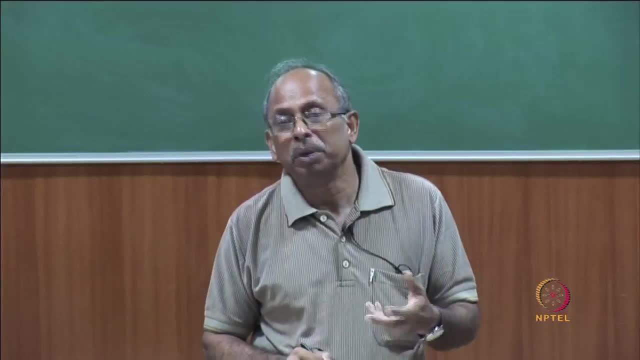 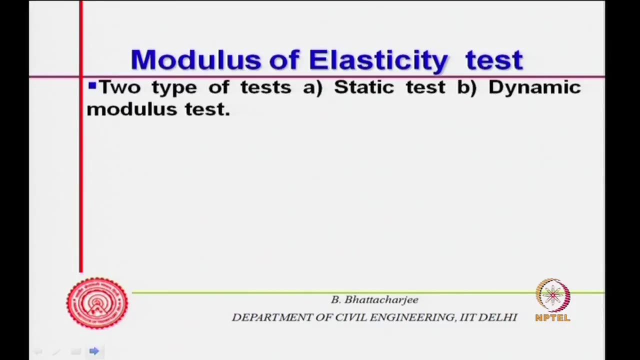 so is the case with permanent deformation. Permanent deformation is also related to micro cracking, So this is the reason why you get non-linear behavior. as well as there is a non-closure of the stress-strain curve, there is a hysteresis. 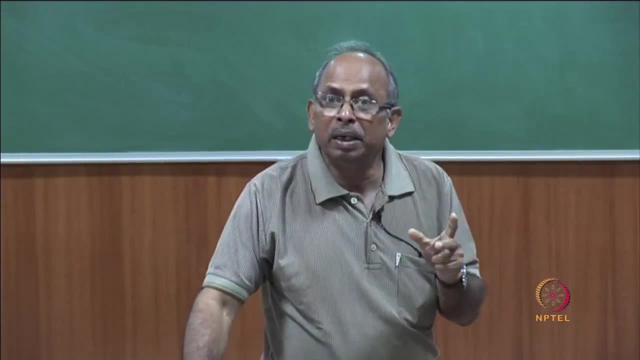 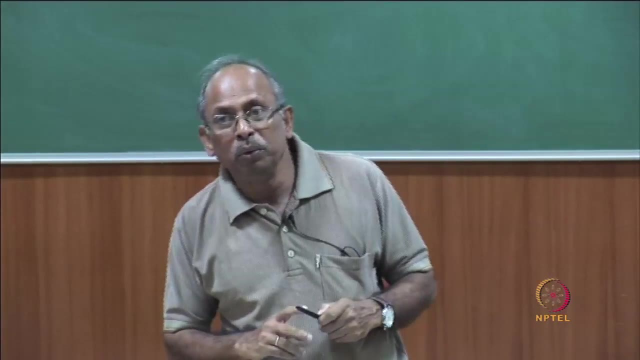 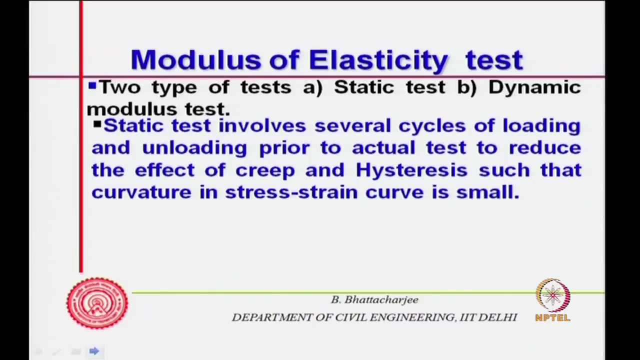 Now, I mentioned that I can determine it. you know I can have static modulus of elasticity or dynamic modulus of elasticity. So we got to do test in two different ways. Static test is done in a, you know, monotonic loading, But what we do is we actually initially apply. 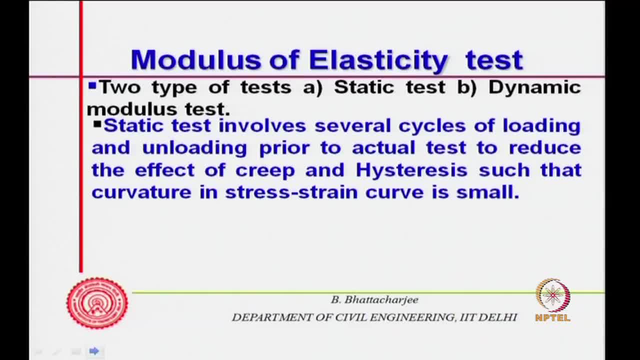 several cycles of loading and unloading at one-third of the estimated cylinder strength. You know, we normally test on cylinder. We do test on cylinders. So central one-third is used for metering, Central one-third is used for metering. This is the portion we 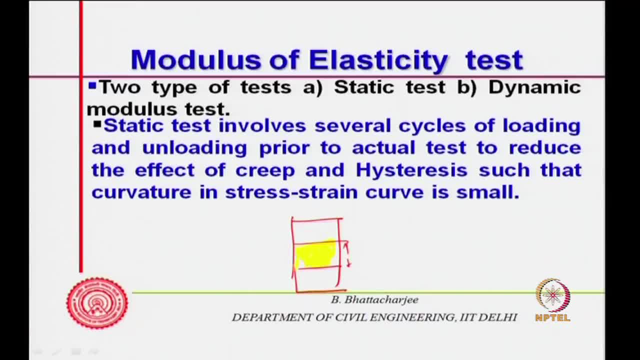 use for metering. This portion we use for metering, So you put gauges. actually, In good old days we had actually LAMS extensometer. It is called LAMS extensometer. you know, It is called LAMS extensometer. 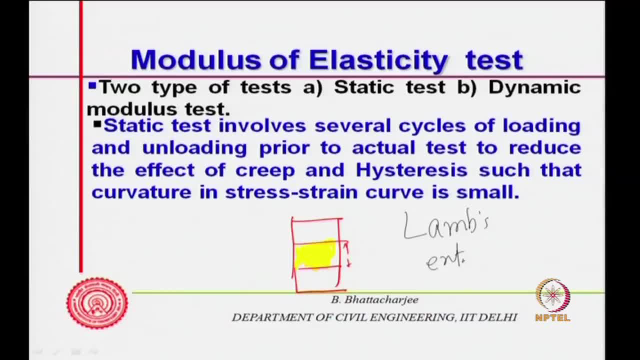 That is what we are using. So we will put the, actually the gauge, there. So in the central this will be 300 mm and central 150 mm. So you put the gauge here, but the deformation is relatively small. So how do you measure this deformation? It has to be amplified in. 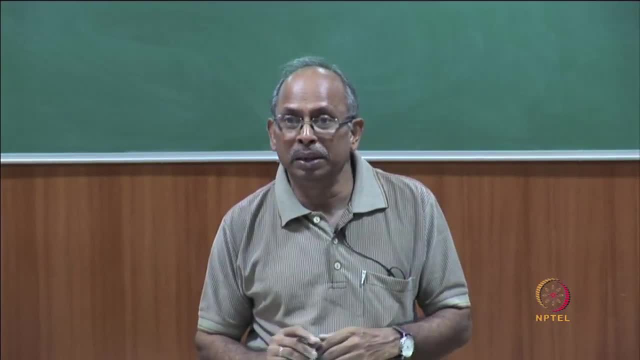 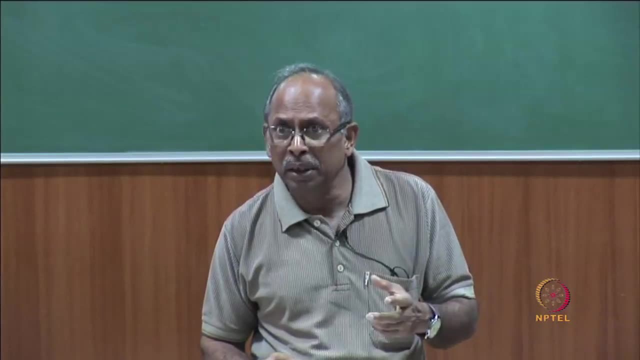 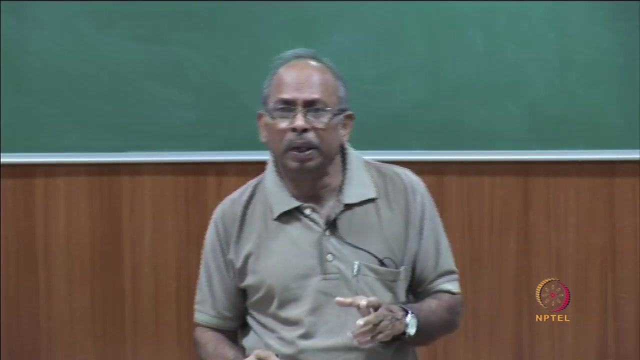 some manner It was actually amplified optically during those days, earlier days. Today, of course, you can put in several types of. you know, you can put in transducer of the kind of strain gauges, various kinds of sensing devices you can put in to measure, measure, measure this. 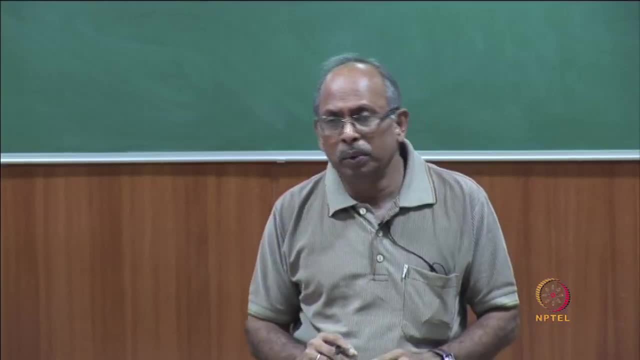 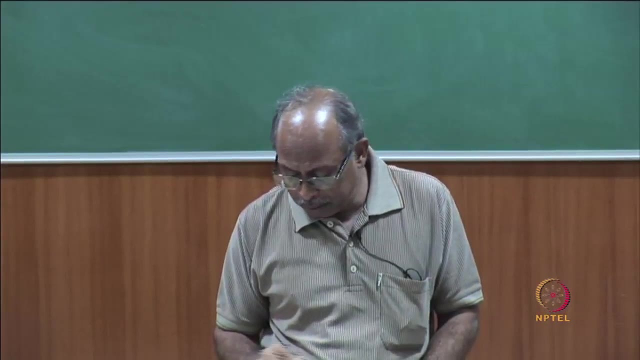 you know deformation. So several, several actually deformation measuring devices are there And one cannot strain. gauges could be there to measure this. So earlier days LAMS extensometer was used, So within anyway I am not going into the transducer part of it At the moment. 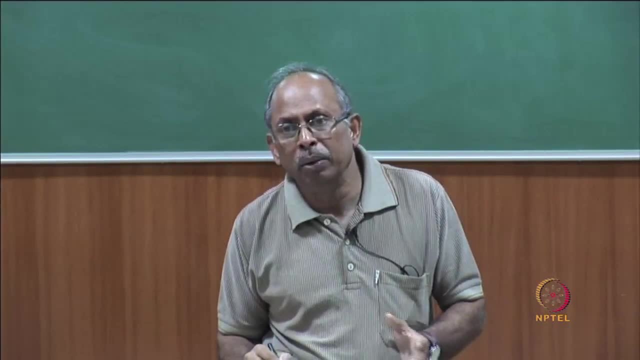 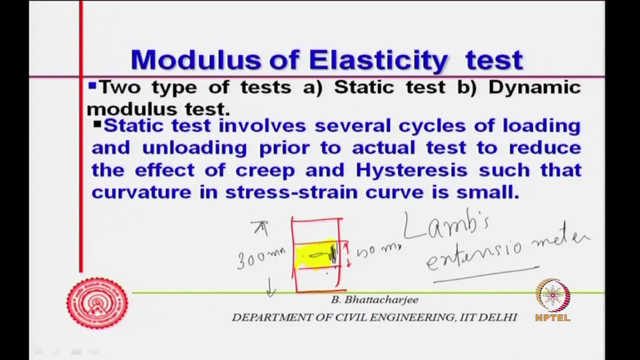 it is not necessary, but if you are doing a laboratory test, then you will be using any one of these. This was the old, traditional way- and then you measure the deformation there, the deformation there within the small range. But before doing that, what you do is you. 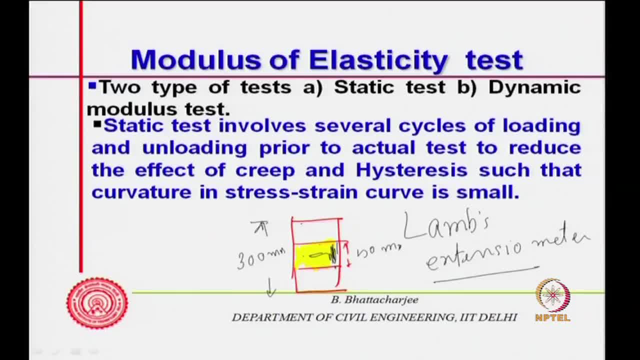 crush the cylinder to find out to the f c y cylinder failure strength And then load it up to one third of f c y l, that is cylinder strength, and then unload it. So this cycles are repeated to see that at least first of all the you know there is no, no, no, no in there. 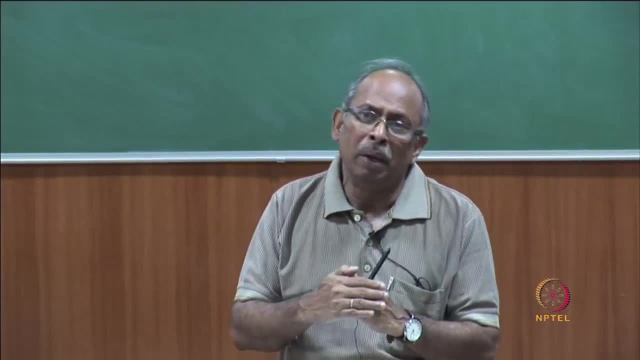 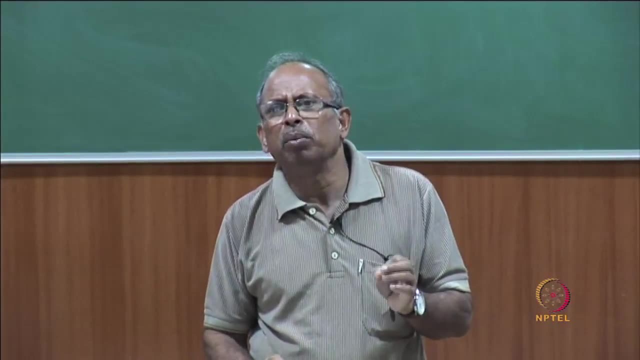 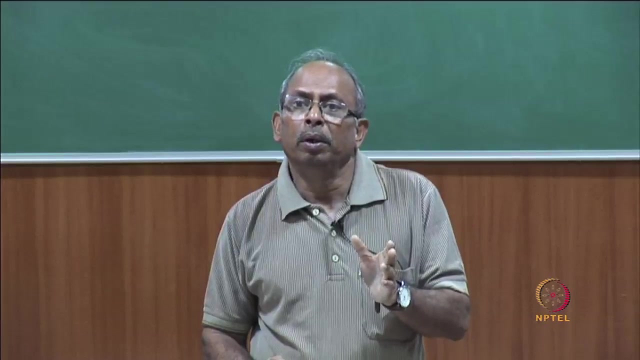 will be no deformation right in the beginning because of plate settling down and things like that number, Number of one, number two. this is prior to micro cracking or whatever small cracks that occurs would occur, And then after that actually the actual test will be done. So this will reduce down the effect of cript. 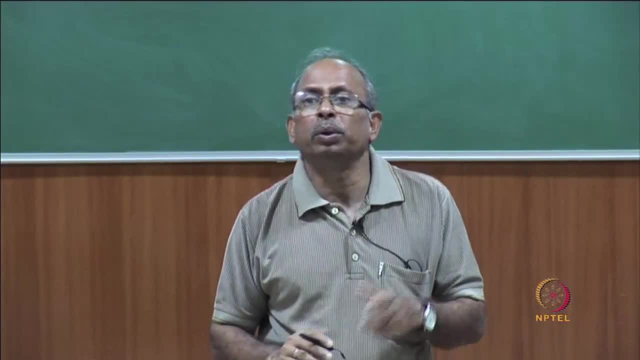 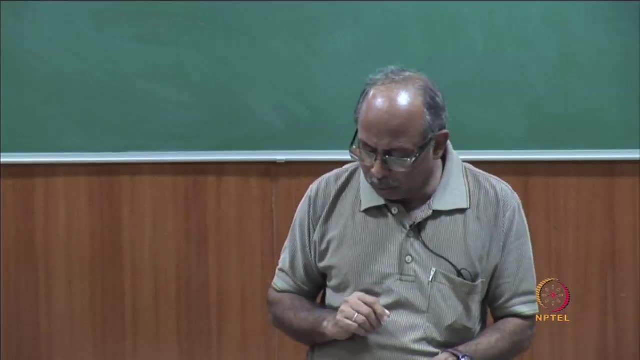 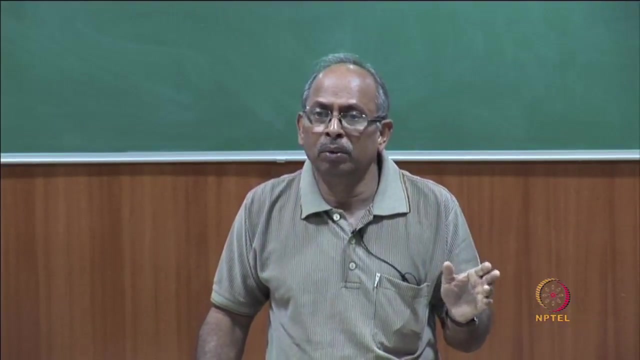 some micro cracking would occur and then hysteresis also will be reduced because of such micro cracking and permanent deformation. So besides that, there is another important issue why you do it this way. the load is never applied one time in a structure. For example, if you consider the room you 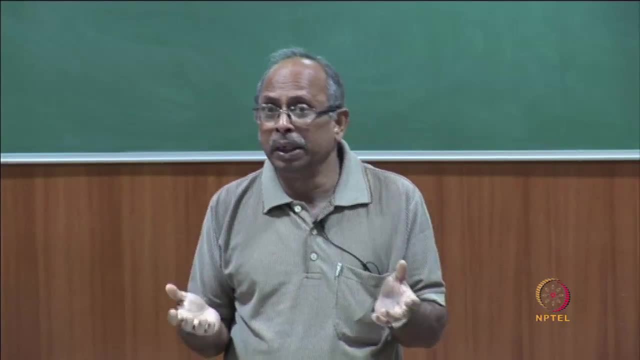 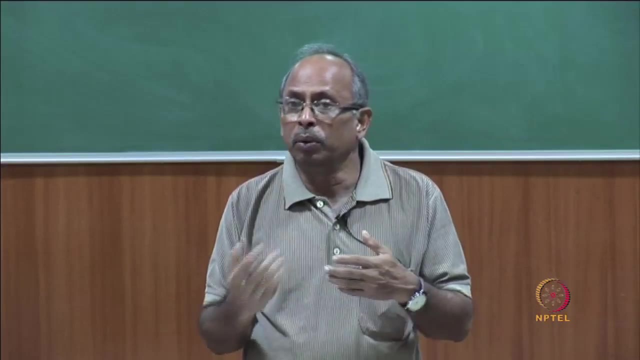 are sitting and if it is a reinforced concrete slab on which you are sitting, prior to actually even loading, there will be several loading and unloading that would occur, actually during construction phase or even later on several loading and unloading that occurs. So, therefore, 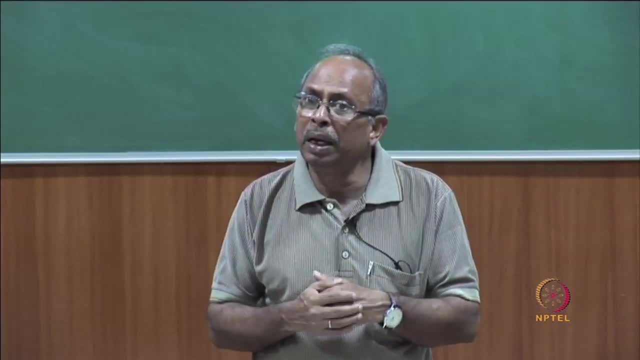 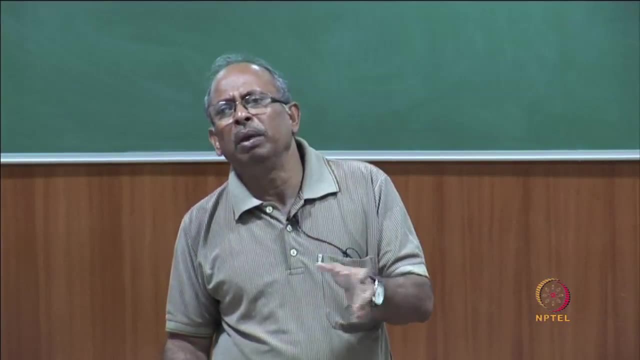 measuring the stress strain curve after some loading and unloading that is worthwhile. So what you do, we actually do about 15 times loading and unloading. you know the codes. most of the codes would tell you how to do error. So roughly about 15 times I think most of 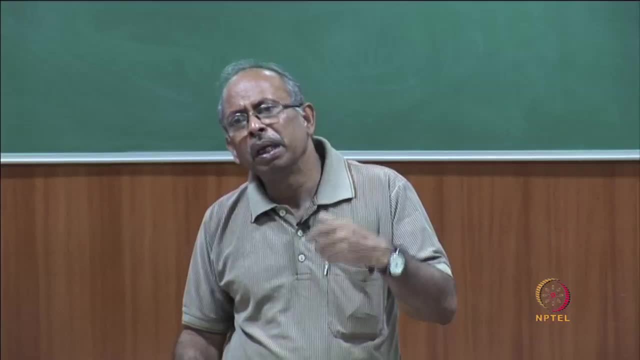 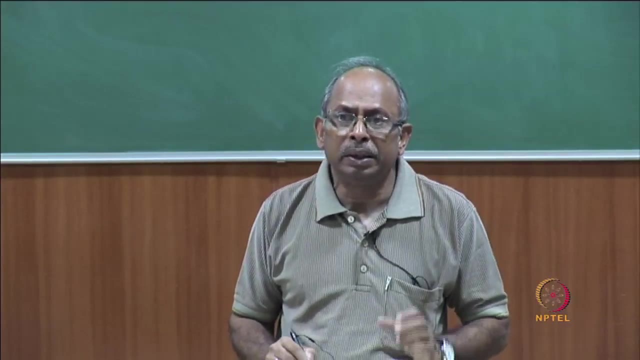 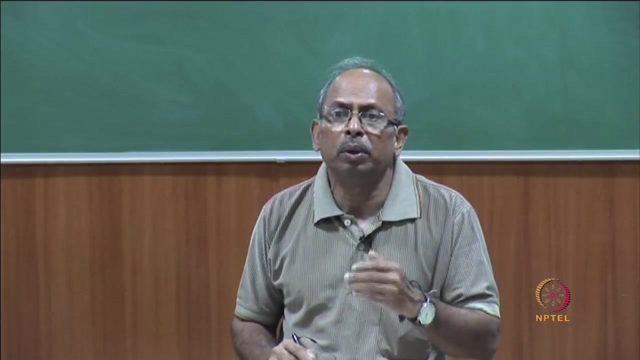 the codes would say: 15 cycling, 15 times, you know loading and unloading, and then you measure the actual strain versus stress. So load is then applied monotonically in steps and corresponding steps, corresponding strains are measured and it is plotted. it is plotted. 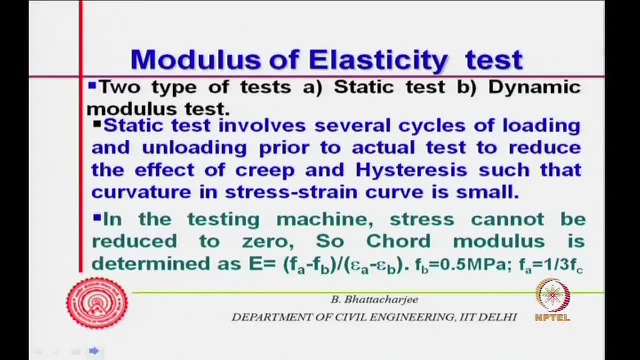 So in the testing machine, of course, stress cannot be reduced to 0. So what you do is: we will find out chord modulus. Finally, after this curve is obtained, we find out chords modulus as given by this formula: chords modulus. So we find out a chords formula. So this: 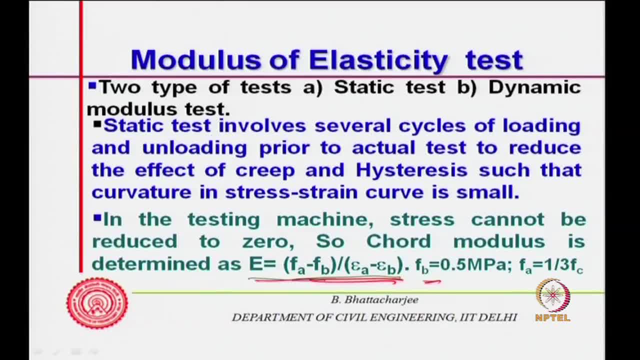 is the stress So F b. So we actually find out chords, modulus, like this. you know, because this is this, is difficult to reduce it to 0.. So corresponding to 0.5 m p a. this is epsilon, this is sigma: 0.5 m p a, and then So F b, So corresponding to minimum stress. 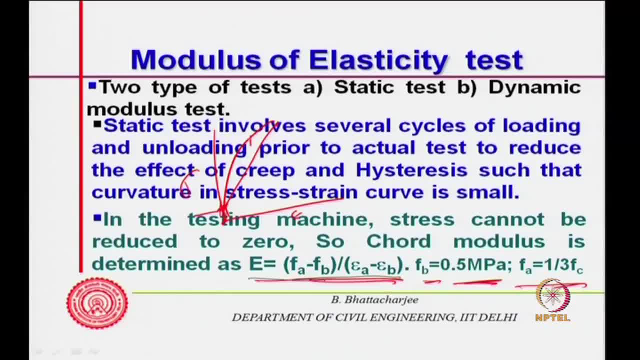 of 0.5 m p a, then up to one-third f c, one-third f c, up to one-third f c within the you know, kind of severe micro cracking prior to severe micro cracking. So F a minus F b, epsilon a minus epsilon b. So you find out, this is your epsilon b. 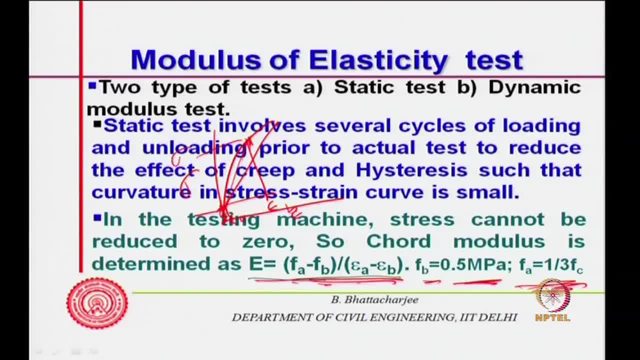 this is your epsilon a and sigma or f or whatever you call it. So you find out a chords modulus according to this, or you know So the code suggest how much where you have to go to test. So f c, one-third f c, is the elastic element and often you might find it, often you might. 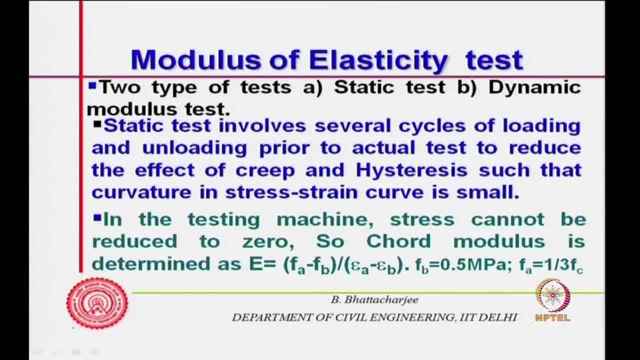 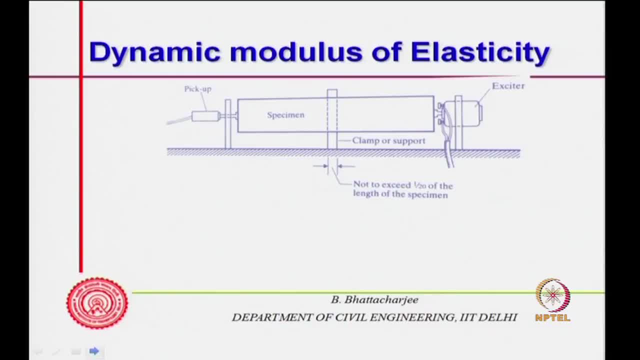 find it there itself, All right. So this is how we determine the static modulus of elasticity. Dynamic modulus of elasticity is determined in this perspective view of the diagram that you see, You have a clamped support which should not exceed 120 or the length of the specimen. So this is length. 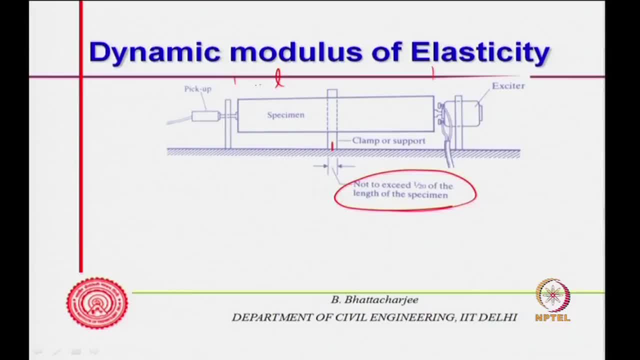 of the specimen. this is length of the specimen. this is l, the length of the specimen right. this is l, and this should not exceed l by 20. So you should not exceed l by 20.. So it should be less than l by 20. there is a clamp of the support, So a specimen rectangular: 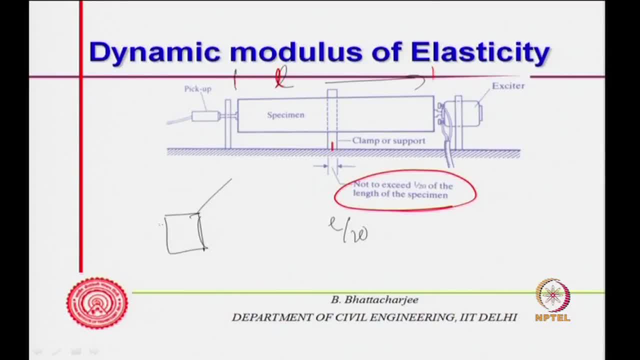 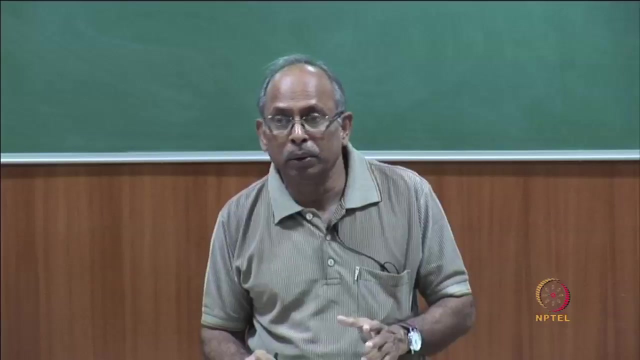 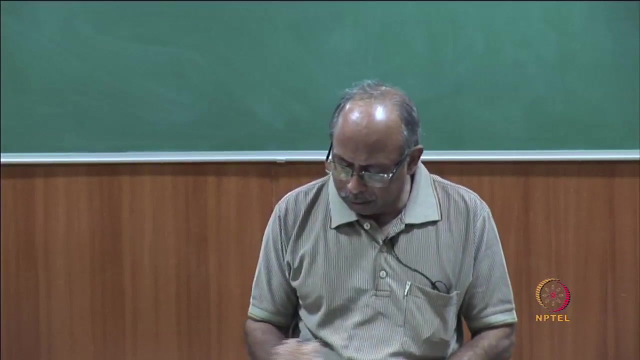 specimen generally: rectangular cross section. you support it, rectangular cross section actually. you, you, you know, clamp it somewhere in between, like this, and then you have an exciter. you have an exciter that actually imparts acoustic, imparts actually acoustic pulses or acoustic, you know, wave basically there, So there is a longitudinal wave will be travelling along. 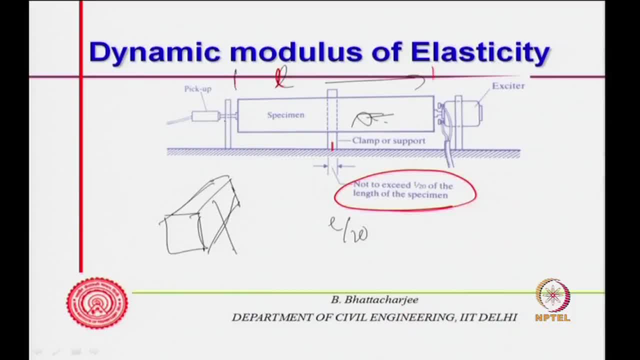 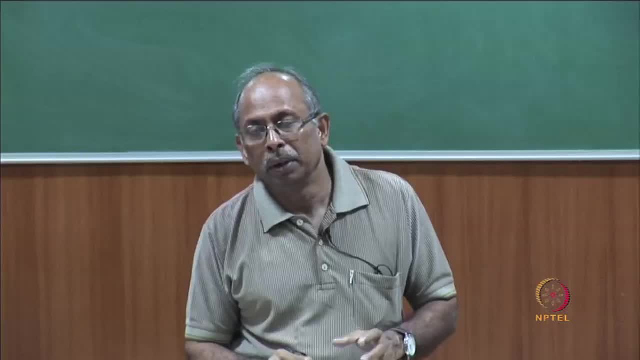 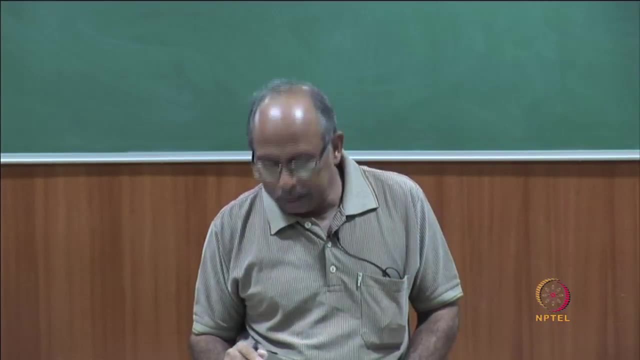 this direction, they will be travelling along this direction and here there is a pick up which will pick up the, the you know pulse transmission, So signal that is transmitted through it. So this is a, this picks up and at, as you go on changing the frequency of 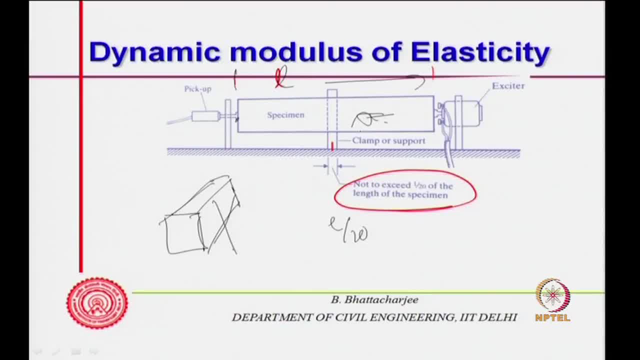 the sonic wave that is travelling along, Traveling along this direction. that is exciting. this, at time, will come. at certain frequency, there will be resonance occurring. right, there is a resonance occurring. resonance should be occurring when actually, this dimension of this one matches with the wave length. I 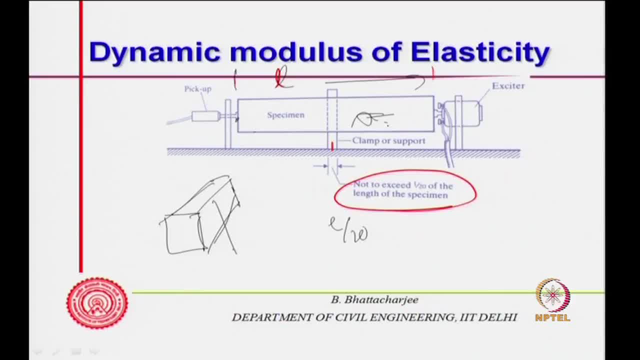 mean some sort of matching with the wave length of the, because the mode would depend upon, because it is a central support, you are trying to vibrate it and it will be related to length of the. So the resonance frequency is related to length of the specimen itself. now how it is. 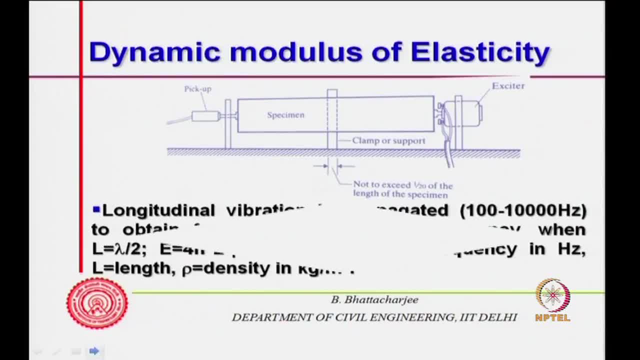 related. it is related like this: longitudinal vibration is propagated, you know So you will have vibration along this direction. longitudinal vibration, So it would be actually, it would be actually exciting in, you know so, longitudinal vibration, So compression and rarefaction, they will be travelling along this direction and from 100 to about 10,000 hertz at 100. 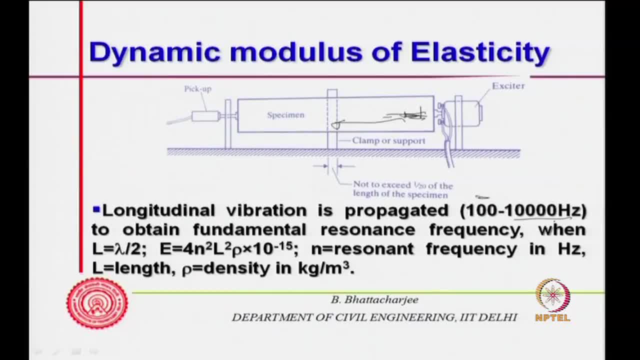 to 10,000 hertz. this range you actually make it to propagate and you will get fundamental resonance frequency when lambda is equals to, you know, 2 l, So when wave length is equals to 2 l, where l is the length. So or lambda is equals to l is equals to lambda by 2 at. 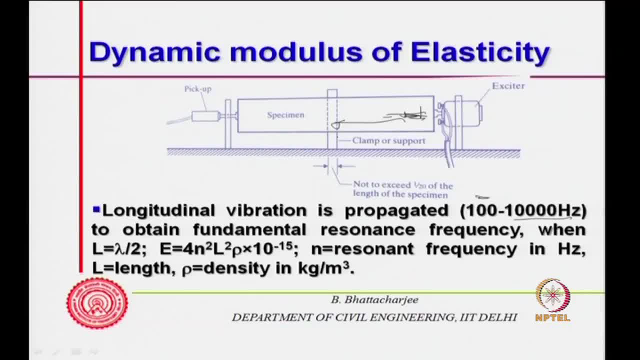 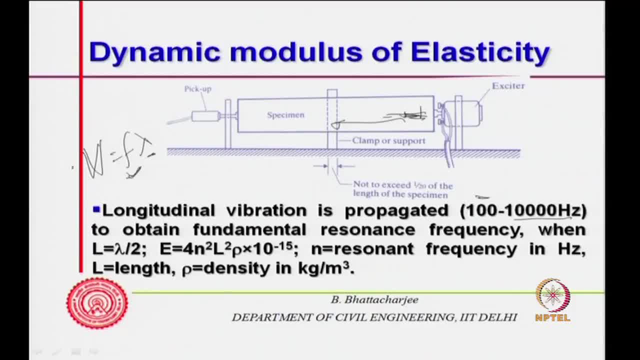 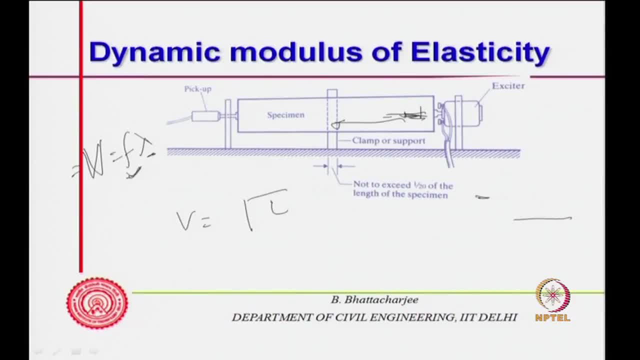 lambda is equals to 2 l, lambda is equals to 2 l and v is actually last. just I mentioned a few minutes before v is a function of e by rho. v is function of e by rho. Therefore you can actually relate e. actually you can relate to. v is a function of e by rho. So 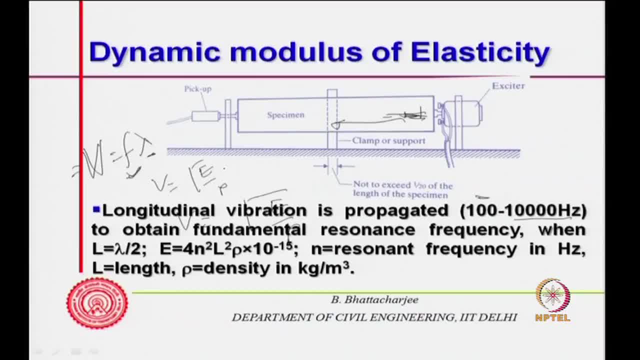 v is a function of e by rho and is also equals to f, lambda- And lambda is actually resonance. frequency is known. lambda is given by this equation: l is equals to, since you know l, so lambda is 2 l. in other words, you can find out e because f is known, l is known and this 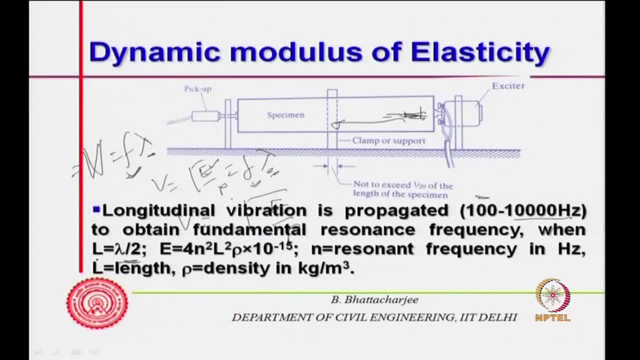 is this 2 l? l is known, this is 2 l. So you know, you know you can actually find out four n square l square rho, 4 n square n. you know, 4 n square l square rho into 10 to power 15. 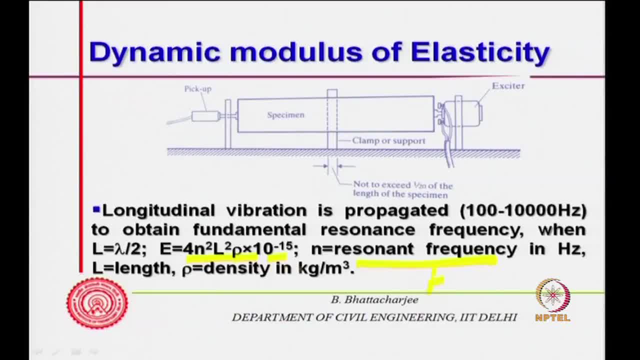 where n is the resonant frequency. you know f that I was saying, n is the resonant frequency. So you determine resonant frequency. So resonant frequency, this is lambda, you know by 2.. So therefore velocity, and then then velocity is, and then the rho comes into picture. 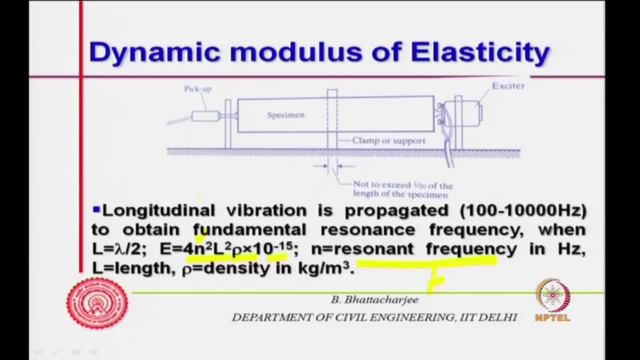 because velocity is under root e by rho. So if you want to find out the e, it is proportional to v square, So rho v square, So e is actually. e will be proportional to. e is proportional to rho v square, So rho v square, and therefore you can find out. v is given by n lambda and. 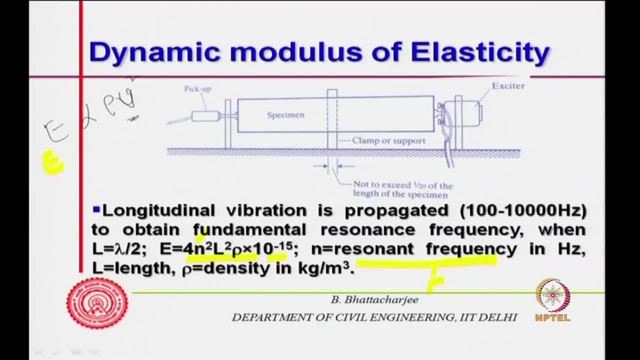 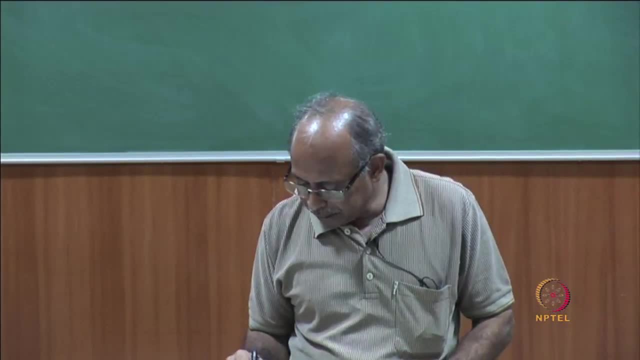 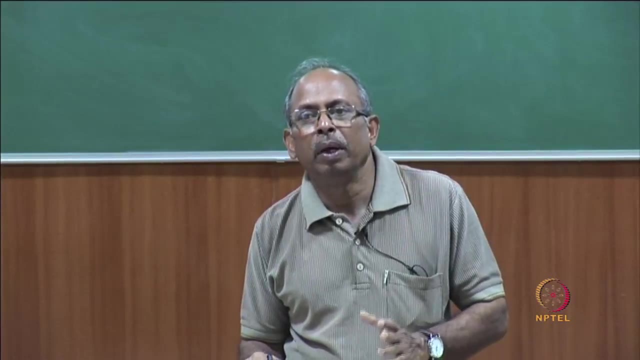 from the dating from, therefore knowing the density of the material. So you have an assume density or measured density. the material, from the data find out the modulus. So dynamic modulus can be determined in this manner. first, what you do is actually in part longitudinal vibration or mechanical way. So excited, excited, so acoustic wave. 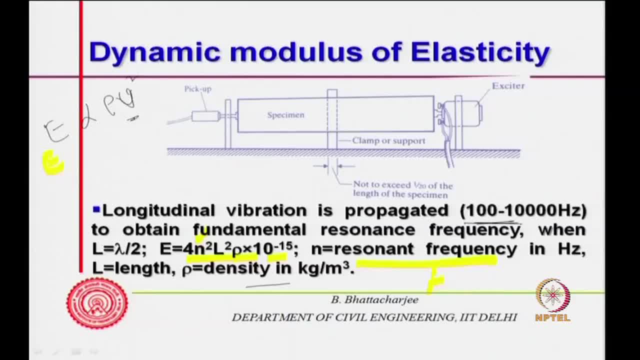 with excite, through acoustic waves or ultrasonic, you know sonic waves from 100 to 10,000 kilo hertz, because 10 k, 100 to 10 k, alright, So it is actually sound, because sound is. 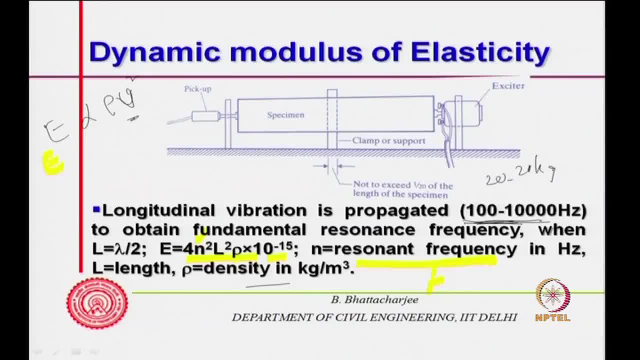 from 20 to 20 kilo hertz, So it is not ultrasonic. this is kilo hertz, So this is not ultrasonic. this is actually sonic excitation you can provide and then find out from this modulus of elasticity. So this is how you find out the modulus, dynamic modulus of elasticity. 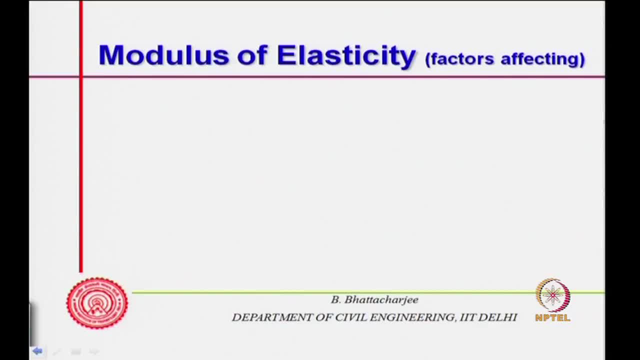 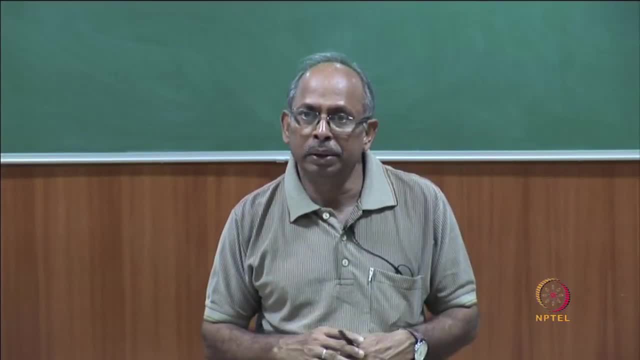 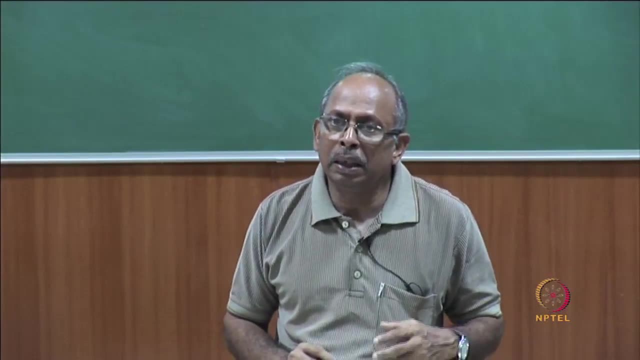 and we said that dynamic modulus of elasticity is initial tangent modulus, because no cracks have occurred. nothing has occurred in an uncracked specimen is actually you are trying to find out the modulus of velocity. Usually these values are higher. So now let us look at modulus of elasticity in terms of the. what are the factors that? 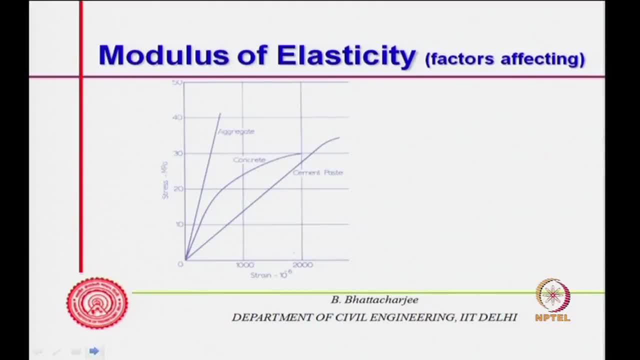 affect. So factors affecting modulus of elasticity. first of all, you see, you have to know the velocity. Here is your cement paste. This is for cement paste. If you see, this is for cement paste. This is the stress strain curve of cement paste. This is the stress strain. 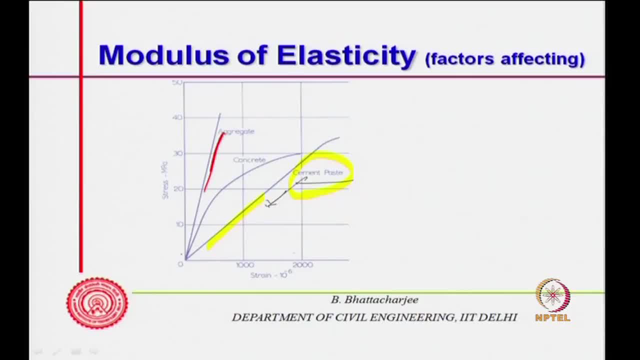 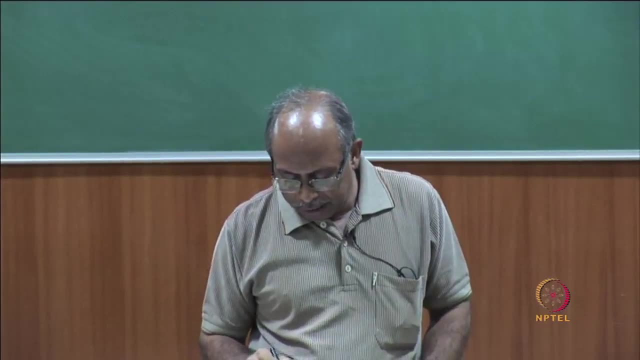 curve of aggregate. Generally it would show something like that, and concrete shows a stress strain behavior of this kind. So aggregate stress strain behavior is of course fixed, you know. thus fixed by I mean you have taken the rock and the behavior will be fixed. 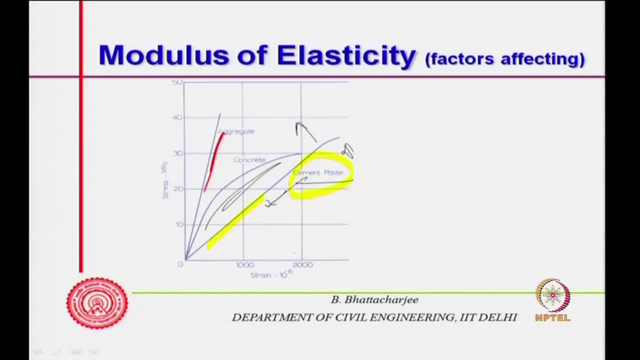 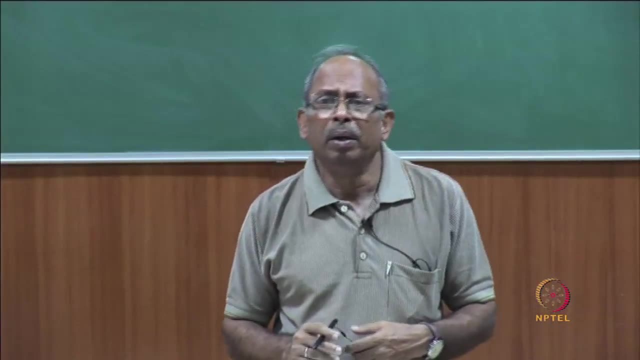 Cement paste of course is under your control. So if you improve this cement paste modulus of elasticity, concrete modulus of elasticity also will increase. So it depends upon both the paste modulus of elasticity and modulus of elasticity of aggregate. I mean one can think in terms of the range will, of course 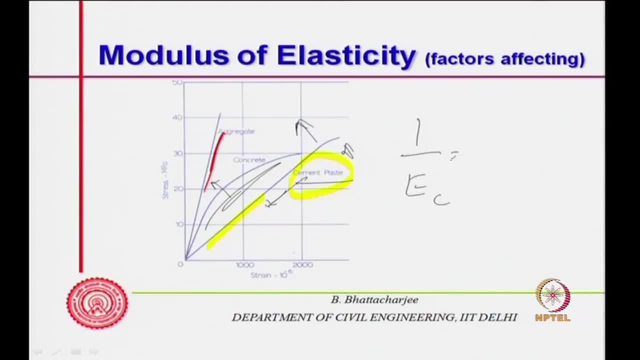 be something like 1 by e of concrete, should be equals to proportion of the aggregate, p aggregate or proportion of the aggregate divided by e of aggregate plus 1 minus p aggregate. that is your paste, or proportion of paste divided by e of paste. or it might also be written as p aggregate- proportion of aggregate multiplied. 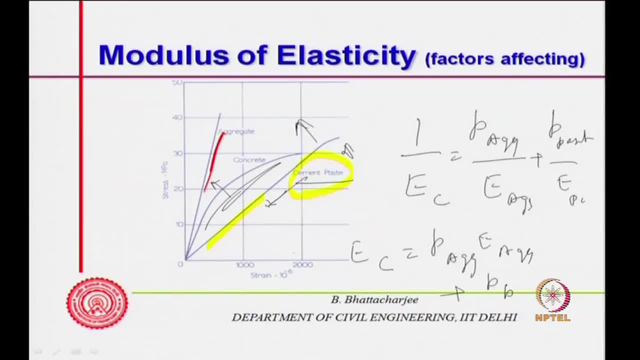 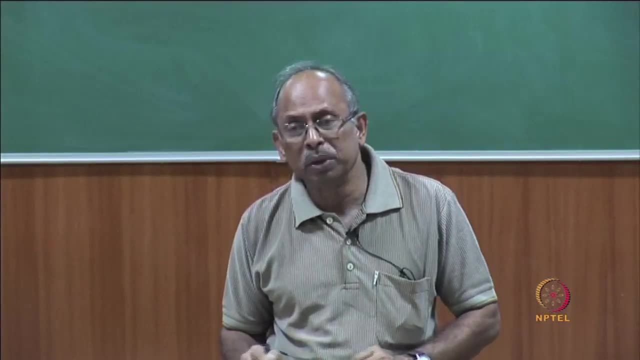 by e aggregate plus proportion of paste multiplied by e paste. This too will give you actually extreme boundary of the the you know concrete modulus of elasticity, assuming series and parallel model. I am not going to go to a derivation of this. 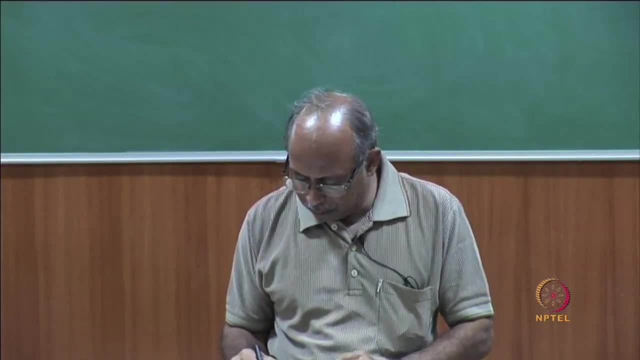 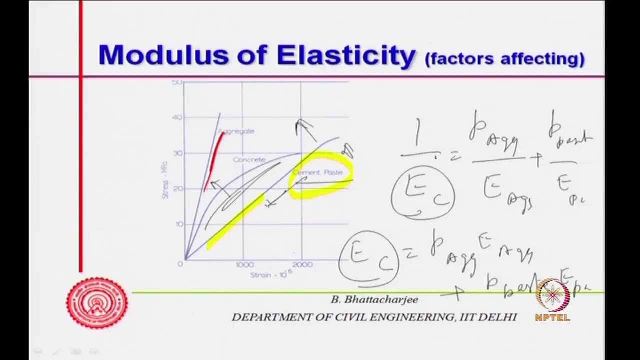 but you know this, of course, this the range, this boundary, this E c calculated from this or E c calculated from this, they give you two different values. So this gives you E c 1, let me call it This is E c 2.. This will actually give you the wide range of the modulus. 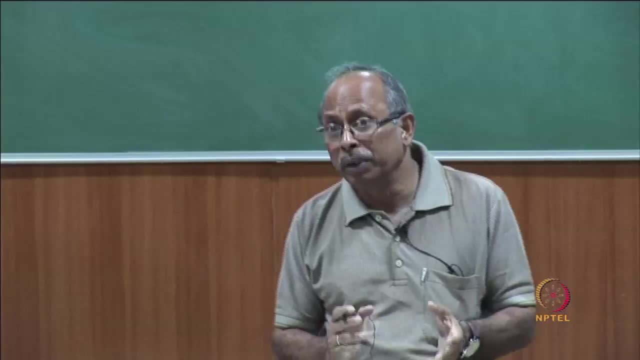 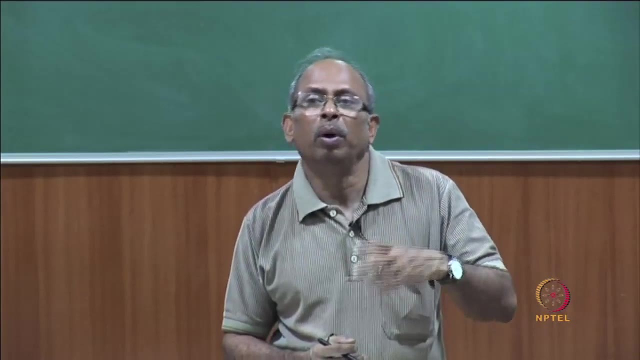 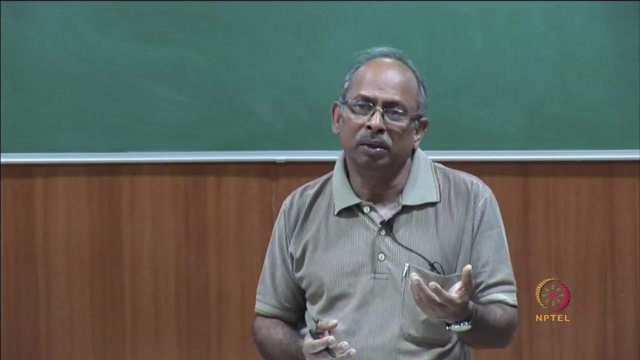 of elasticity. but at the moment it is more important for us to understand the modulus of elasticity of concrete as a function of modulus of elasticity of the paste and modulus of elasticity of the aggregate. So high modulus aggregate will tend to give you higher modulus elasticity for concrete and high modulus obviously paste modulus. 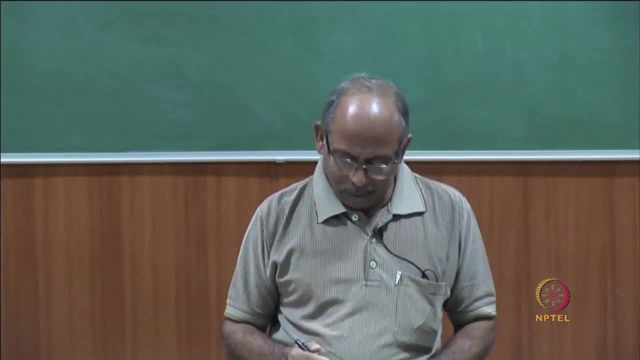 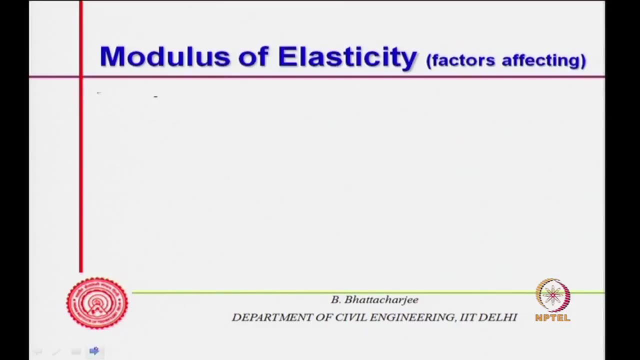 if you improve by increasing their strength, then you can actually get higher modulus for concrete as well. So first thing is this: other factors where specimen exhibit higher modulus. Why? Because water has got a water has got water. E for E for water. 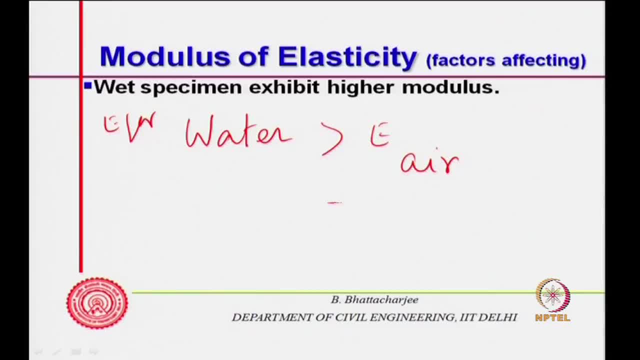 for water is more than E for air. Both are fluid, by the way, So wet specimen: the pores are saturated with water. For wet specimen, pores are saturated with water. pores are filled with water. They replace the air. So therefore, modulus of elasticity is likely to be higher because 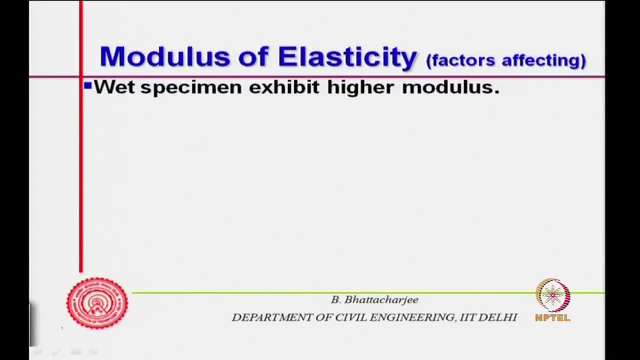 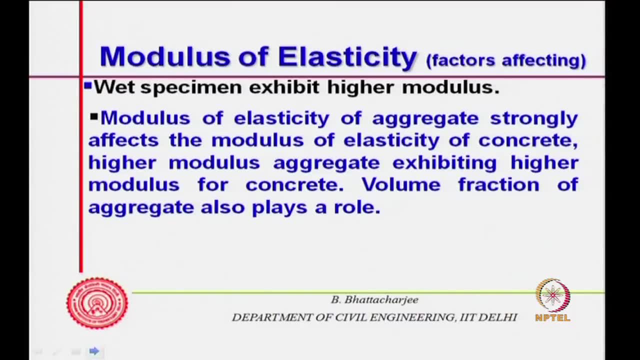 now it is, the pores are filled up with water instead of air. Modulus of elasticity of aggregate strongly affects the modulus of elasticity of concrete. Higher modulus aggregate exhibiting higher modulus of concrete volume of fraction of aggregate will also play a role. So this 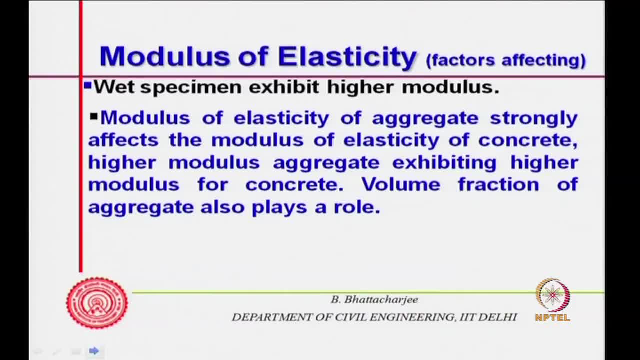 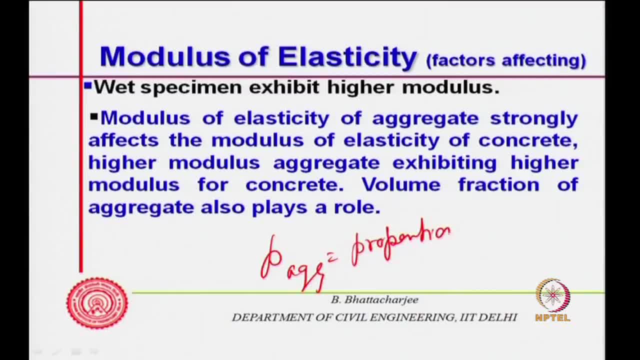 of aggregate proportion. proportion of aggregate, proportion of aggregate and p paste. p paste, let us say Paste which will be gives to 1 minus p aggregate, minus voids or whatever there are. So basically, proportion will play again a big role, Because whichever bounds you take, upper or 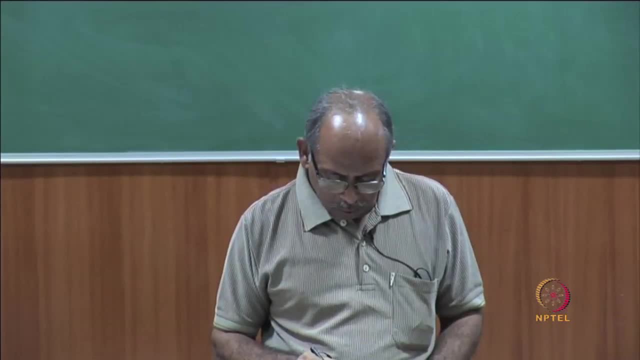 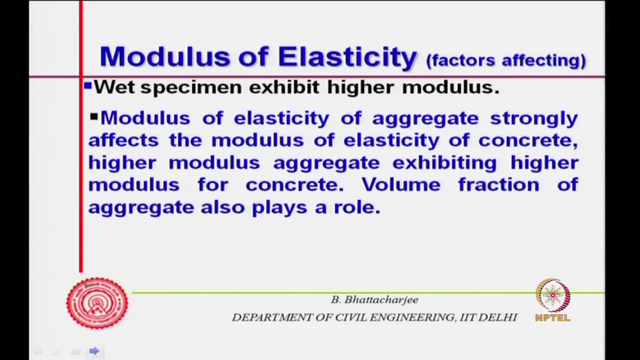 lower bound both cases is a function of those two. You know the series or parallel model which gives you bounds both cases. it will be related to that. Then mostly E can be related to mod f, c. well, compressive strength. Now E can be related. 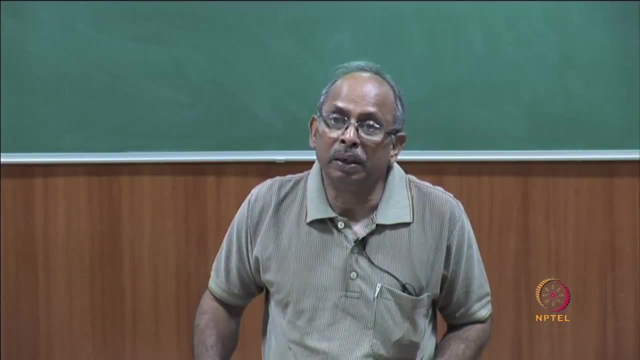 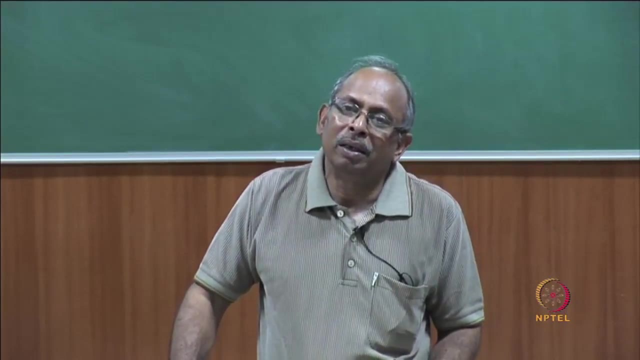 to compressive strength. you know it can be related to compressive strength. In fact, we have seen that modulus of elasticity governs the strength. Therefore, we can argue it out that strength would be strength would be also related to modulus of elasticity. 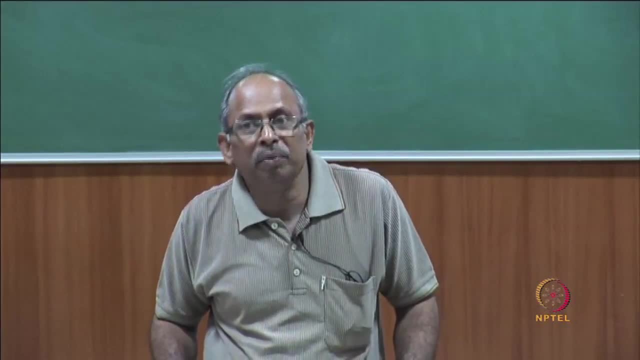 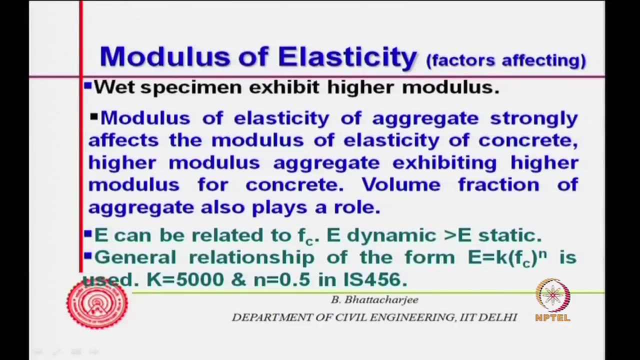 Dynamic modulus is somewhat close to initial tangent modulus. Therefore it is more than E, static and general relationship, empirical relationship people have found out for modulus of elasticity is E is a function of k into cube compressive strength to the power n. and you know I s 456 2000 for design uses this f c as f c k, characteristic strength and n. 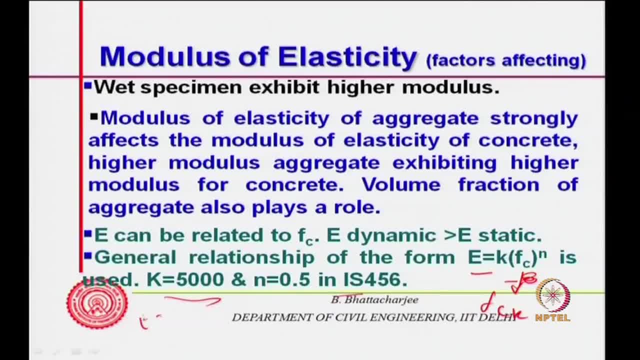 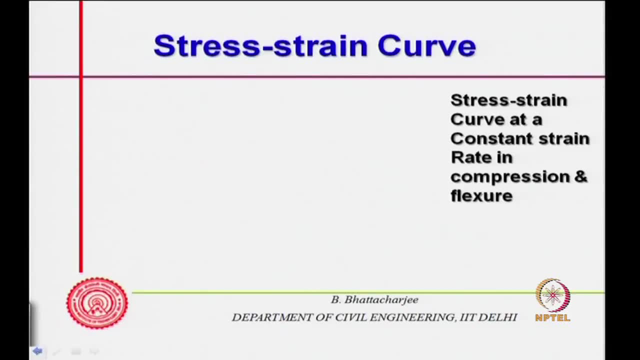 as 0.5.. So E is written can be written as 5000 under root. f, c, k is this for meant for design. So this is actually conservative value. In fact it will be something like this, you know, if I- I just I just plot it here before this, I just plot it here- it will be. 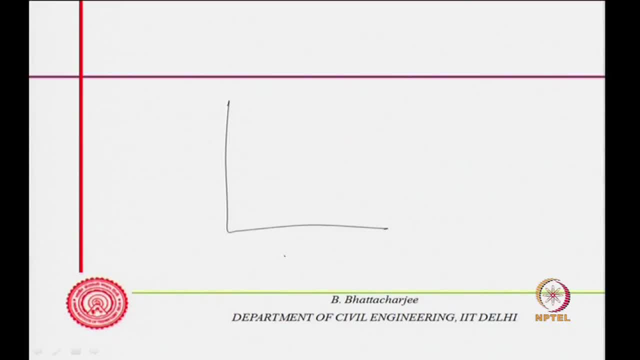 something like this. you know, if I plot f c in concrete cube strength and E then, or under root f c, then you get all sorts of scattered results and you can plot a curve. So this is what it is trying to do: linear curve, or some people p pity some m c to the power n. 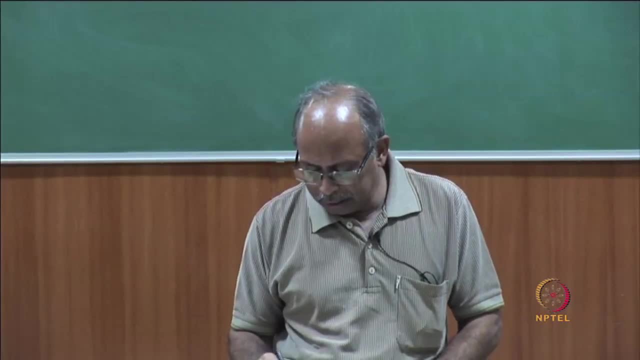 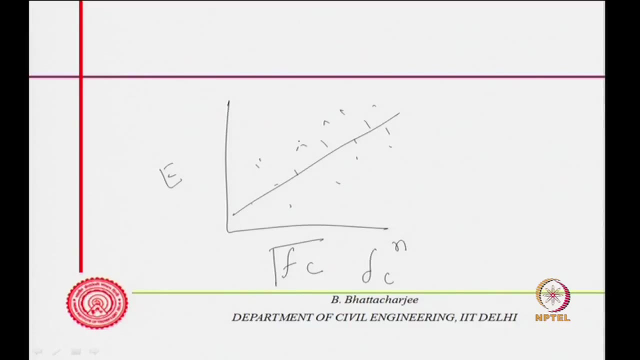 may be 0.6or whatever values are, and one can, because cứ is This is. you know, scatters are there. because it can, you can gift어�, it's just you canリ there. Now code would use a value of modulus of elasticity. The code, you know, the actual. 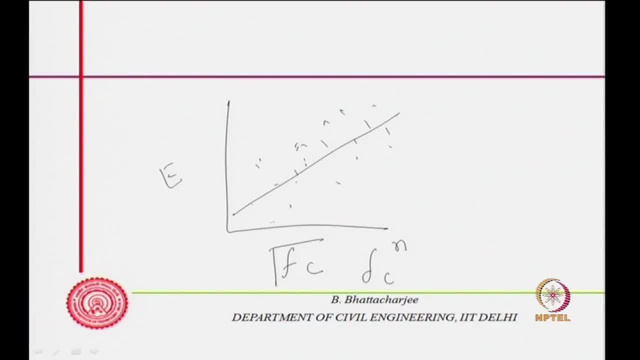 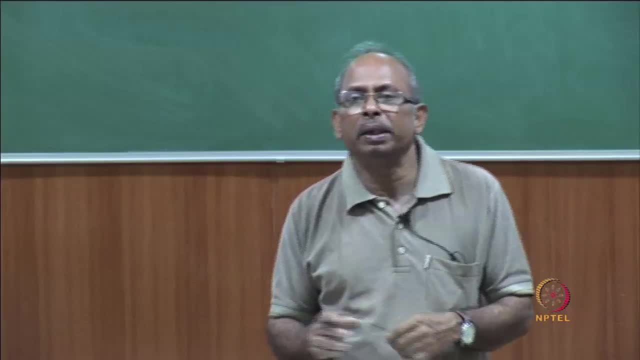 values will be there And the relationship that code tend to use is somewhere there – conservative value of e. It takes lower value of e because effects of creep, long term behavior. several other things comes into picture. So code takes this sort of stand actually Actual. 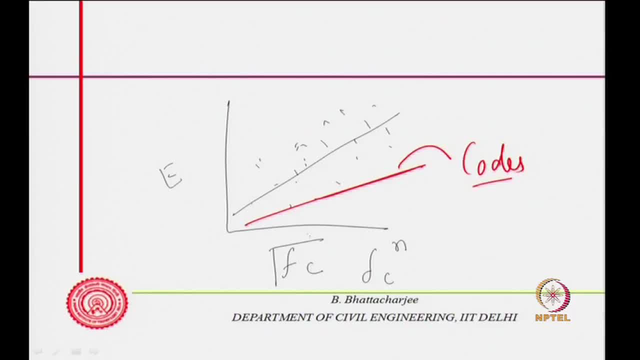 values could differ. Now, since this is, you know, under root f c, I said it can be f c to the power something else. So different codes may use different one. But I S 456 of course uses e is equals to 5000 under root f c, k. So you know the line is somewhere. 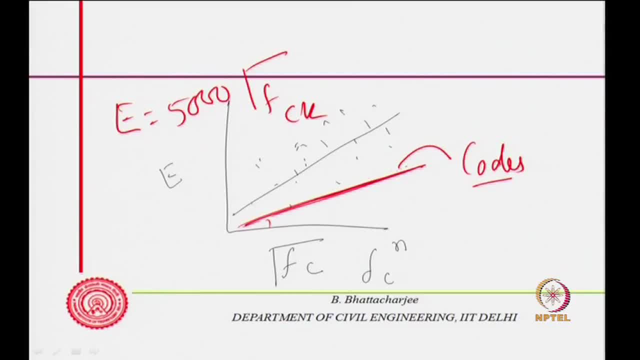 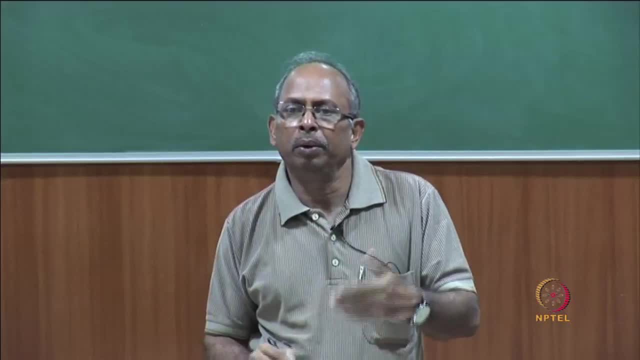 The slope is 5000 and under root f, c, k. That is what it uses somewhere down there, because it takes long time, behavior and other things into account And therefore try to use a conservative value. So that is it. That is related to what code? 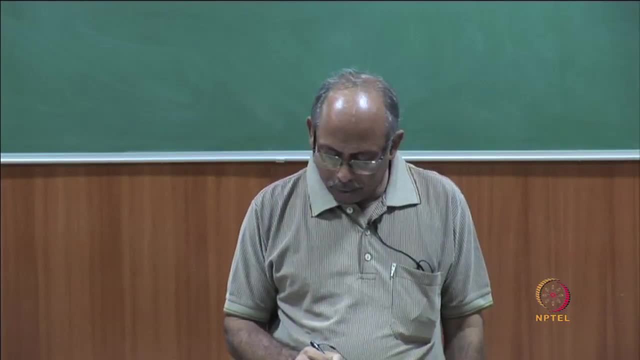 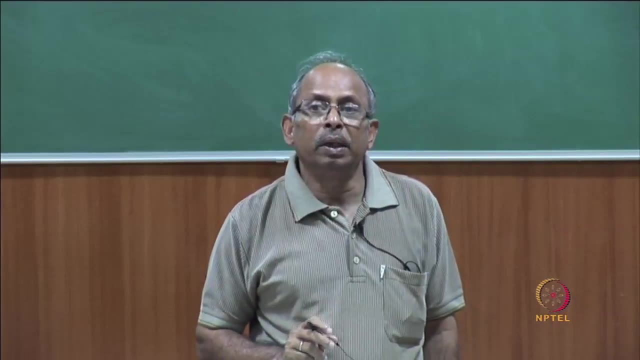 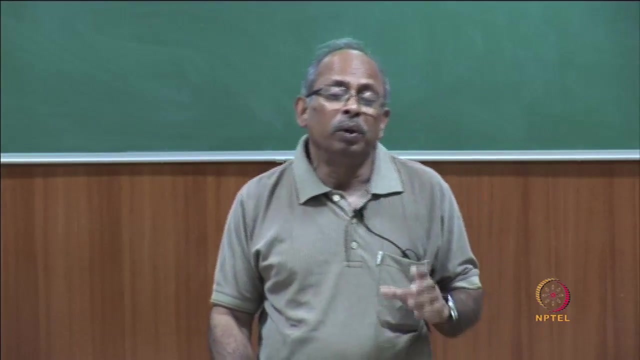 uses And it can be related to compressive strain. Now let us look into now stress-strain curve. If you look at stress-strain curve at a constant strain rate Now last class, last lecture, if you remember, we talked of constant rate of loading. Now you can do test by constant. 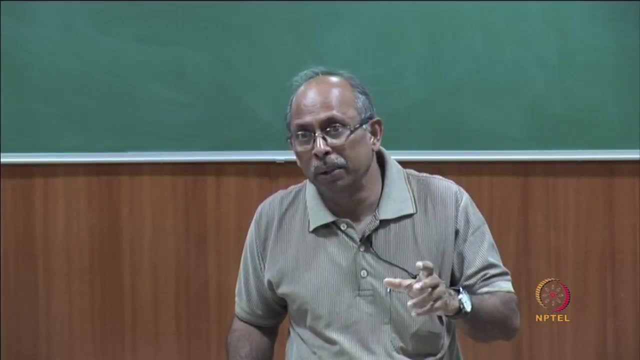 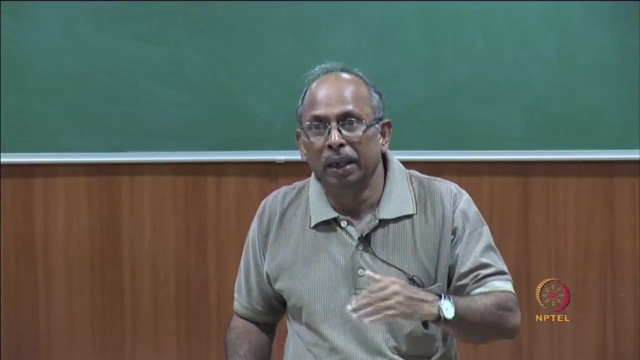 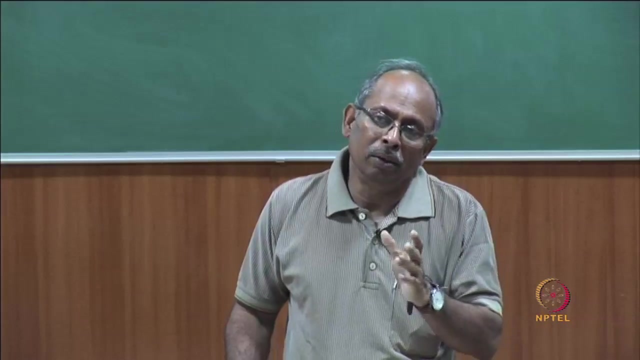 loading rate of loading. That means you apply load at a particular pace. Now you know 14 MPa per second. So you apply load at a constant rate And we have seen rate of loading actually changes the behavior. You know, like behavior changes. 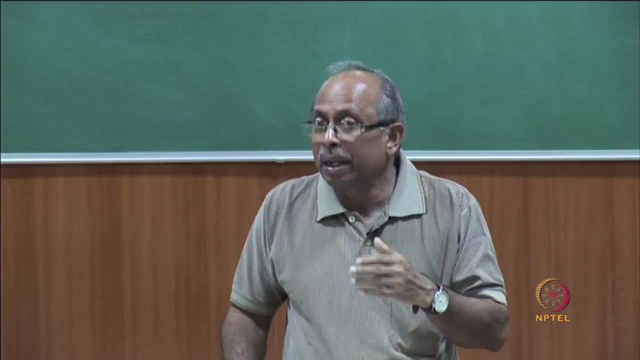 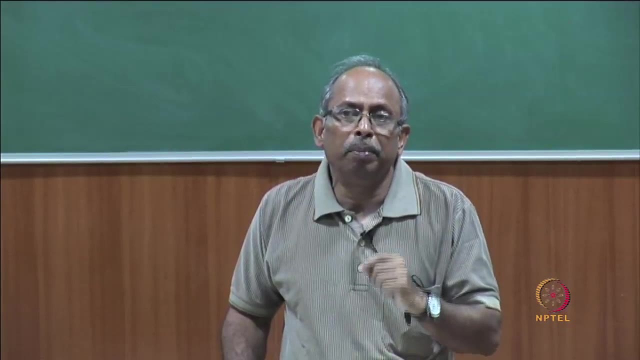 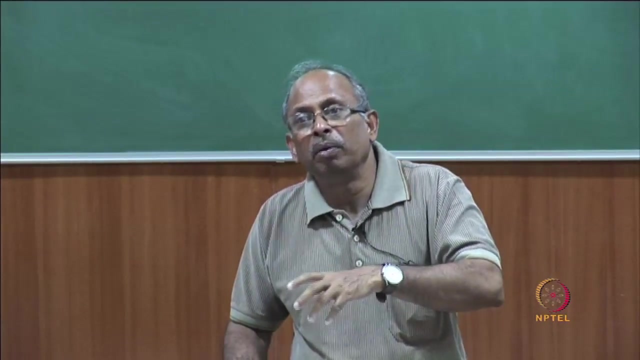 So supposing I apply Now, I can apply in terms of strain, at certain micro strain per second, some strain rate. So if I apply load at fixed strain rate- and I told you also that it is difficult to apply this- You need a machine which is capable of applying the 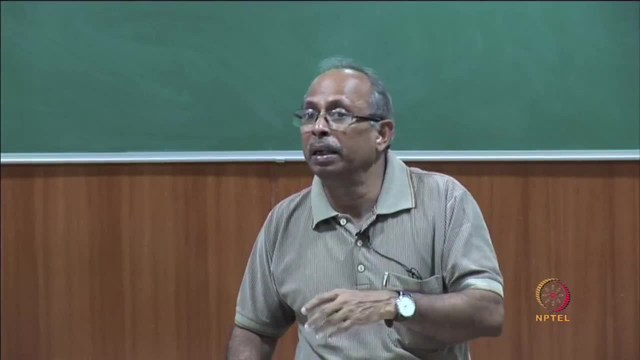 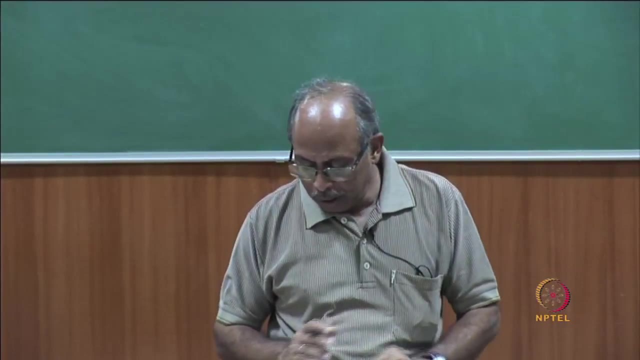 the servo controlled. It is capable of applying the maintaining the strain rate at a fixed rate whenever required, and that would require a controller and a servo control system and so on, so forth. So if you are applying load at a constant rate, you will find that depending 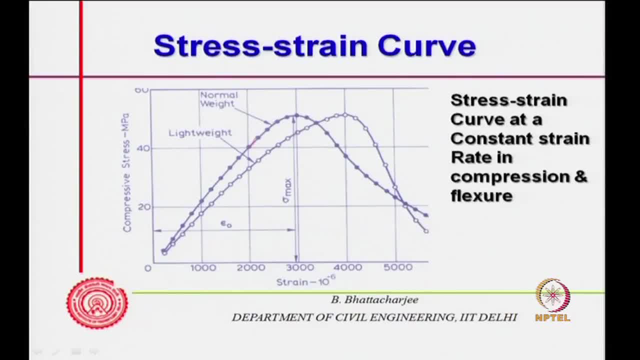 upon normal weight concrete behaves in this manner, while lightweight concrete shows this kind of behavior because you are able to now, since strain rate is there. So this portion of the current curves becomes available. and this behavior is similar in compression as well as in flexure: under compression, behavior in flexure. So you find some sort of behavior. 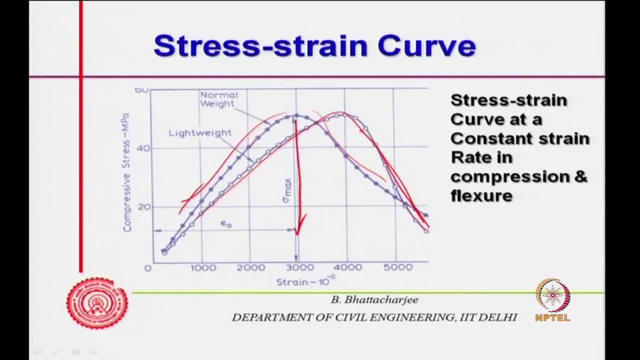 like this, where this is the E max, or rather F max or sigma max, maximum stress and corresponding to this we call as epsilon 0, that is the strain at maximum strain at maximum stress, strain at maximum For lightweight. this would be the maximum stress, sigma max and epsilon 0 would be this much So, epsilon 0 and sigma max, these are the 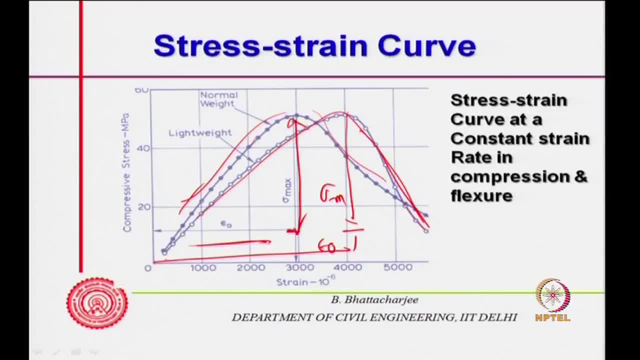 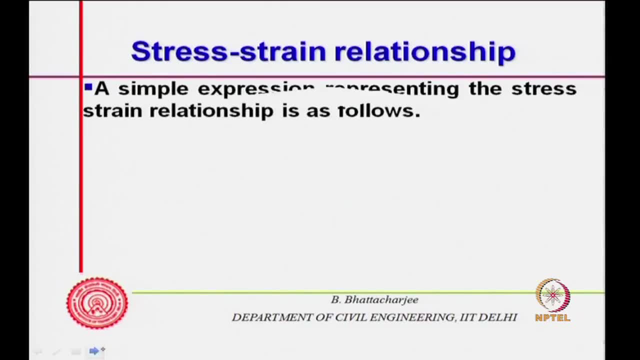 two ones, and you see this kind of a behavior. So people have tried to fit it, approximate equations to this, empirical equations to this and this, empirical equations that have you know, representing this, the simplest. There may be many more complex relationship, but one of the simplest relationship is of 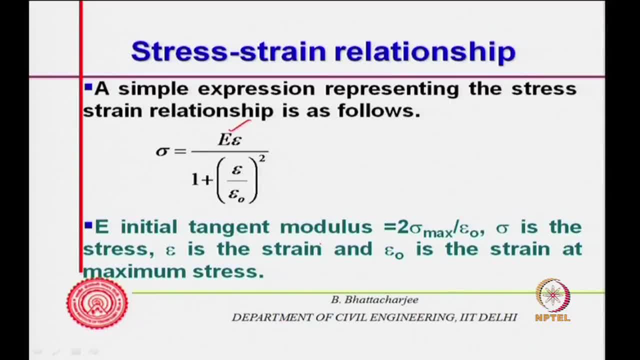 this form, where E is the initial tangent modulus, and you know it is, which is twice sigma max divided by epsilon 0, and sigma is the stress at any point, epsilon is the strain at any point, epsilon 0 is the strain at maximum stress. So epsilon 0 is strain at the maximum stress. So this sort of formulae: 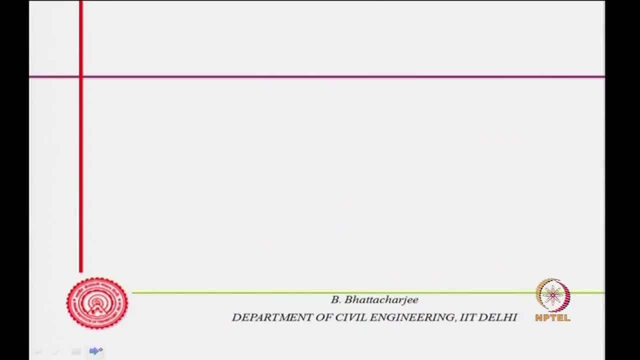 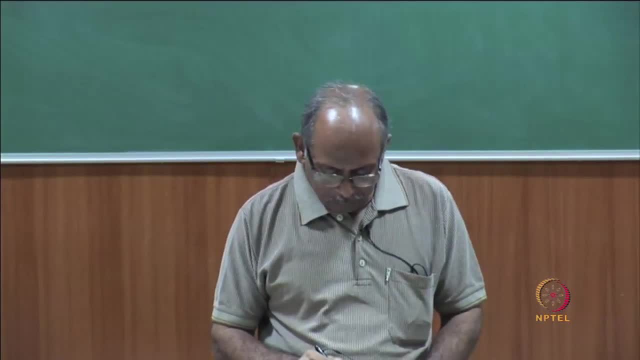 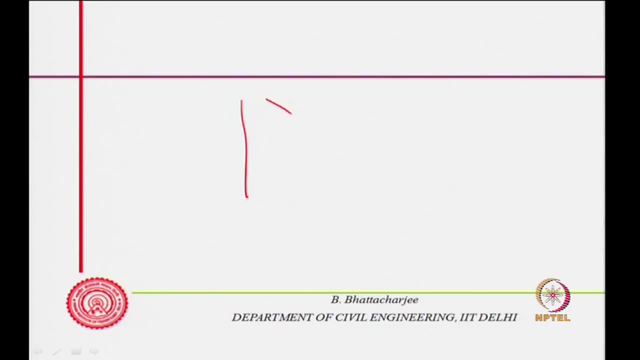 is available through which you can define the stress strain curve, and there are complex formulae also available. So, what is the stress strain curve of concrete? Now we actually- if you just before I go to this- in flexural design. therefore, one should be using this sort of curve in compression. 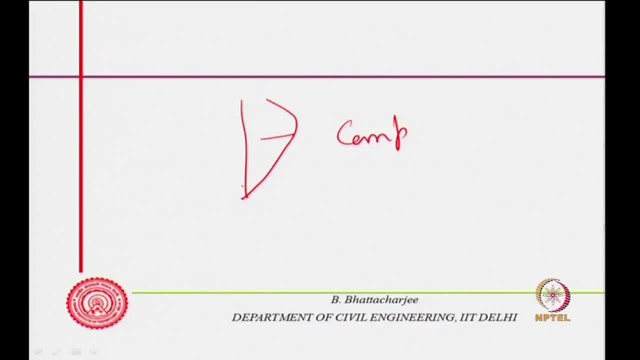 compression, you know. So this is, if you remember, flexural design, flexural stress strain curve given in the code. stress strain curve given in the code would be something like this: You know: stress concretely of to the mass, it should be 1.5 or 1.15 in scale. 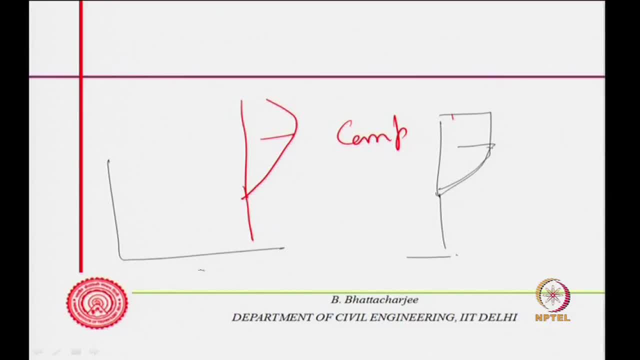 complete stress strain curve of concrete. If you recollect this is strain Inflexor, you know if it is a beam, section of a beam, If I am looking at a section of a beam, this is a steel reinforcement, this is a concrete Anyway. so stress strain curve will be like: 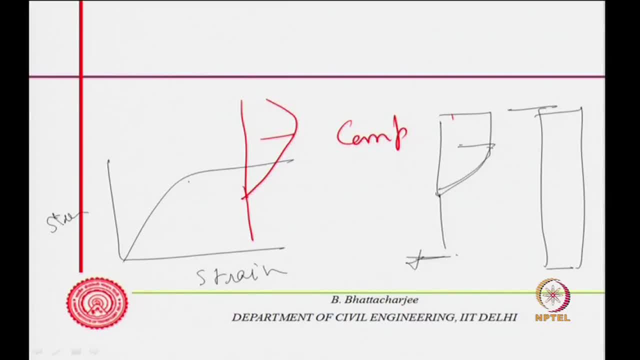 this stress versus strain curve. If you have seen idealized stress strain curve, it will be 0.002 here and 0.0035 stress strain curve And this is actually, you know, F, c or whatever you call it, the stress maximum failure stress. Now, this is an idealized stress strain curve. 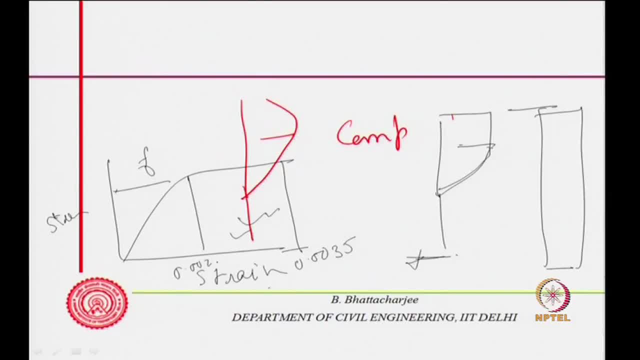 idealized stress strain curve. idealized stress strain curve of concrete. In fact, stress strain curve of concrete should look like. should look like something of this kind. you know some stress strain curve of concrete will look like. let me draw it with a red. 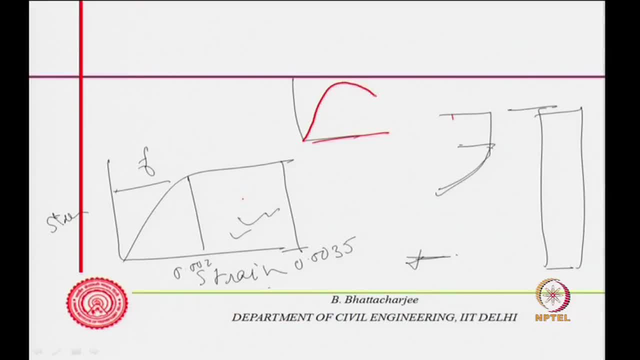 color Stress strain curve of concrete will look like this: alright, maximum stress. and here Now this is idealized stress strain curve Beyond that you assume is as if it is straight line. So actual stress strain curve of concrete is like this, and this is important in flexural design. So the measured stress strain curve. 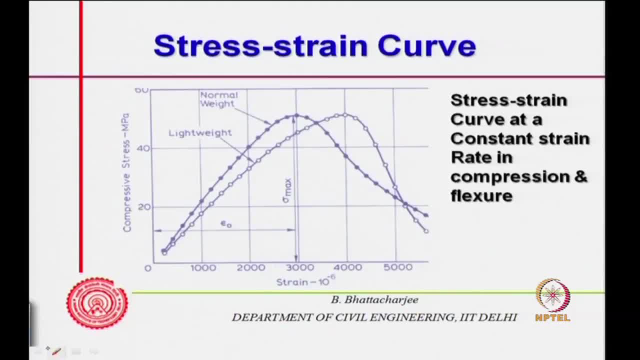 that we have seen, you know, measured stress strain curve, actual stress strain curve observed, as we have seen. this is idealized into this sort of a straight line curve And of course, this line factors are applied to bring down the load as well. that I am not discussing. 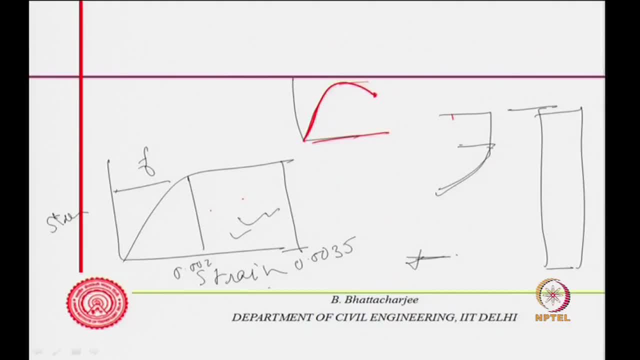 at the moment. So this importance of the stress strain curve is here because in flexural design we have got to use this. So idealized curve is something of this kind. this is arrived from this real behavior. this is arrived from this real behavior. 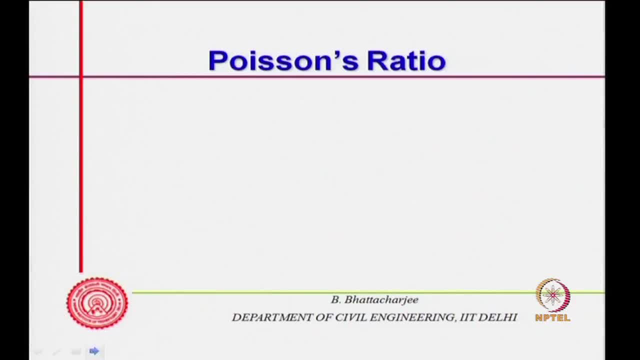 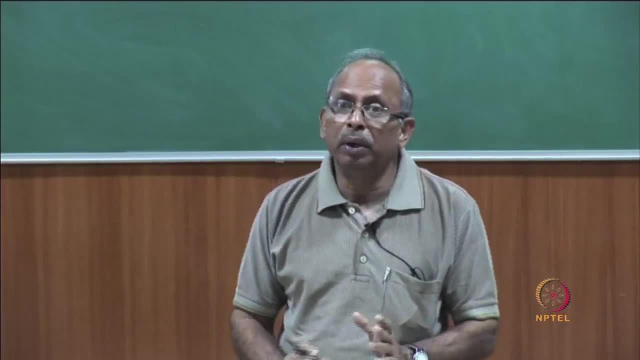 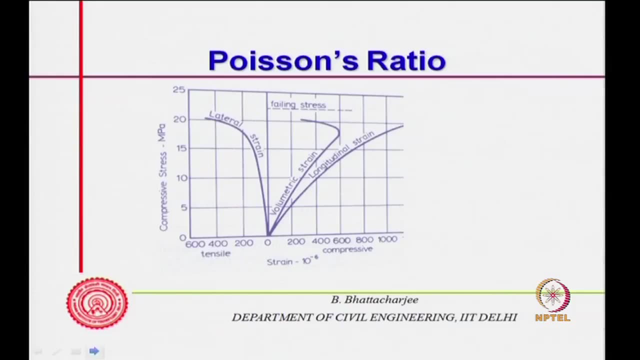 So that is the importance of the stress strain curve. Now let us look at next property, which is portion's ratio. This is important to find out: lateral deformation when you have applied a longitudinal stress right in axial situation, and so on. So therefore, if you apply load when you 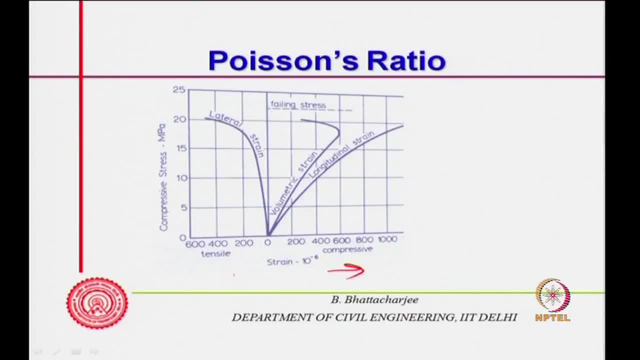 apply load. you know, you can see, this is compressive loading, this is tensile, the strains are here and this is compressive stress. So what happens is this is a longitudinal strain, this is the volumetric strain. that is what we talked about earlier, that you 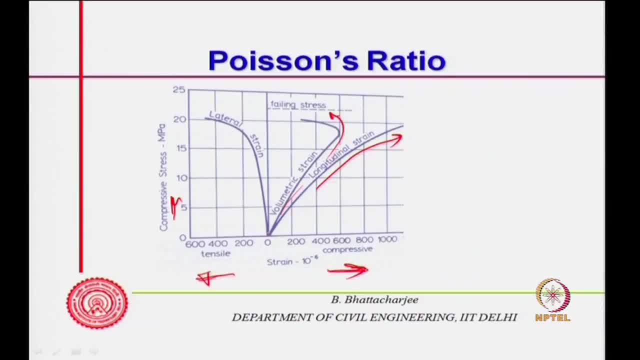 know when we talked of ultrasound pulse velocity and acoustic emission, and this is the lateral strain which is in the opposite direction. it is in the tensile direction. So mu is defined as lateral by longitudinal strain. So this is lateral by longitudinal strain. 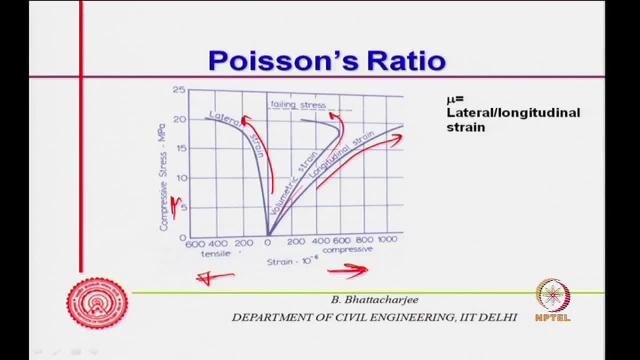 mu is defined by this actually. So from this, if you try to calculate out the mean, you know ratio of, for example, this divided by this ratio. you know this divided by this ratio. all right, or let us say at 400 strain of longitudinal strain corresponding to this: 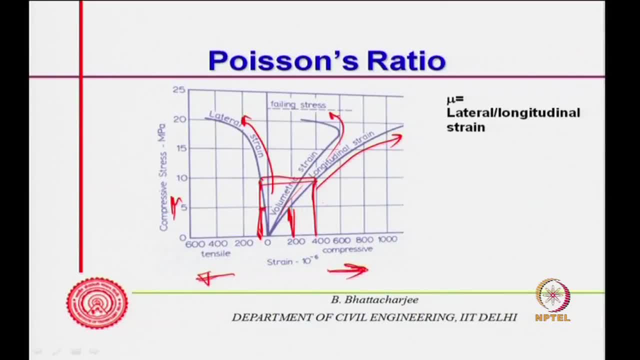 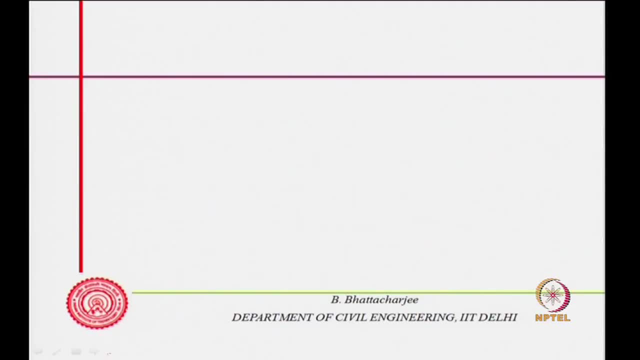 is, may be whatever the value is, and similarly, you know, so you can, You can, you can actually find out the mu values. Now, mu values: if we calculate out in this manner and then plot, we will see that it is roughly around 0.2,. it is roughly. 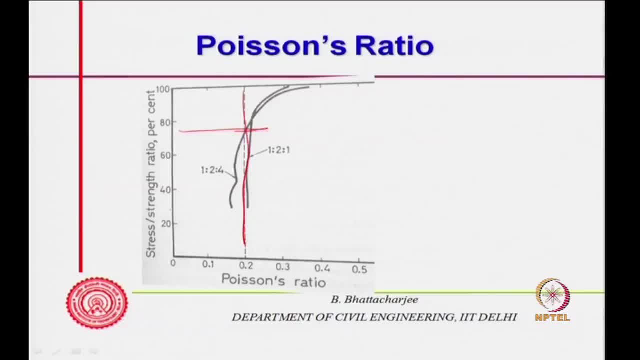 around 0.2, up to about 70 percent of the load. for two different concrete good old days, people conducted experiments and found out. But beyond that point actually it starts increasing. it starts increasing, can go close to about 0.3, 0.5, 0.5, 0.5, 0.5, 0.5, 0.5,. 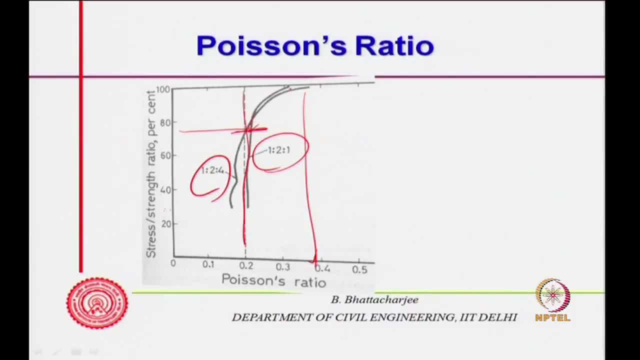 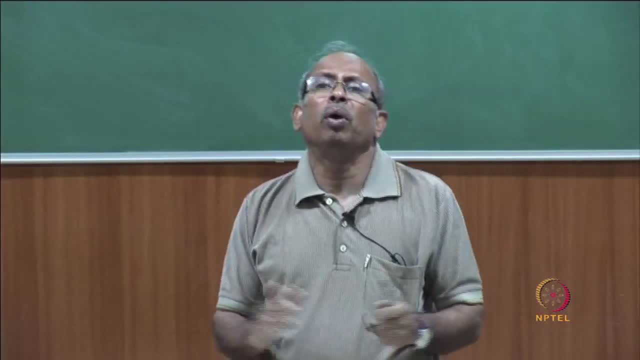 0.4 or so on and so forth. if you know, like, if you stress, stress to strength ratio. So we are before failure, percentage ratio increases and we understand this, because lot of microcracking would have occurred. lot of microcracking would have occurred. 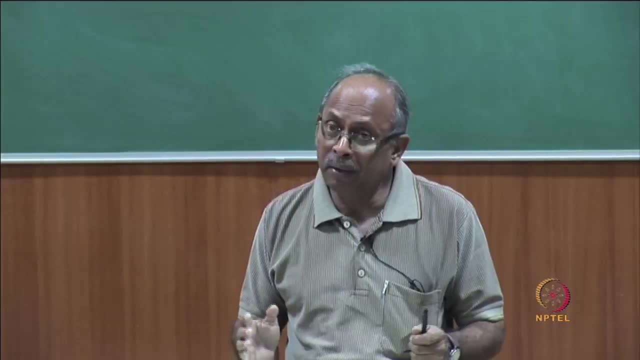 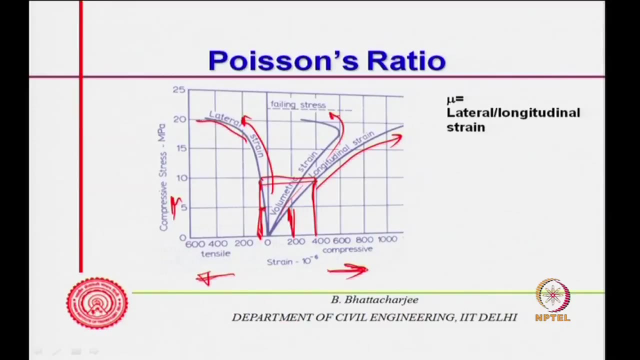 and that would have caused lateral strain to expand. you know, increase at a faster rate than the longitudinal strain And this is manifested here also. this is manifested in this diagram also. Suddenly there is a lateral strain increasing, not you know. 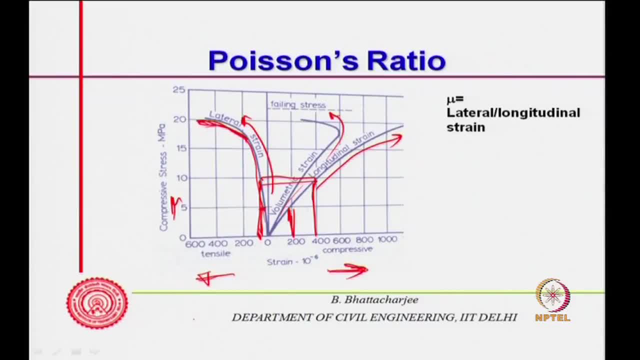 here it was increasing in slow manner but it was increasing increase started increasing in a faster manner. While this is increases- although although there is a faster increase here- I mean you know this is this is not really- it is almost close to linear sort of situation. slight variations are there, but 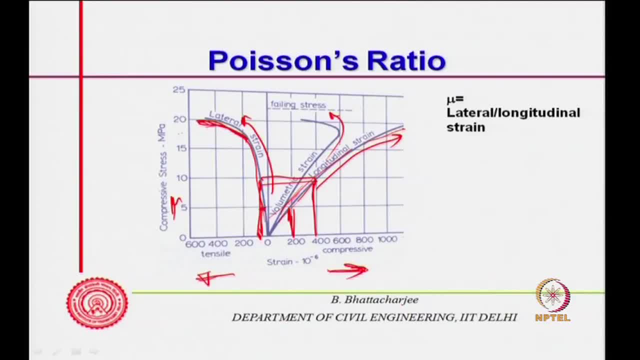 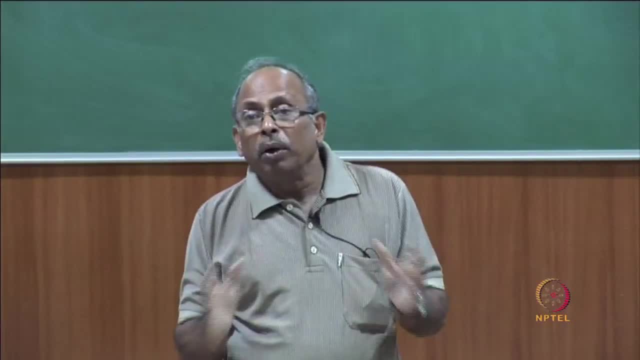 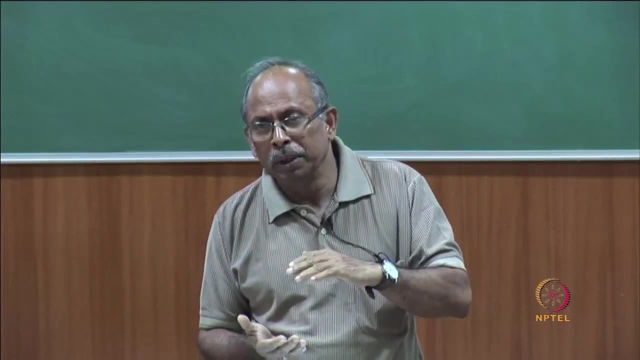 this increases at a very fast rate. this increases at a fast rate, but this increases still at a faster rate. And this we can understand from the physical scenario, because micro cracking in the would would result in lot of transverse deformation. Longitudinal deformation also would be there, but lateral deformation will increase significantly. 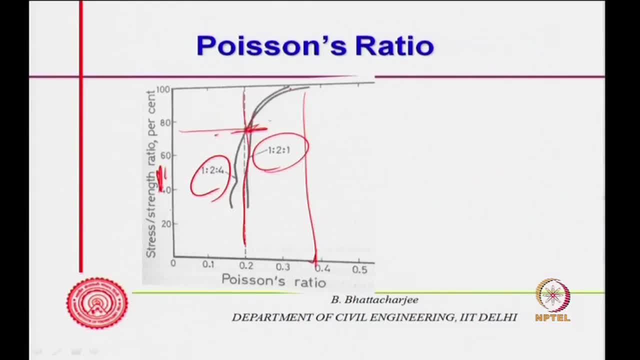 because of the micro cracking. So beyond 70 percent of the load. actually, your Poisson's ratio increases significantly and you know, up to its constant, almost constant, up to 70 percent of the strength, 70 percent of the strength, 70 percent of the strength Generally. 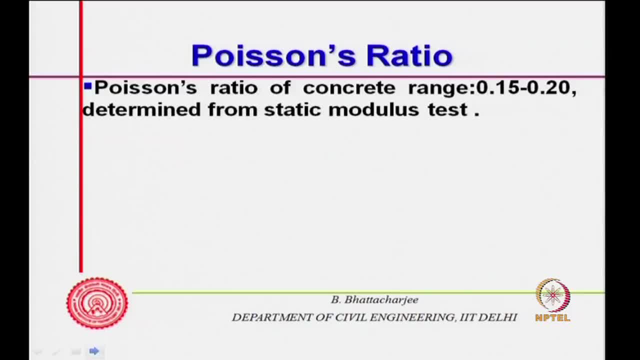 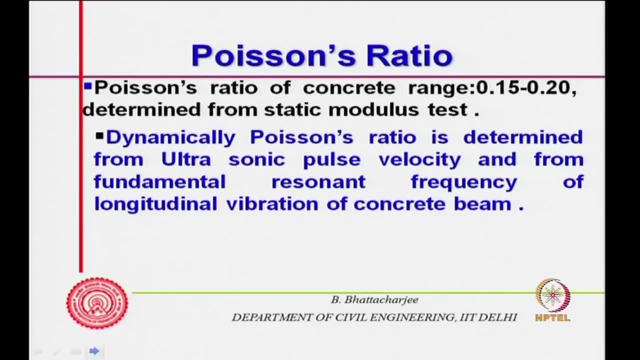 it varies in the range of 0.15 to 0.20. that is what you see determined from static modulus test test. But you can determine dynamically Poisson's ratio also from ultrasonic pulse velocity test from fundamental or, or you know, sonic velocity test from fundamental resonant frequency of longitudinal vibration. 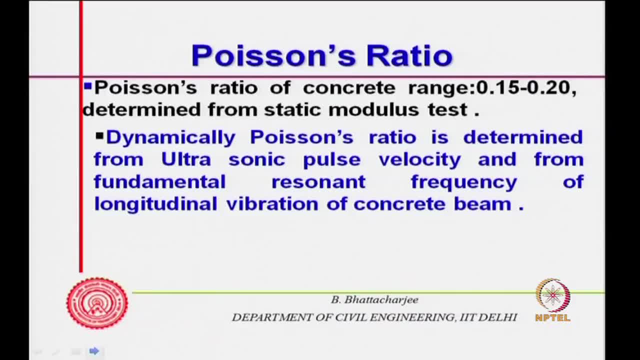 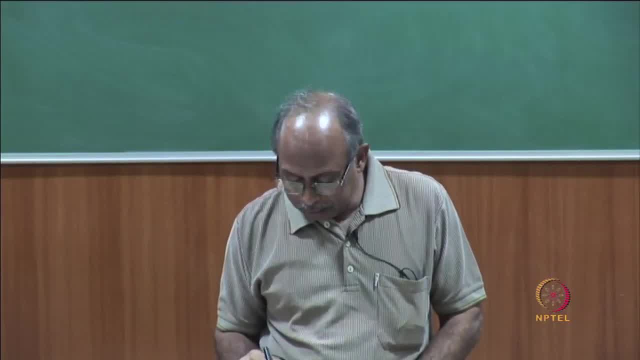 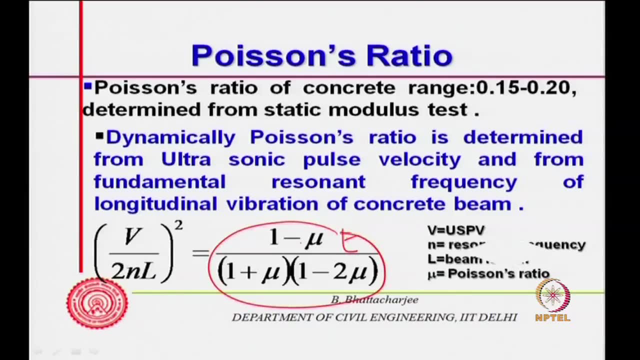 of concrete beam, similar test that we did for modulus of elasticity. Now, how do you determine this? how do you determine this? actually, because the bulk modulus- you know it was related to bulk modulus. So this is the relationship between the. You know this is involved in the velocity equation. The Young's modulus is related. 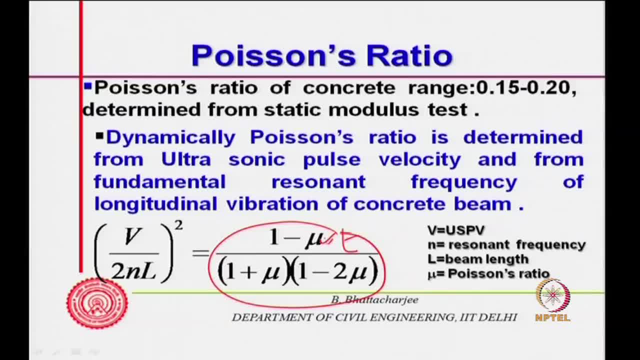 to the Bunk's bulk modulus in this manner, where mu is the Poisson's ratio, So velocity, frequency length, and it is related to modulus of you know, Poisson's ratio is related to that. So this is the velocity, pulse velocity, resonant frequency, beam length and Poisson's. 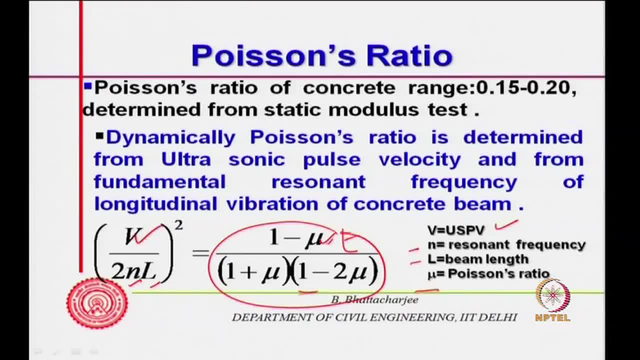 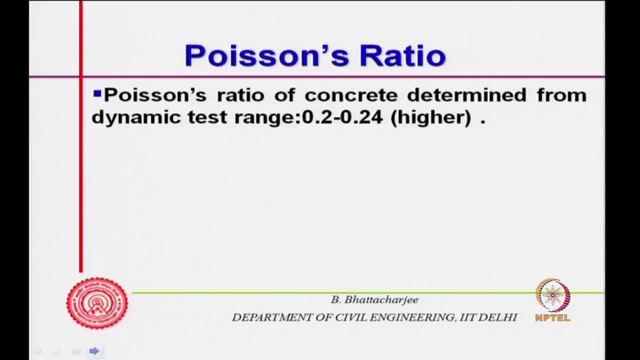 ratio. from that one can find out. So from dynamic testing also you can find out Poisson's ratio. And generally dynamic modulus again gives you higher value of Poisson's ratio, because you know higher value of Poisson's ratio is usually 0.2 to 0.24.. And higher the. 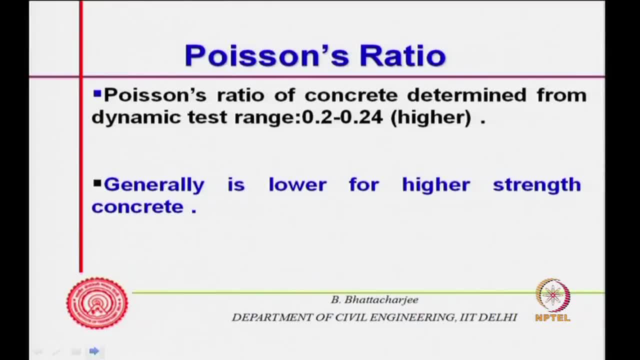 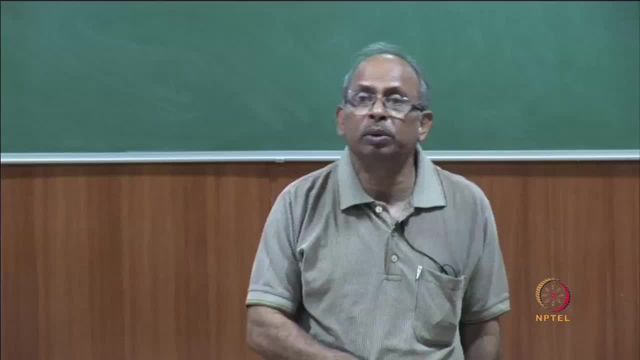 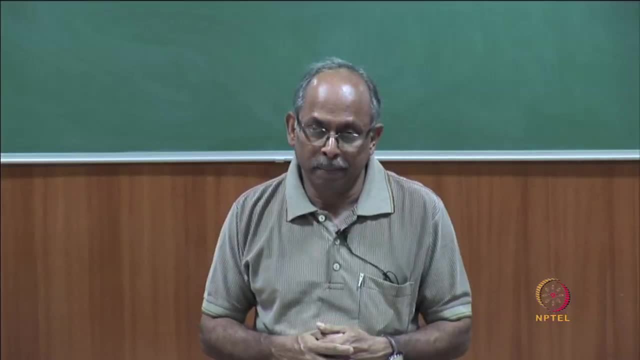 strength of concrete Poisson's ratio is lower. Higher, the strength of concrete Poisson's ratio is lower. So that is right. So this is related to Poisson's ratio. Now let us look at another mechanical properties called fatigue. You know fatigue is related to reversal of stresses And you can understand. 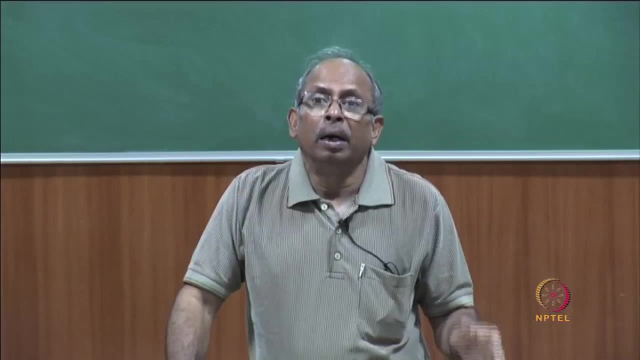 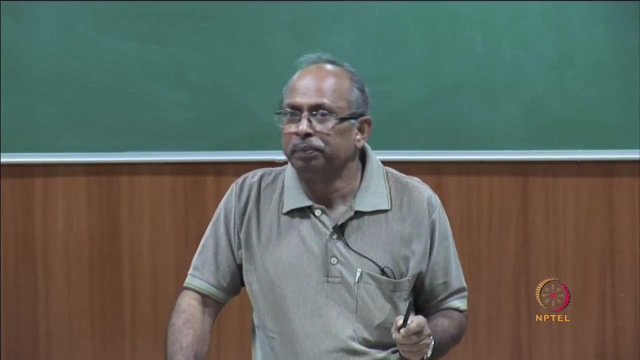 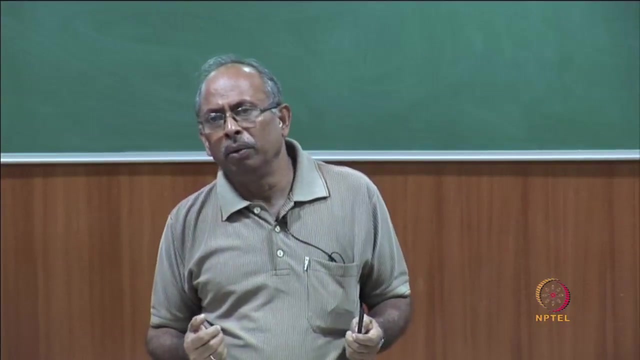 the importance of this one in many structures, The load that is applied in most of the structure, the imposed load that is actually quasi-static, But that we do not call it fatigue, You know like, because even in a building where you are sitting, let us say right now, if it. 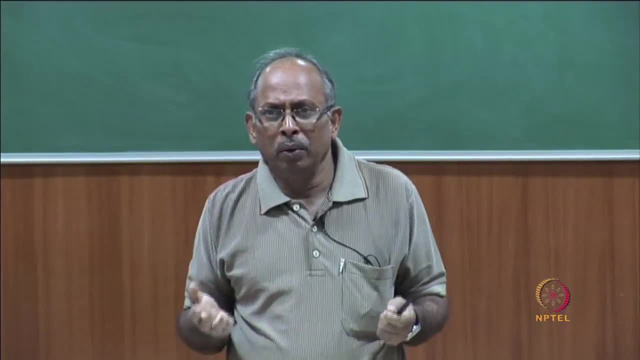 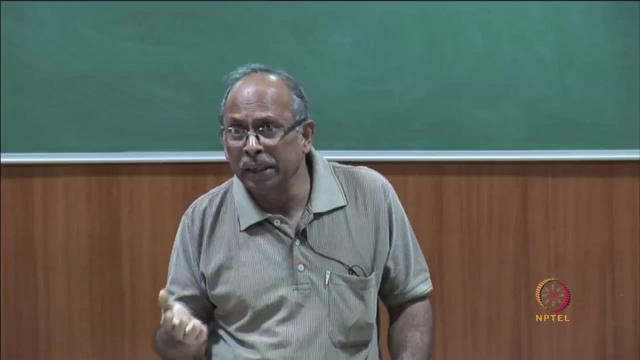 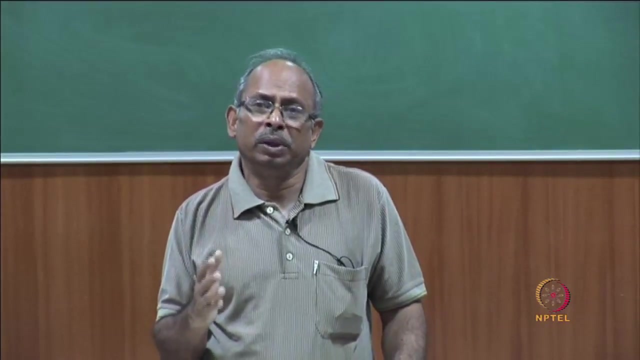 is on the first floor, or you know, in the higher floor other than ground floor, the slab that you are actually sitting on or your chairs are the load. you are coming and then you are going out. So there is a kind of stresses. It is quasi-static, actually. What? 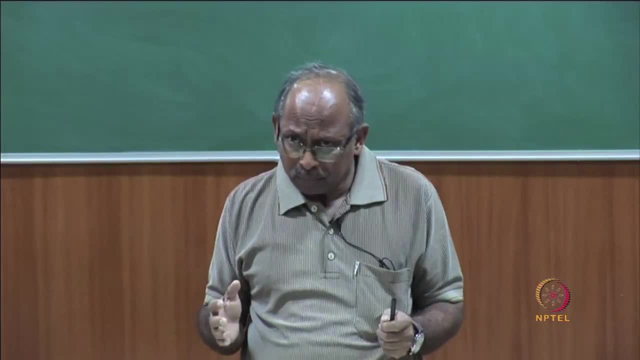 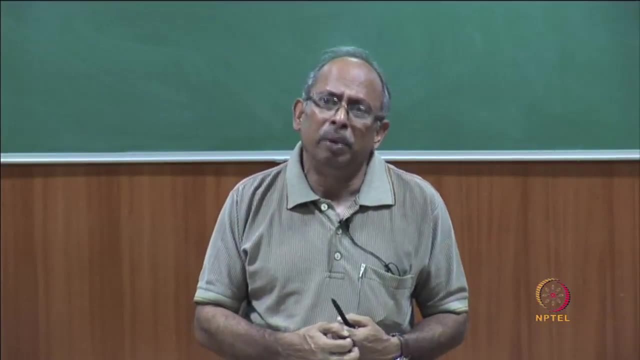 happens is by and large we assume that to be static, because major load will come from the permanent fixtures such as furnitures and things like that. the imposed load- Human contribution is- will be relatively less. So we assume it to be practically you know. 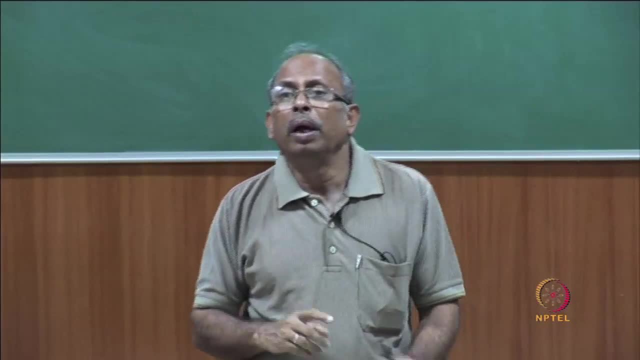 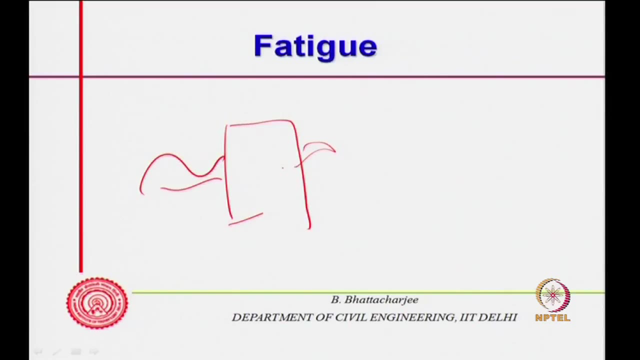 static, So fatigue is not there. But supposing it is a bridge, or assume a structure in marine environment where waves comes and hits- here waves comes and hits, you know waves comes and hits, So it is actually under kind of a reversal of stresses would be occurring. 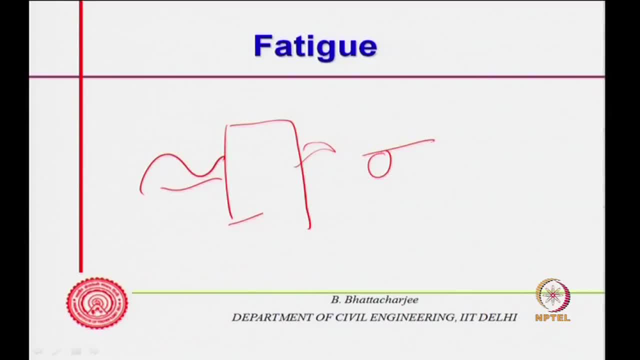 Bridges – this is vehicular load. comes in vehicular load, comes onto the you know vehicular load. It comes onto vehicular load, comes onto a bridge deck and then it moves, bridge deck and then it moves. So therefore, this is: there is a reversal of stresses there, reversal. 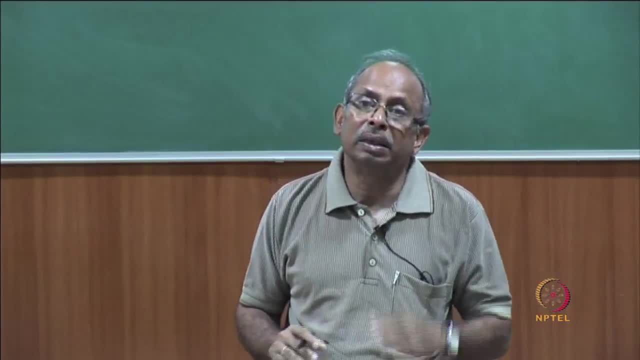 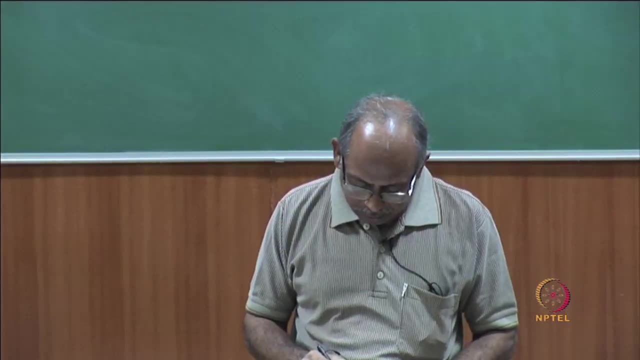 of stresses, you know, onto the deck. So, therefore, this reversal of stresses is related to what is called fatigue strength. Reversal of stresses is related to fatigue strength. So let us see, And in fact, the load one, any structure or any structural element can: 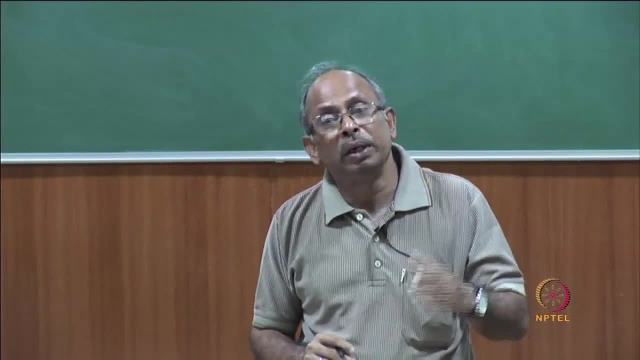 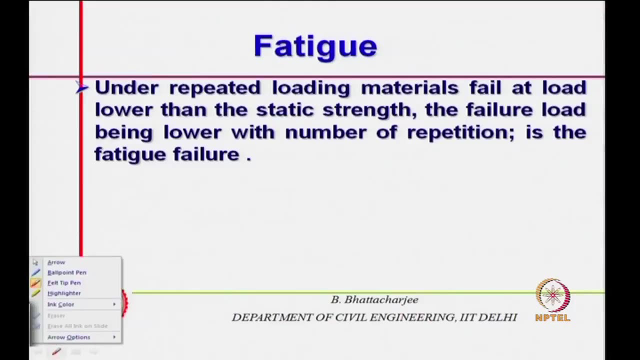 carry, under reversal of stresses, much lower than the load it can carry in static conditions. So fatigue is related to… Repeated loading – under repeated loading. under repeated loading, materials fail at load lower than static strength. the fall load failure, load being lower with number. 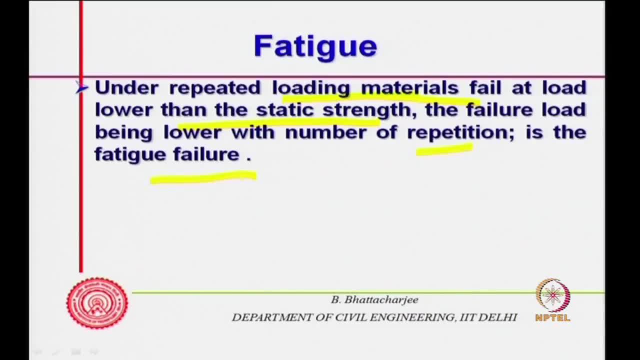 of repetition and it is a fatigue failure. A simple example is given. Supposing I have a wire- small wire- and I try to pull it, it will, I can never break it. You know binding wire which are used for binding the steel in concrete while casting concrete. But 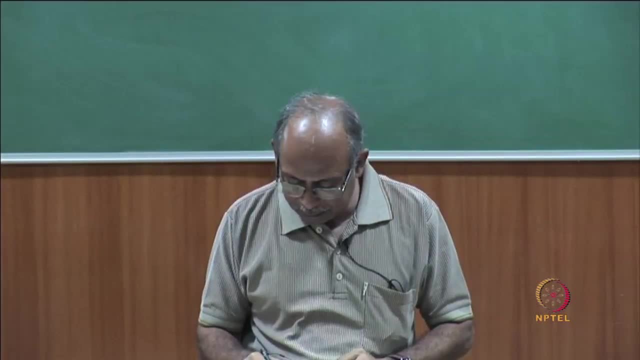 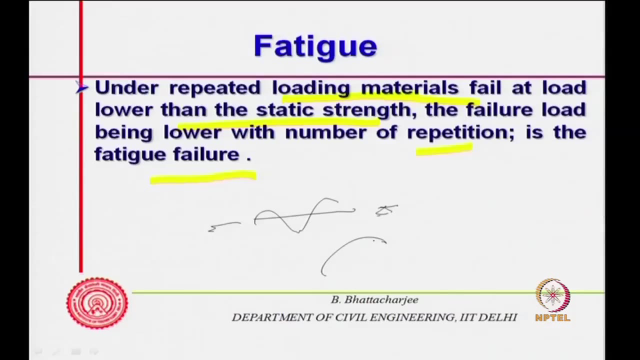 if I try to bend it in this manner, that means bend it in this manner. bend it in this manner, you know reverses the stress. There is a reversal of stresses, So you bend. first you bend it in this manner, then bend in the reverse direction. So first you bend in this. 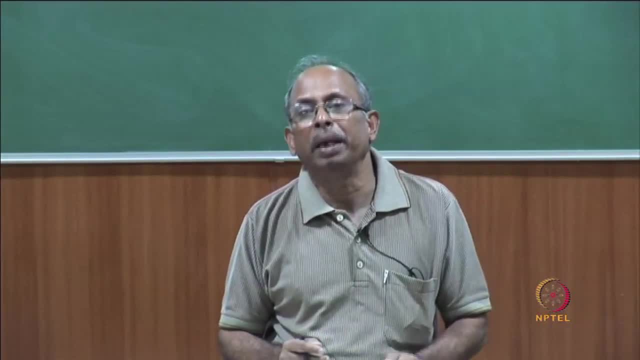 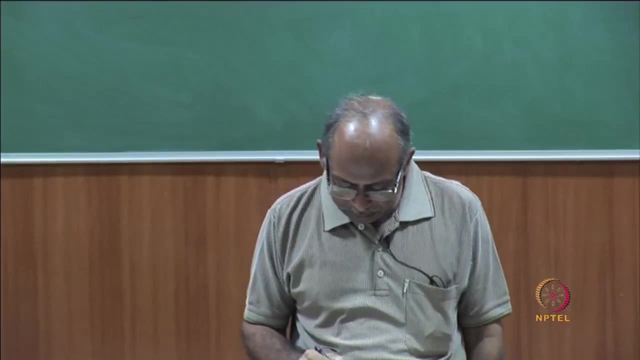 manner, then reverse direction. You go on doing this. after sometime it will break. So repeated loading you can. you know it fails at much lower load, much lower load, and that is basically much lower load and that is basically a fatigue failure. Therefore, 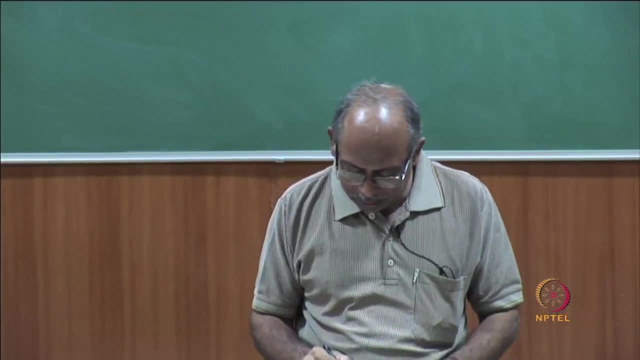 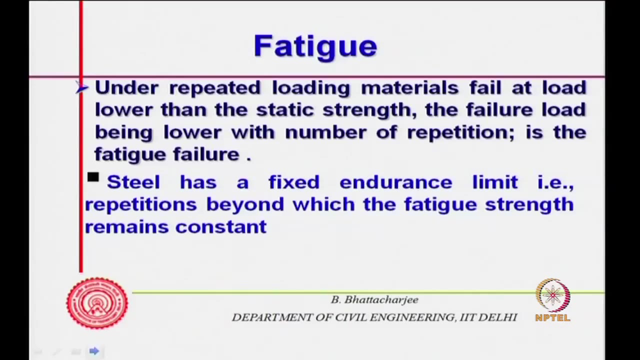 fatigue failure occurs at much lower load. So the mechanism, you know that is what is a, you know that is what we define as fatigue and let us see how what happens in case of concrete. Now, steel has an interesting behavior. We. define something called N D O. What happens is, as you go on number of repetition, you know if you apply a load, say load which is 50 percent of the strength, and then apply reverse, the stresses may be bring it to 0,. 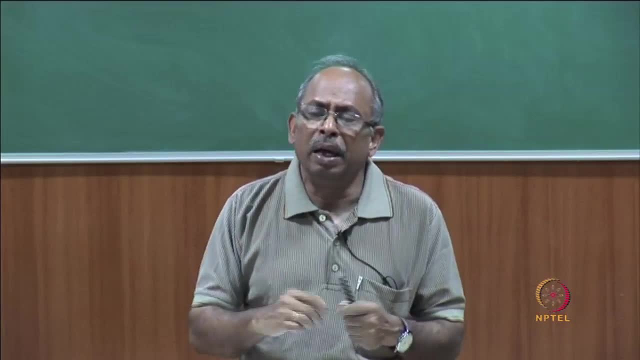 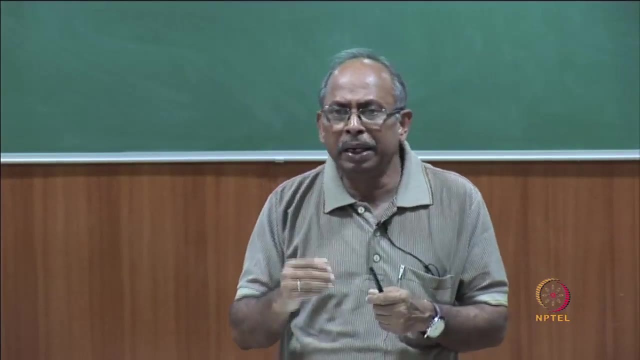 some reversal, bring it to 0,, take it to 100, near 100 percent. Number of, number, of, number of, I mean one thing: the amplitude, you know, or the maximum stress positive and the negative Or maximum stress positive and the negative Or maximum stress positive. So the maximum reversal range, range of the stress, range in which it is reversing. Let us say we keep it fixed. Now, after a certain period of time we will find that it fails. Now, if you lower the load, if you lower the range in which you are operating, then it 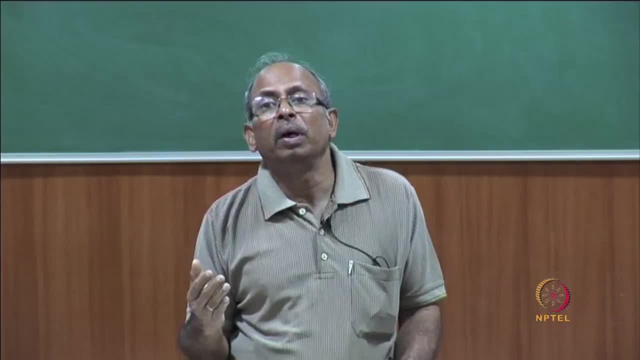 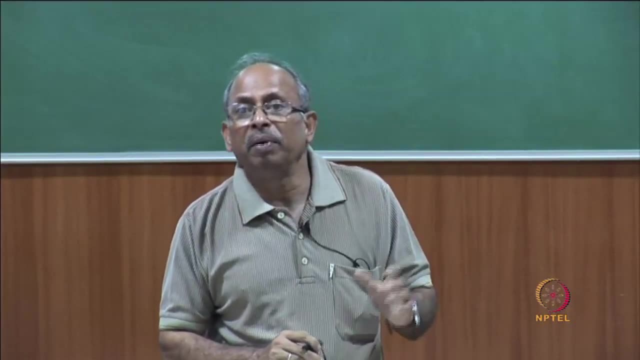 will take longer. more number of cycles. So the number of cycles is a function of number. the number of cycles is a function of number of cycle is a functional level of the stress. you know reversal: where you are, reversal of the stress is occurring. 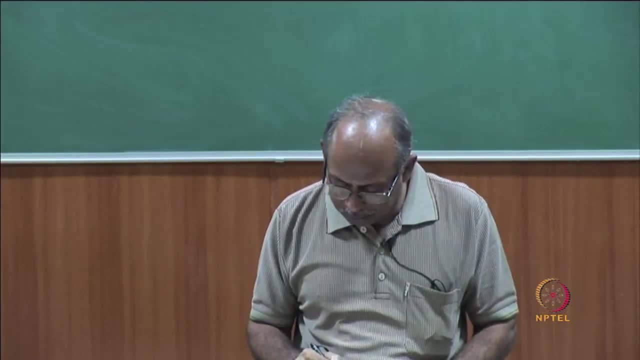 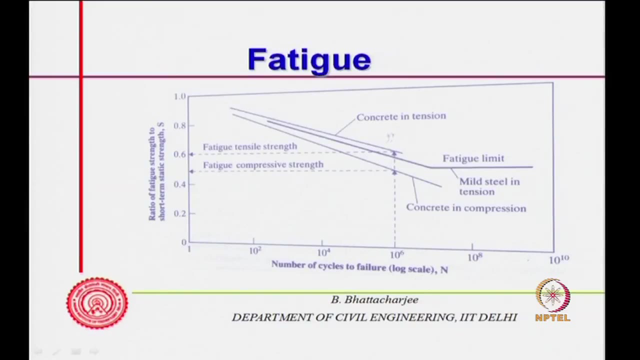 Now, endurance limit is defined in this manner. it is much better to define this and we come back to this. if you look at this diagram on this axis: number of cycles drawn in log scale. drawn in log scale because 10 to the power, 2, etcetera. this is in log scale and ratio. 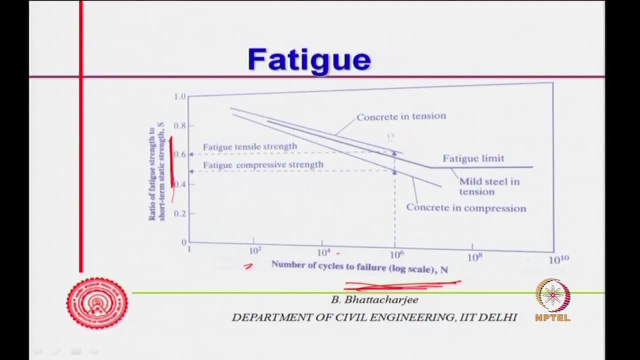 of the fatigue strength to short term static strength, fatigue strength to short term static strength. So actually, if you are operating at you know fatigue strength, you will find that in case of steel, this is mild steel. in tension you do reversal of stresses, but beyond. 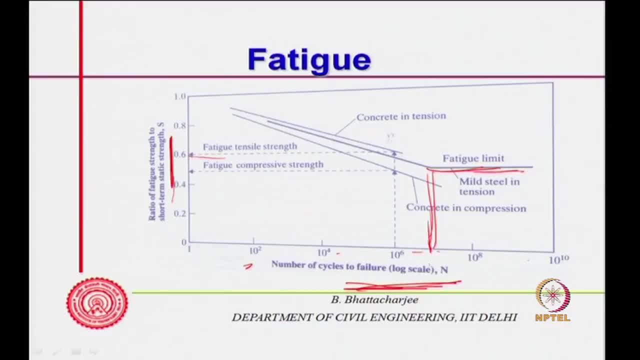 10 to the power, 7 cycle or some such cycle slightly above 10 to the power, 10 to the power, 6 cycles and 7 cycles. you know the endurance, the fatigue, the load at which reversal this is occurring at 0.4 or so 0.4 or so close to 0.4.. So close to 0.4.. So around, you know. like 250 MPa is a yield strength of mild steel if endurance limit is around 100 MPa, close to 100 MPa. So that means if you apply less than you know 100 MPa and do stress reversal, actually it is not going to fail Now endurance limit. 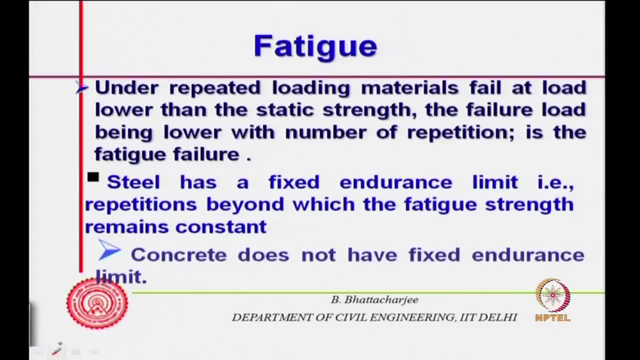 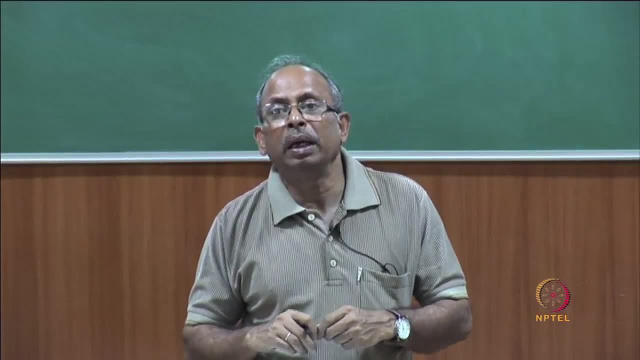 is defined. therefore, endurance limit is defined as as fixed endurance limit, that is, repetition beyond which the fatigue strength remains constant. So what is fatigue strength? fatigue strength is the number of repetition or the strength which you know it can withstand at certain number of repetition. So it is related to both repetition and the level of the strength. 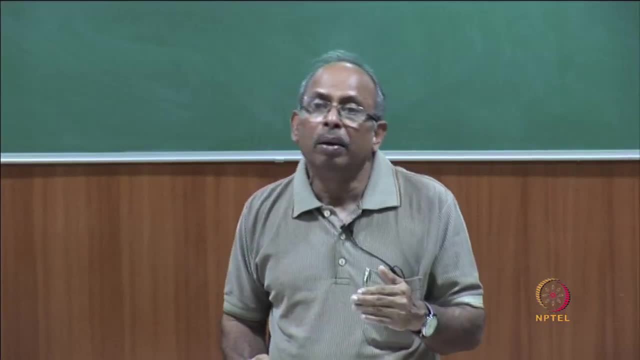 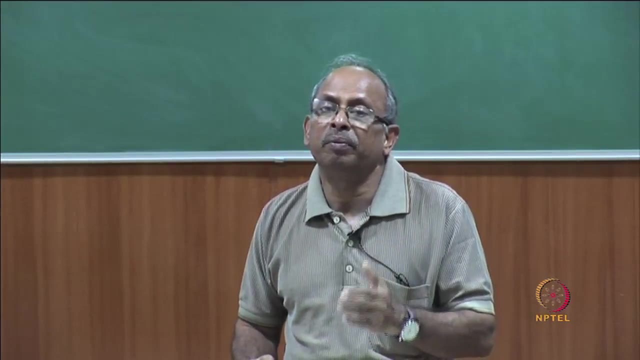 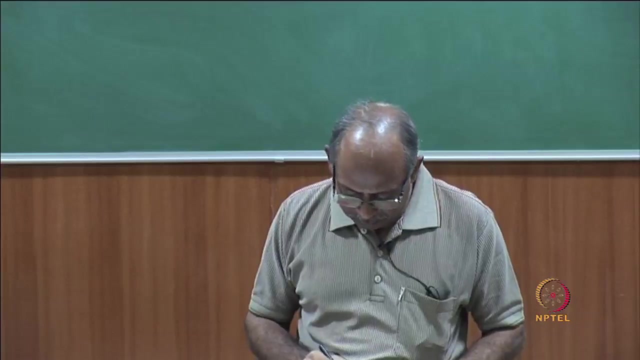 Now, endurance limit is that level of the strength beyond which, actually, lower than that strength, it can withstand large number of repetitions, you know, because fatigue strength becomes almost constant. Now, concrete does not have a fixed endurance limit. concrete does not have any fixed endurance limit. concrete does not have any fixed endurance limit in 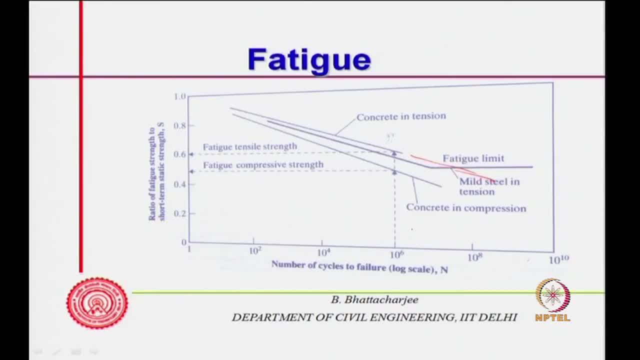 tension, concrete in tension. it shows continuously. if you the, you know the first, fatigue strength will go on. So by increasing as we increase the number of cycles. So here also, concrete in compression, same thing. So therefore, how do I define this strength? there is not endurance limit. 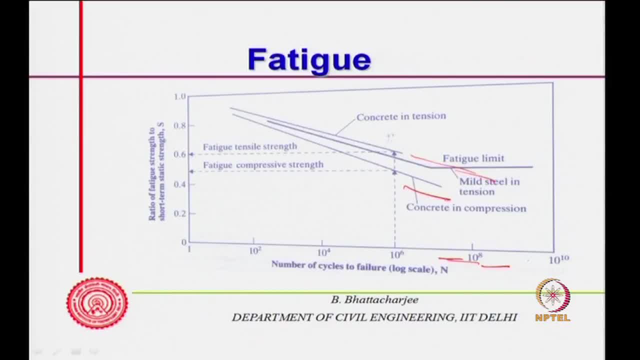 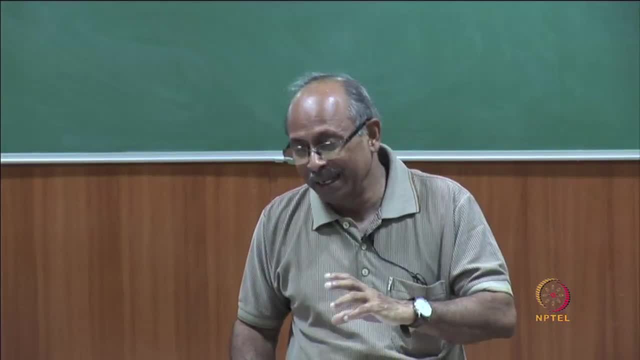 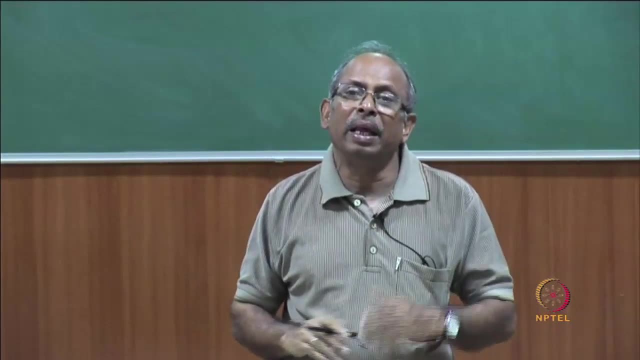 how do I define the same endurance limit? So thus, you know, steel is advantageous in that sense, from usefulness point of view. I mean what I say. it design, calculation point of view or understanding point of view, because you have got a fixed endurance limit. So therefore, if you know it is likely to, 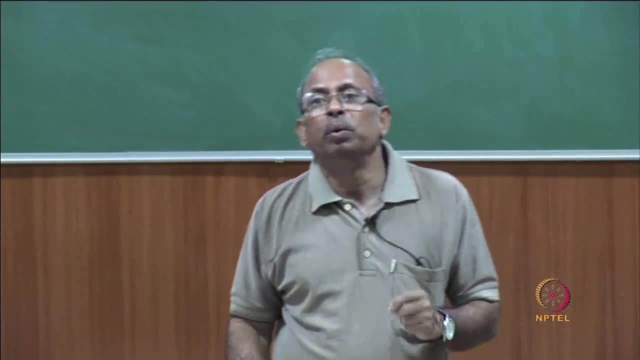 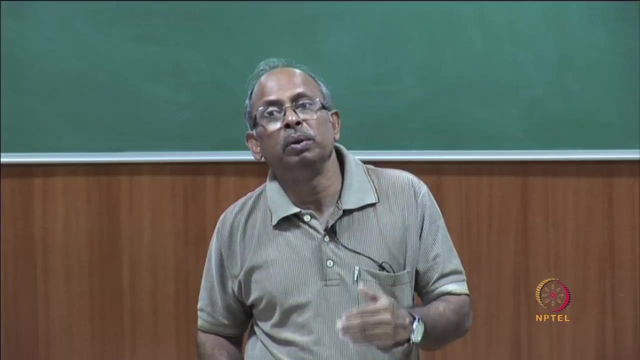 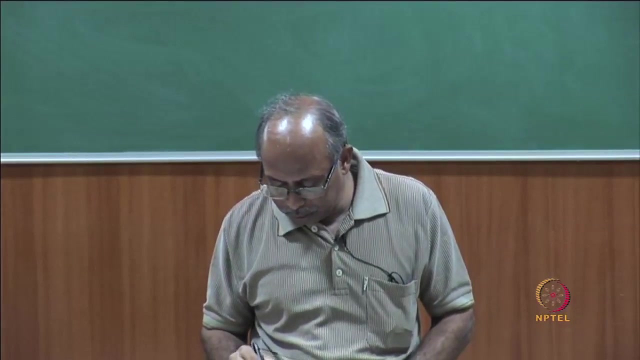 l come under cyclic load, you assume that it would. it can withstand around. that endurance limit is the you know is which, it which will be the which you can use in design. In case of concrete, you cannot do that because it will go on reducing. So what we do is: 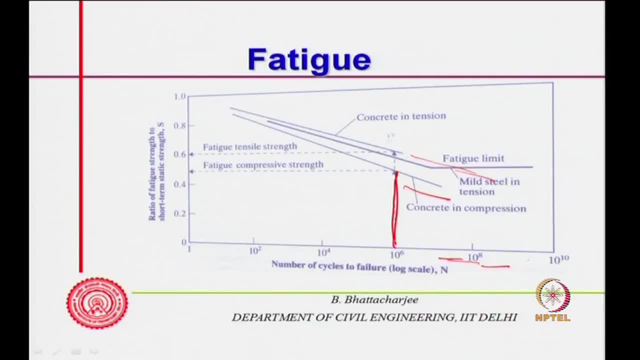 we take the fatigue strength corresponding to 10 to the power 6 cycles as the fatigue compressive strength. Similarly, in this case 10 to the power 6 tensile fatigue tensile strength. So fatigue compressive strength and tensile strength are defined with respect. 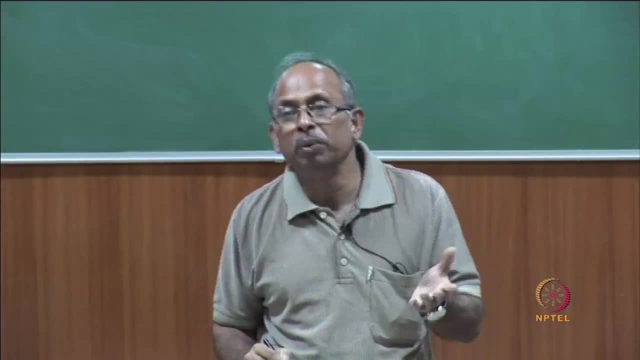 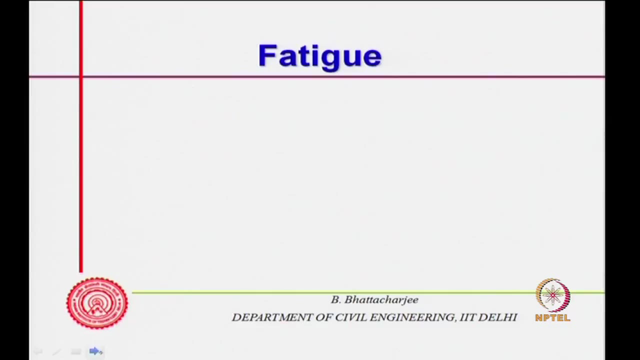 to 10, to the power: 6 cycles, because it will go on reducing. For steel, of course, you can use the endurance limit, So it will go on reducing with number of cycles, increased number of cycles. So this is how we define. 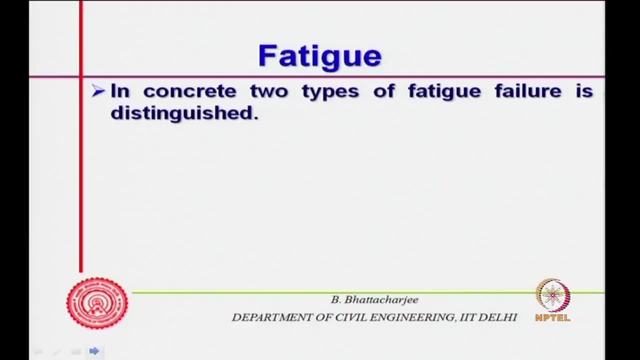 Now in concrete, two types of fatigue failure is distinguished. The one which is which is sustained load near the static strength under increasing load, causes failure. So it is static fatigue or creep rupture. Now concrete shows creep at ordinary temperature. 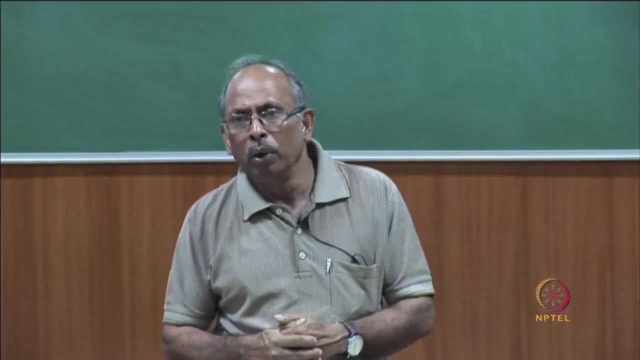 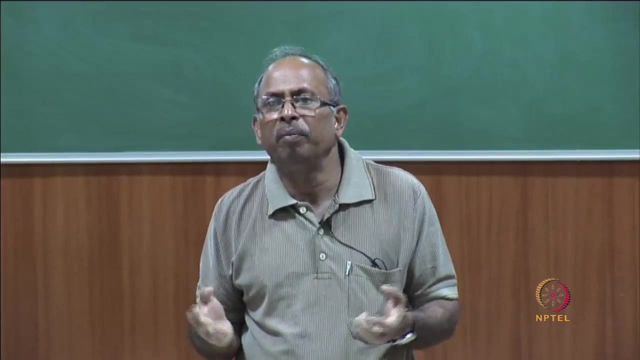 That means if you put a load- we will discuss this in subsequent module- That means if you keep the load constant and over the time period, over the period of time, you will find the deformation is increasing and it can have a failure. also depending upon the 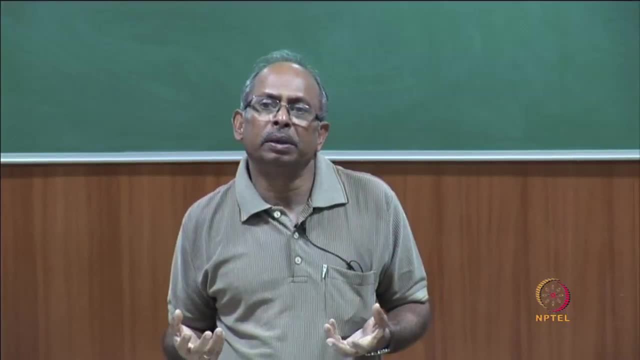 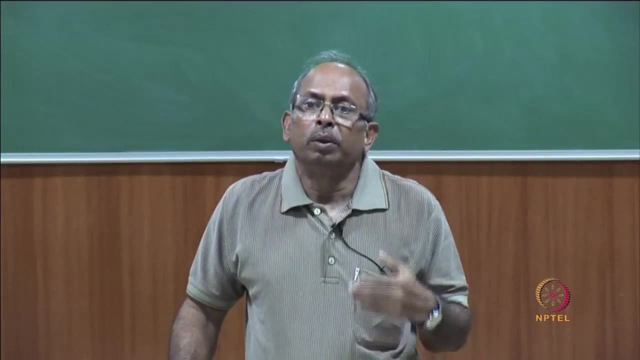 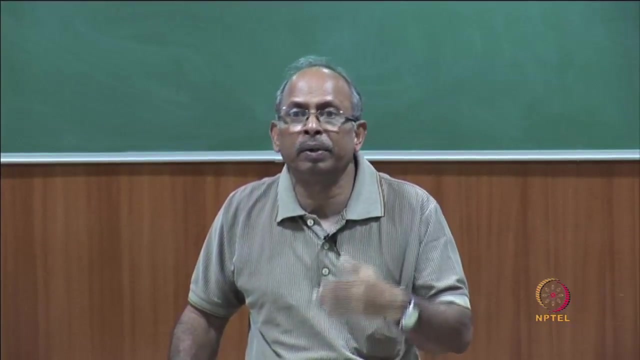 situation. So under sustained load, concrete exhibits kind of deformation and that is related to phenomena of creep. So if you have sustained load near the static strength, Now fatigue is also nearly sustained because you are reversing the stresses- and near the static. 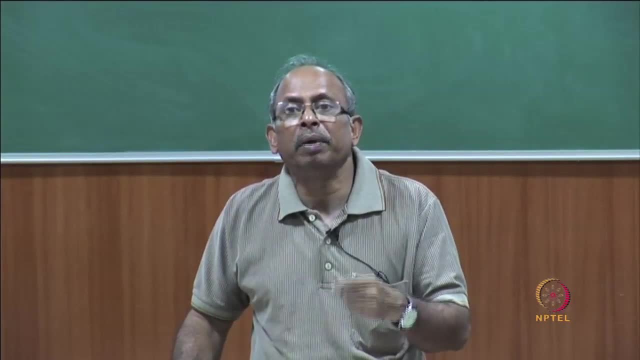 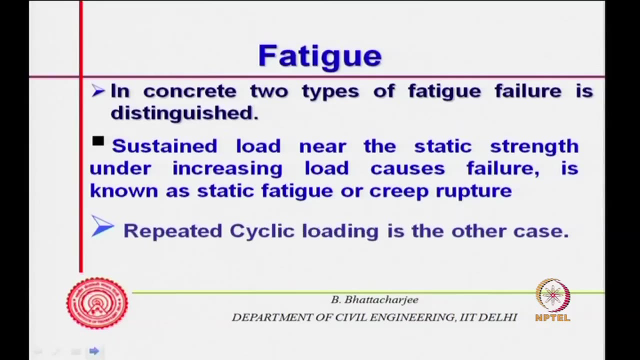 strength, So you increase the load and it causes the failure and this is related to static fatigue or creep rupture, you know. So if you are reversing the stresses, keeping keeping the stresses close to the static strength, then there can failure can be by: 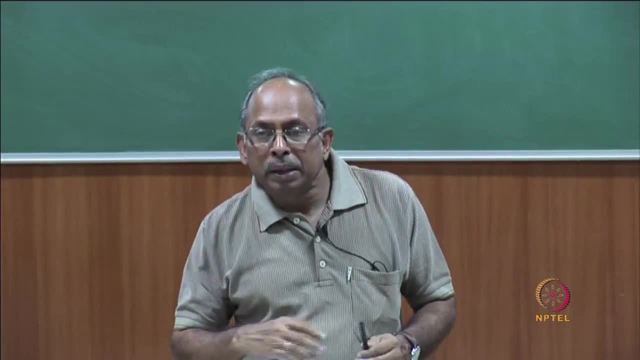 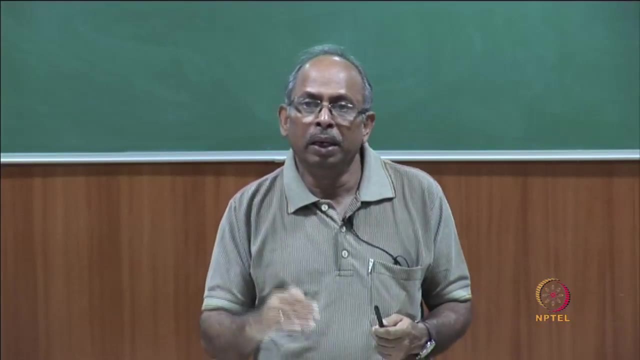 creep rupture because sustained load is sustained. very static load is sustained plus minus something is always occurring. you know, plus minus something is occurring. So this, this sustained load, can result in creep rupture. because load is sustained very close to the 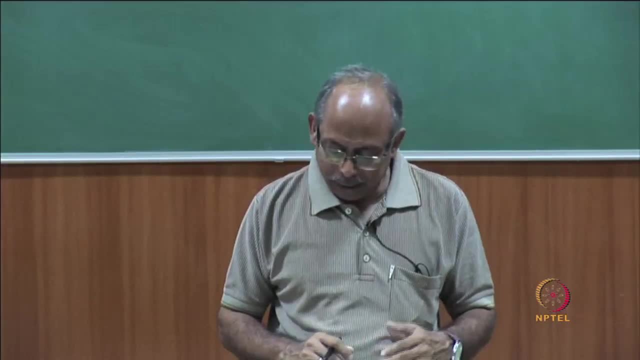 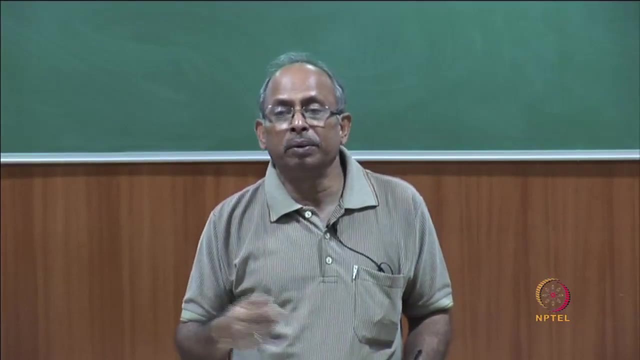 static strength. Repeated siting loading is of course other case where you are operating at much lower level, But then it fails because repeatedly you have done, you know, reversal of stresses are being done over a large number of cycles. 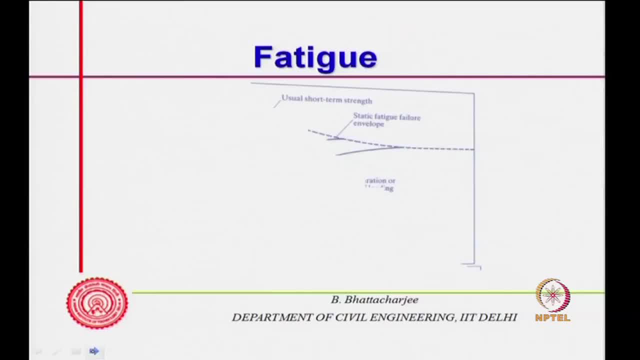 So these are the two situations and we can see the behavior in this manner If you look at this diagram, if you look at this diagram, usually you know in this case what you are doing. You are sustaining the load for 50 days, 3 minutes, stress strain, rapid loading. 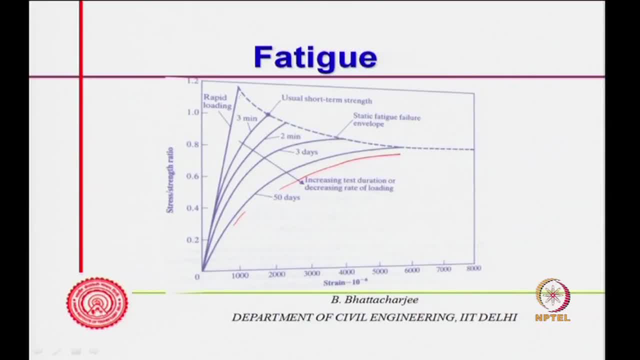 stress strain curve is like this: This excess is strain, this is stress. Rapid loading stress strain curve is like this: and here it might fail. If you finish it within 3 minutes, it will show you failure. like this: I do not have a…. Here I am only controlling the. 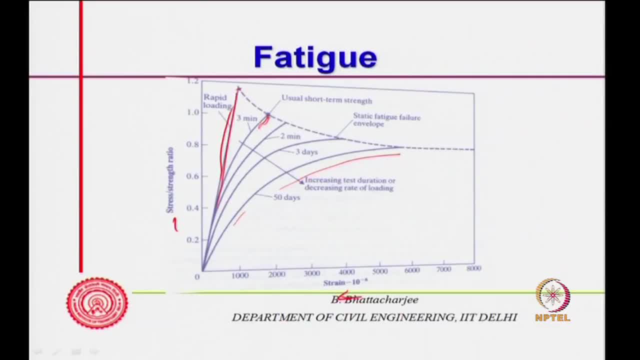 rate of loading in terms of load per, you know, per unit time, not in terms of strain control situation. So what will happen? Very rapid load loading? no… The micro cracks would not happen. It will form, but suddenly there will be a sudden brittle failure at some higher load. 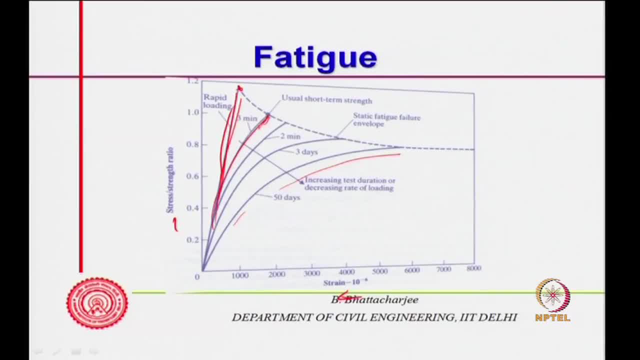 So it fails somewhere there. but if you are loading under, let us say, 3 minute failure up to failure, which could be the case in case of static, monotonic loading, So it will fail somewhere there. No, not much deformation or such thing. It will not show. It will show. 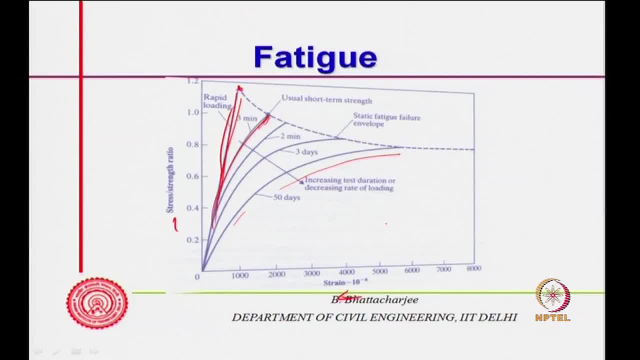 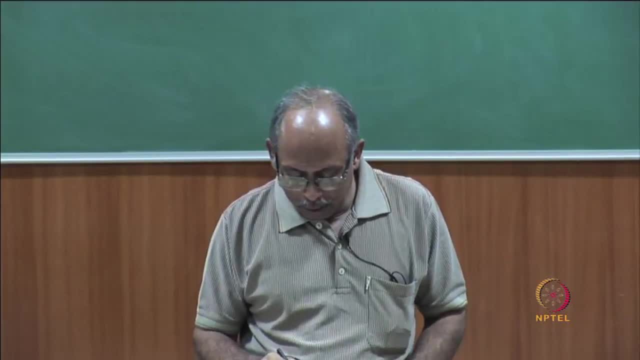 this if you have a strain control situation, So a kind of what we call strain softening would occur. you know, as the strain increases, Strength it can… Load it can carry is lower. So if you, if you, you know, if you go on, 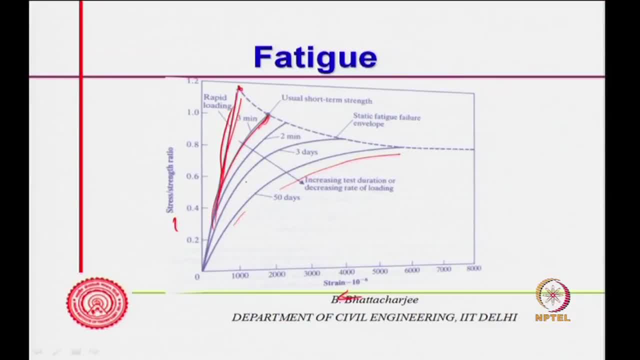 increasing…. This is normal, normal stress-strain diagram. but if it is 3 days, this is, this is, this is you know, this is about 3 days you take. If you 3 days, if you take, then 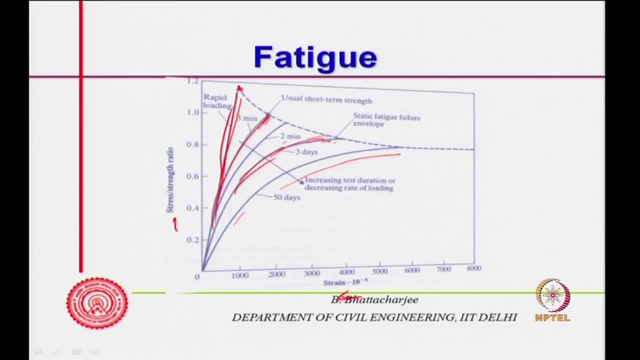 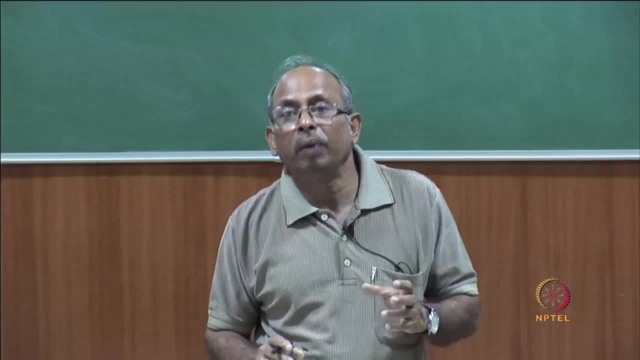 you find that…. Keep the load for 3 days, So it is 80 percent of the static load. it will actually… 80 percent of the static load, it will fail. Keep the load for 3 days, It might fail somewhere. 80 percent, I mean. this is a notional thing. One cannot take. 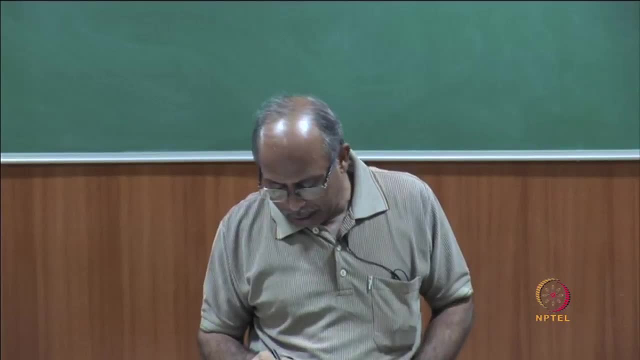 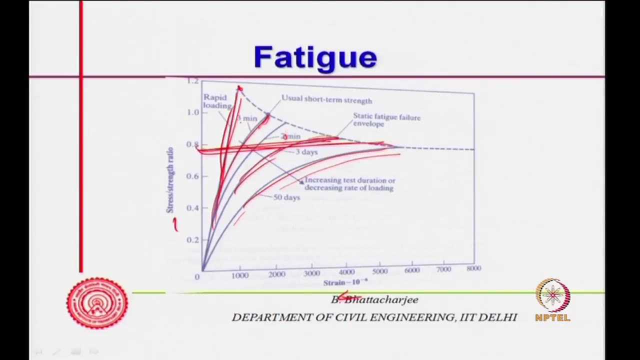 it for all the time granted, The values might differ from test to test, And if you keep it for 50 days, it is actually fail at somewhere there. So depending upon, let us say, 20 minutes, 3 minutes, 2 days, 3 days and 50 days, So increasing the test duration then, which means 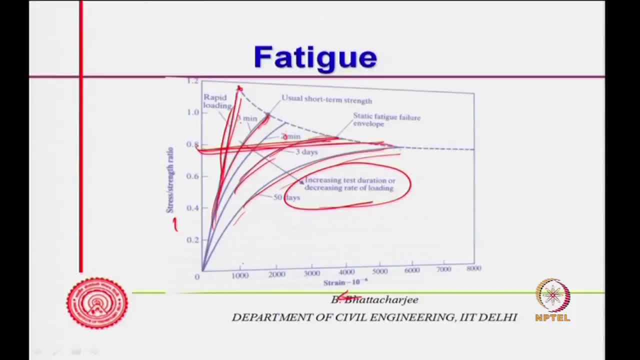 that my rate of loading. I am decreasing rate of loading I am decreasing, And at least lower rate of load loading. we have seen that it fails earlier. So 50 days, same load you are applying. in 50 days you find that the load carrying capacity is much less So. 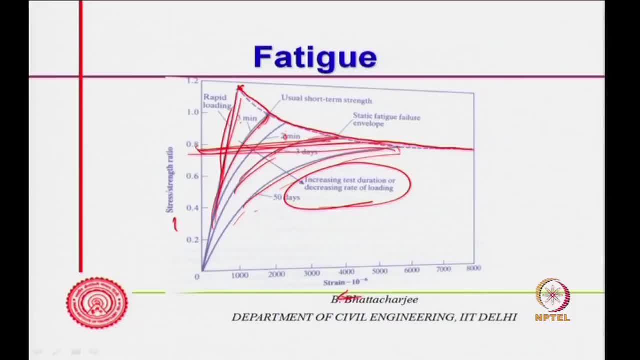 I can actually have a kind of a envelope, So you can call it static fatigue failure envelope. static fatigue failure envelope because this is related to micro-cracking or creep behavior and so on. So very close to the load quickly. if you load it, it fails. 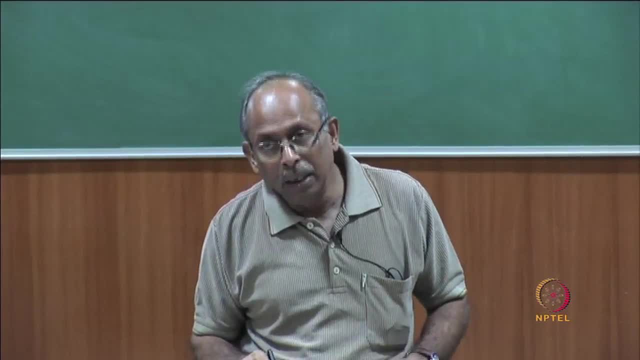 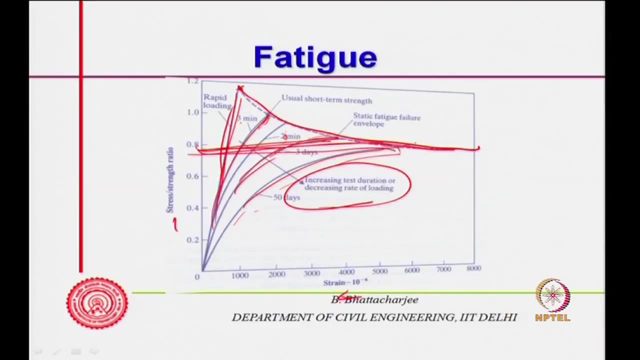 at higher load. If you take it for longer period of time, it will actually fail after certain period of time because it is sustained for 50 days, So it will actually fail. So this is related to static fatigue failure. So close to this one if you take, you know, if you do reversal. 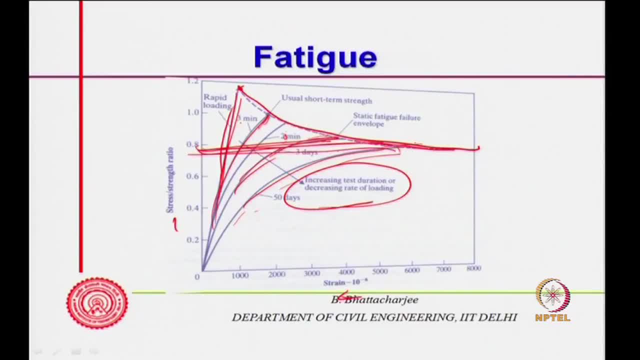 for 50 days, it will fail. So if you do reversal somewhere here, if you do lot of reversal, the time frame it will be related to this. Actually, failure would occur even though you have not gone to too much of a cycle, For example for 0 cycle. this situation is: 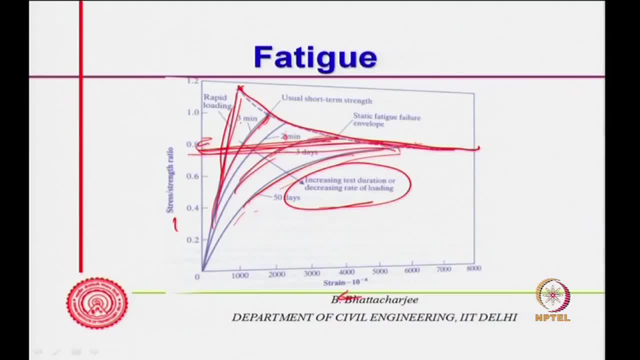 for 0 cycle. So even if you have not got too much of cycle, it will still fail. So this is actually related to static failure, static fatigue failure, you know So, or creep rupture, as we are calling it. creep rupture, right, And this is again strain versus stress. 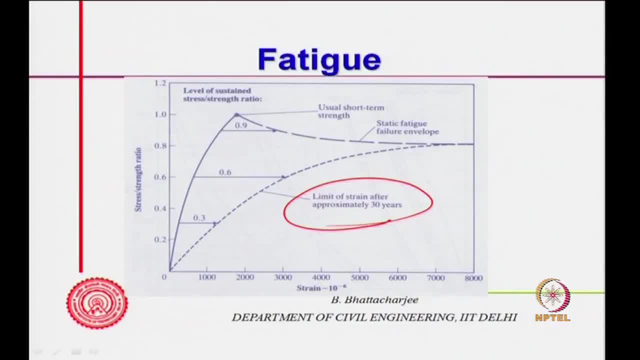 curve. So limit of strain after approximately 30 years. So if I look at it, static rupture curve is here Maximum strain after 30 years. this envelope gives you 50 days we looked into. So 0.6 of the strength, 60 percent of the strength if you load it to after 30. 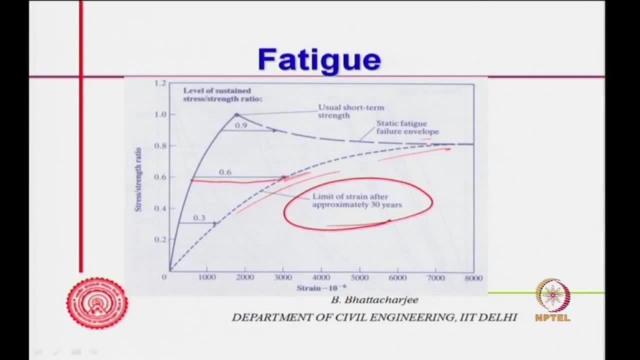 years, deformation will be somewhere here. you know, after 30 years deformation will be somewhere here. Of course it will not fail, but if you put it at 80 percent after 30 years it will actually fail. after 30 years actually it will fail. So this is it. 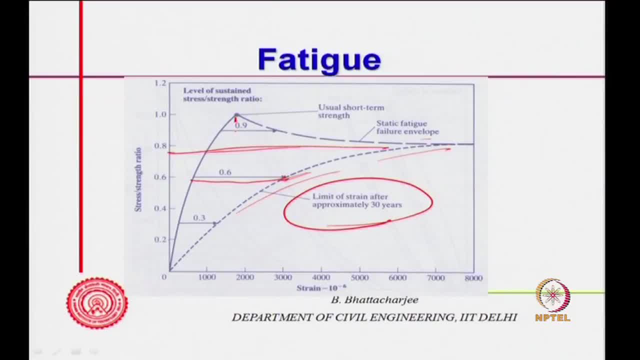 And this is the usual short term strength, which is about 3 minutes or so. So this is the 0.3,, let us say, 30 percent of the strength it will actually, after 30 years, deformation will increase, but it will still not fail. So it fails up to something like 80 percent. 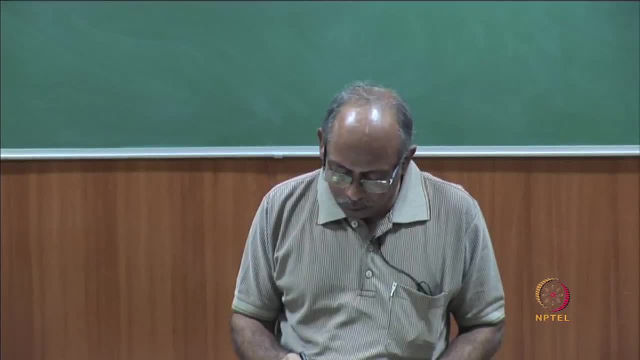 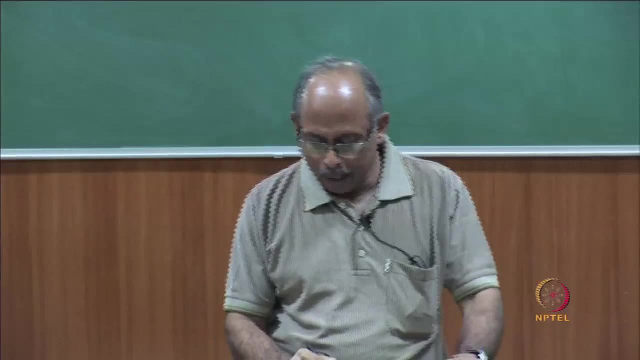 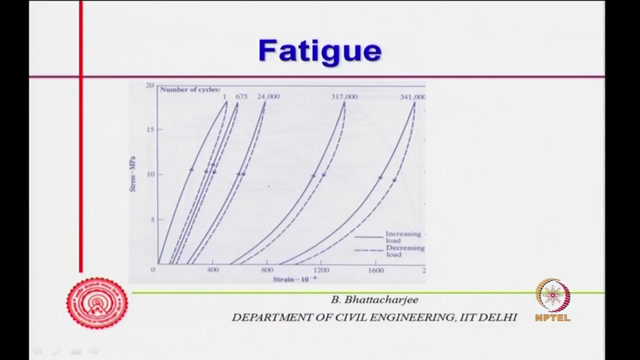 of the static strength over 30,, after 30 years and so. But if you have something more than that, it will fail. So this is how you know. this is related to this fatigue, And if you do reversal of stresses, one cycle, the behavior is like this: 3000 and first. so that this. 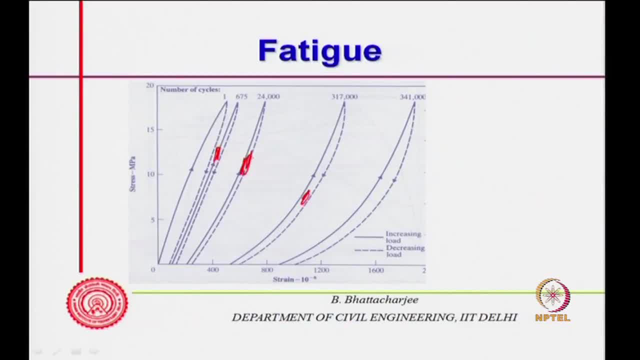 hysteresis area reduces significantly. hysteresis area reduces significantly and then this area would increase. So what we will do is, you know the fatigue we have. introduction to fatigue I have given to you right now and you can see that after long period of 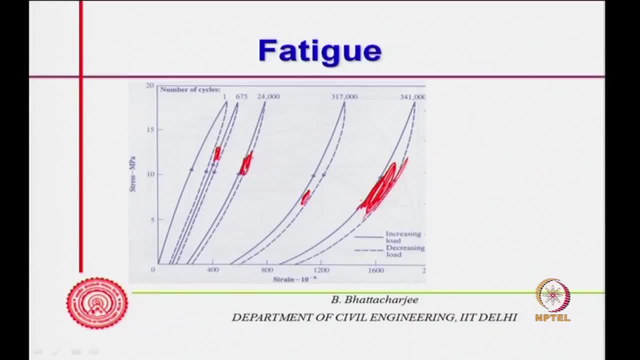 time because of the- because after long cycling number of number. of you know cycling causes more micro cracks to appear. So therefore this increases. In the beginning there is a reduction, but under long cycling actually more micro cracks form under fatigue loading because there will be frictional and heat generation. 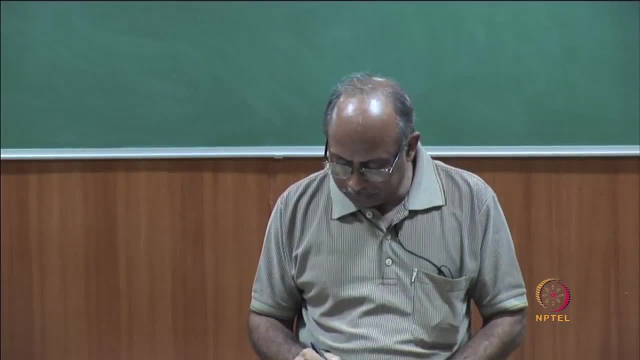 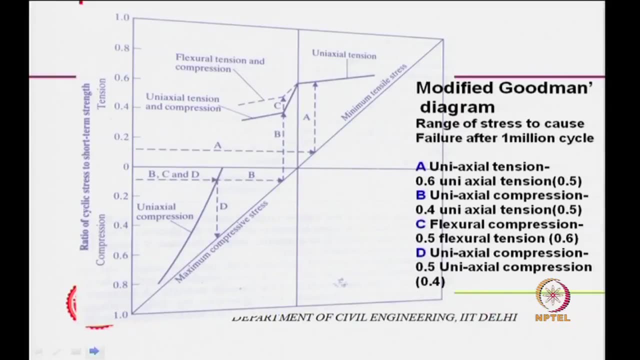 as it happens, or whatever mechanisms are there. So fatigue causes failure in this manner. We have something called modified Goodman's diagram Here. this diagram helps us in finding out what is the stress level or reversal of stress concrete can withstand. For example, 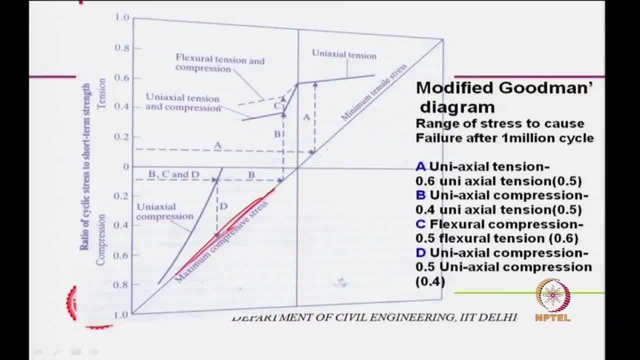 this curve. you know this is a minimum compressive stress. This is a stress line, This is a minimum tensile stress line. Now, in uniaxial compression, if you are operating at 40 percent of the strength level, or let us say 20 percent, 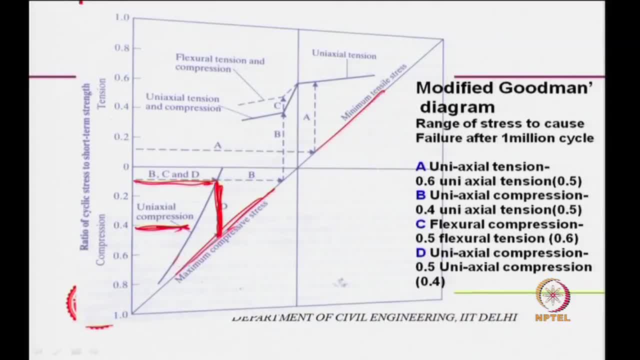 10 percent of the stress level. you can do reversal up to this and come back in compression mode only. So failure would occur at 10 to the power 6 cycles. and if you are applying, let us say, tensile stresses, you can go up to 20 percent of the tensile, 30 percent of. 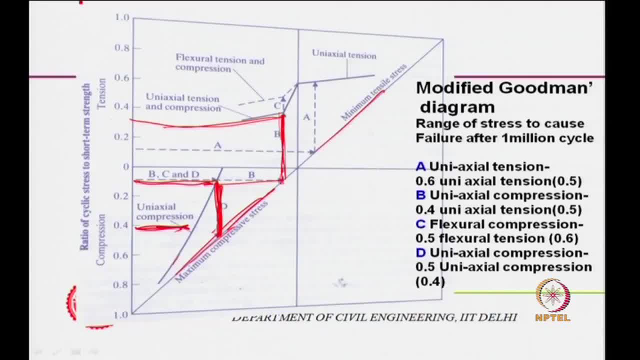 the tensile strength, and reversal can occur from 10 percent of the compression to 30 percent the tensile. This is in compression, uniaxial tension and compression, This is in flexure. And if you are doing purely tensile, say at 10 percent of the tensile load, you can go. 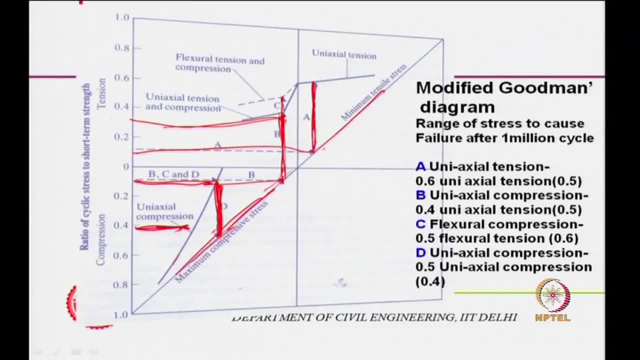 up to this and come back. So modified Goodman's diagram can be used to find out what level of stress reversal you can do, what level of stress reversal you can do at what level of static stress level. At 10 percent of the stress level you can reverse the stresses. 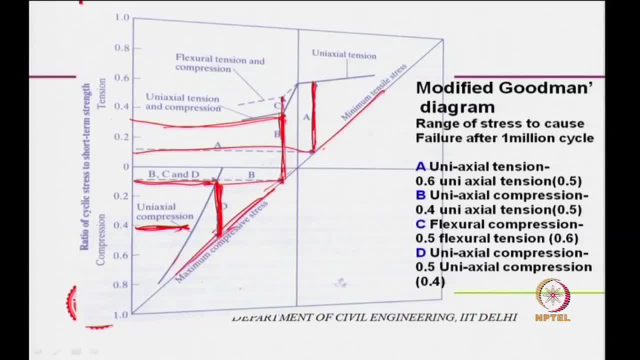 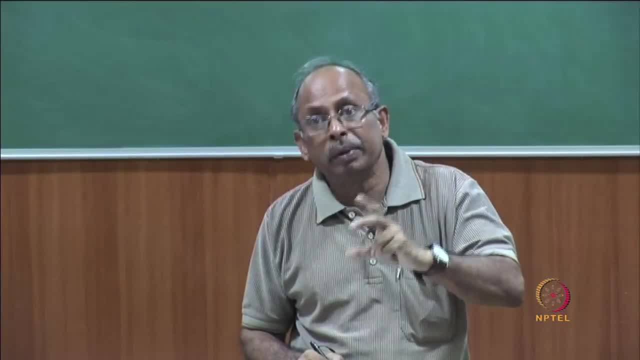 given from this diagram, Say if it is compressive stress, If it is tensile stress, one can determine from this diagram. So modified Goodman's diagram can be used to find out what level of stress, stress range of stress you can use. 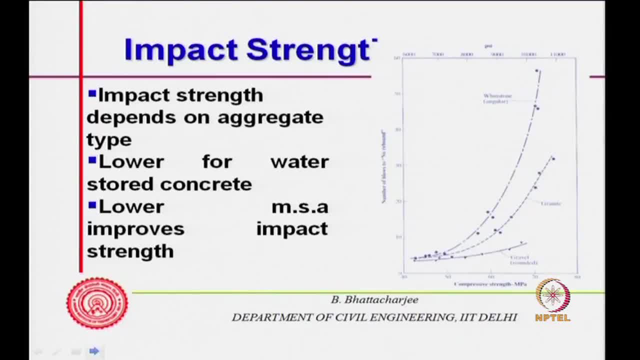 Impact strength is again can be related to compressive strength and it depends strongly upon aggregate type. Lower for lower water stored concrete and lower MSA improves impact strength And that is shown by this diagram. different types of aggregate: This is the number of 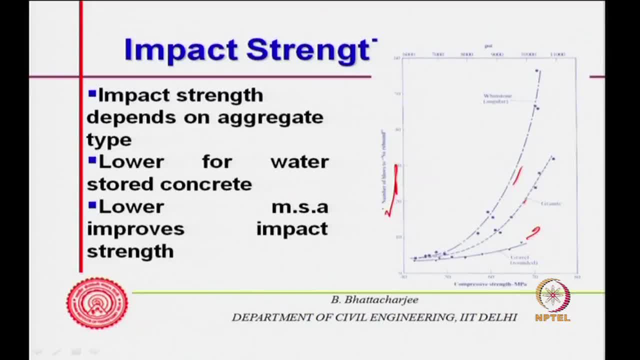 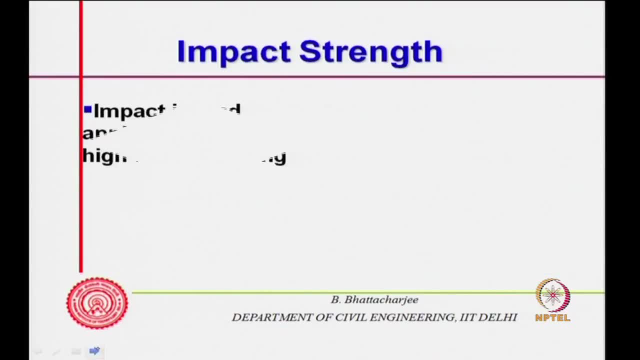 actually impacts. actually, it can take the way it is measured, depending upon compressive strength, Both impact and both impact strength, as well, as you know, abrasion. they are function of compressive strength And impact is loading at a very, at a very high load, you know. 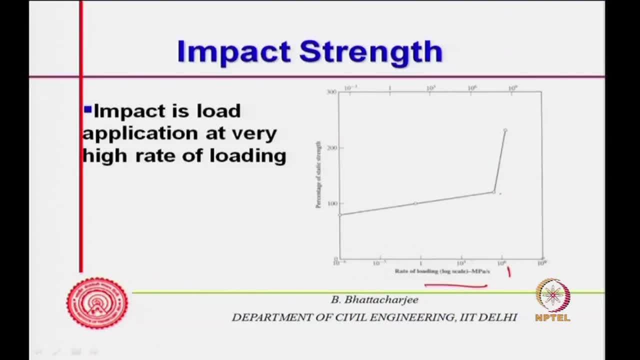 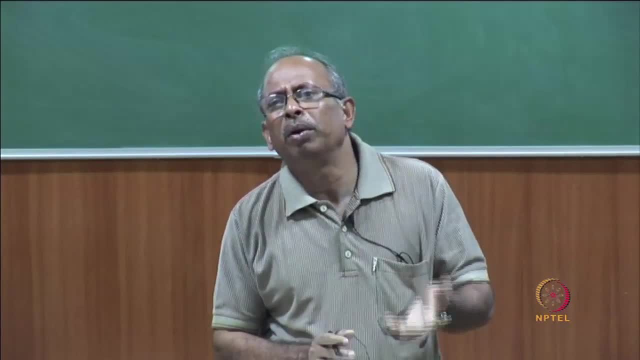 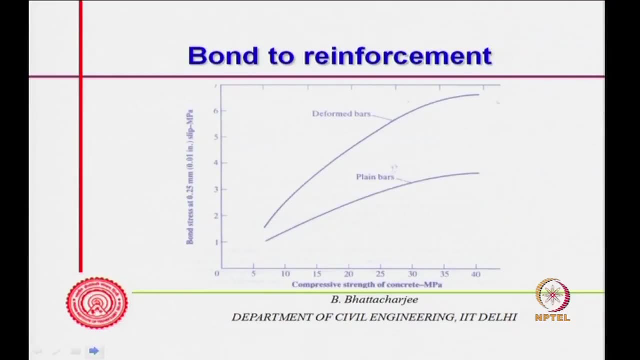 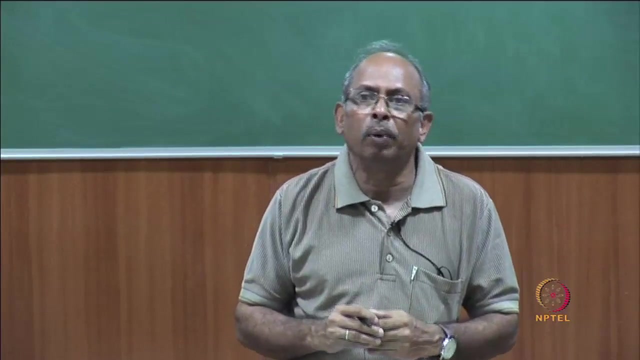